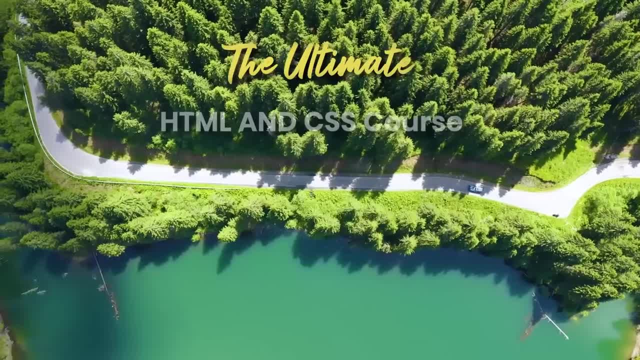 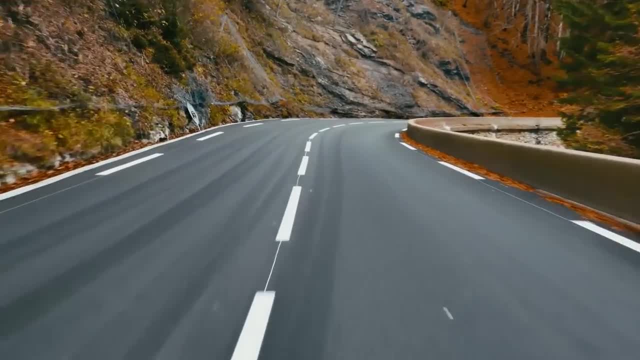 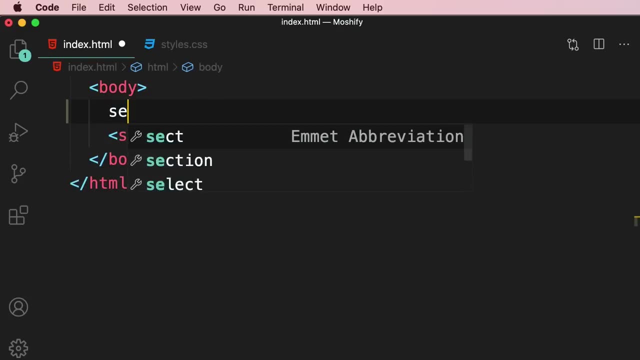 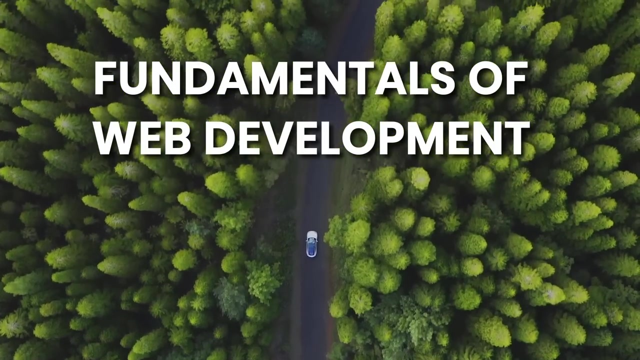 Welcome to the first part of the ultimate HTML and CSS series. In this series, I'm going to take you on a journey and teach you all the skills you need to build fast and beautiful websites that look great on all kinds of devices. I'm assuming you know nothing about HTML or CSS and want to learn everything from scratch, So in the first part of this series you're going to talk about the fundamentals of web development with HTML and CSS. In the second part, we'll explore the advanced concepts of HTML and CSS. 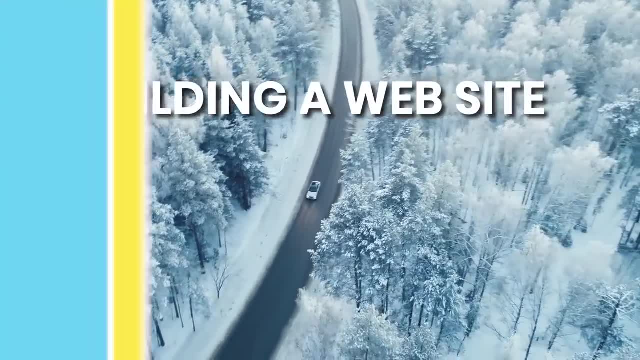 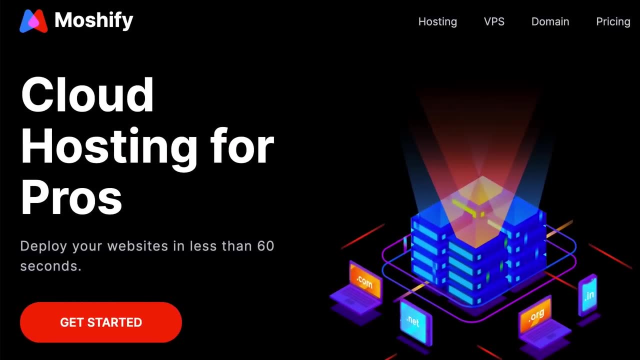 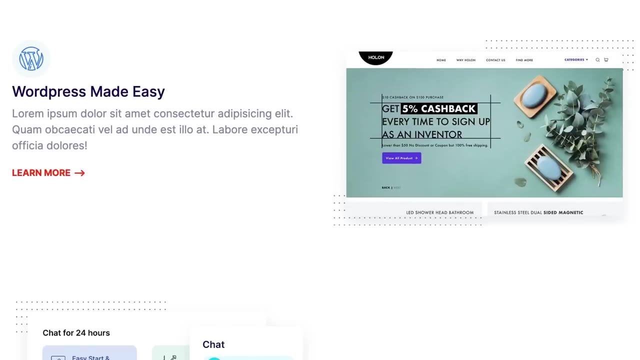 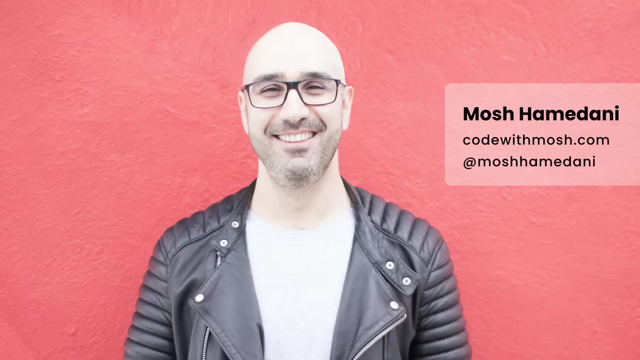 And in the third part, we'll put everything together and build a beautiful, responsive and blazingly fast website for an imaginary cloud hosting company called Moshify. If you want to play with this website, just head over to moshifycom and see it for yourself. This is what you're going to build in this series. I'm Mosh Hamadani and I've taught millions of people how to code or how to become professional software engineers through my coding school and YouTube channel. If you're new here, be sure to subscribe, as I upload new videos all the time. 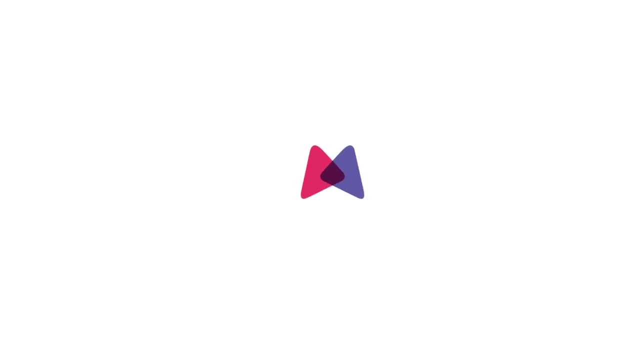 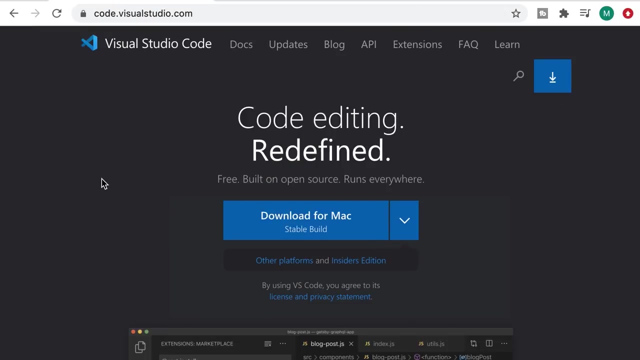 Now let's jump in and get started. All right, let's talk about the tools you need to take this course. For the starter, you need a code editor. There's so many code editors out there, like Visual Studio Code or VS Code, Sublime Text, Atom and so on, In this course. 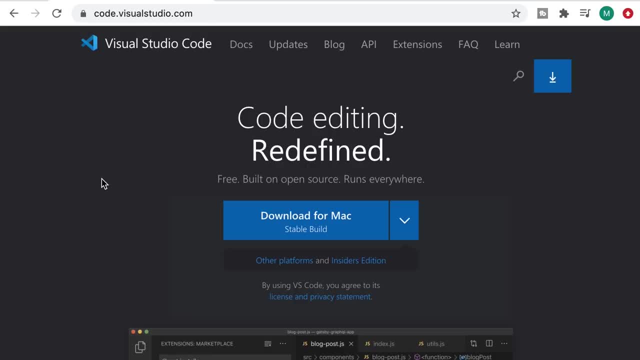 I'm going to use VS Code, along with a few extensions, for starting a web server and formatting our code. You're welcome to use your favorite code editor if you know what you're doing, but otherwise head over to codevisualstudiocom and download the latest version of VS Code. 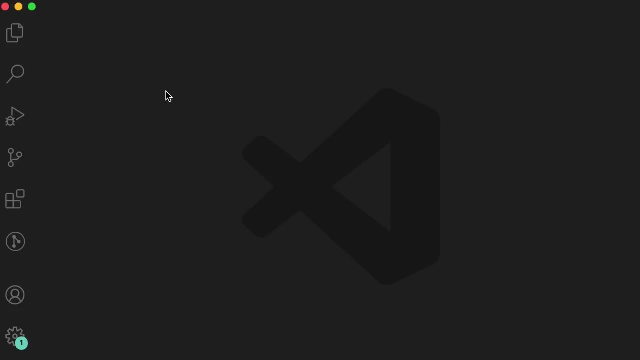 Now, here inside VS Code, we're going to install a couple of extensions. So let's open the extensions panel and search for Preview. Here's the extension we're going to install: Preview Code Formatter. With this extension, we can format our code and make. 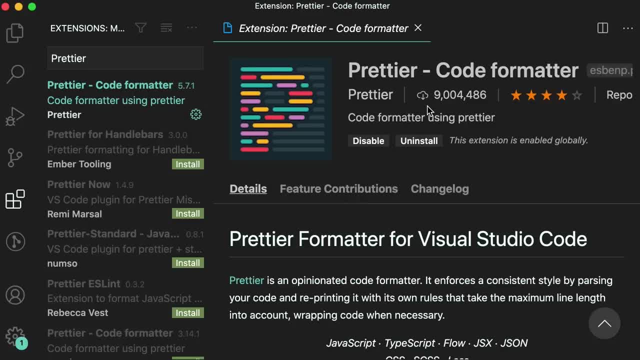 it pretty. This is a very popular extension. As you can see, it's been downloaded more than 9 million times. So over here you're going to have an install button. Just click it and you're done. Next we're going to install. 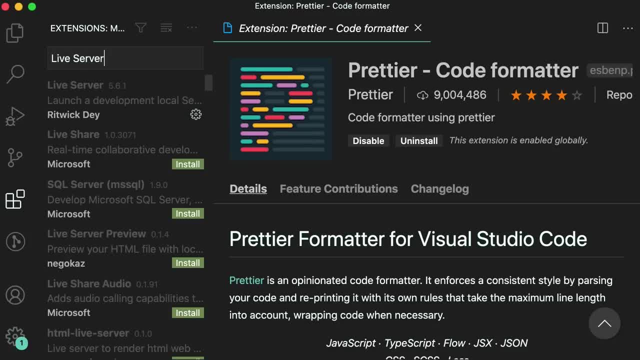 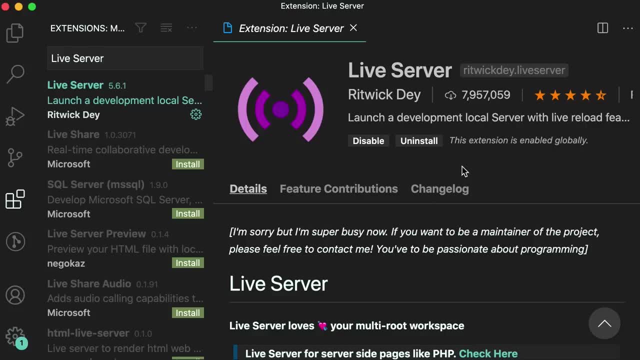 another extension called Live Server. With this, we can launch our website inside a development web server. Again, this is a very popular extension. It's been downloaded almost 8 million times. Now, in addition to these we're going to use: 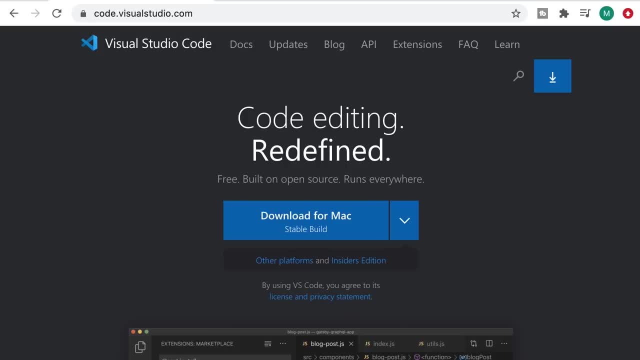 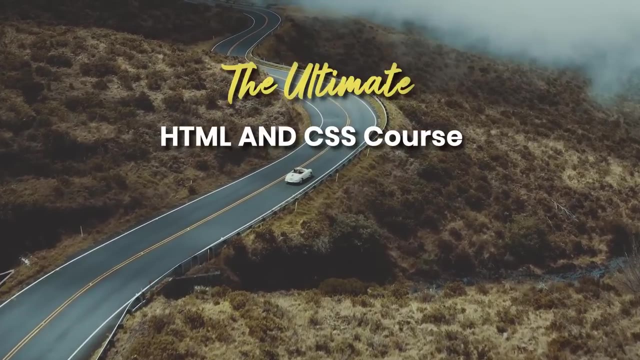 a browser to view and test our web pages. Again, you can use your favorite browser, but in this course, I'm going to use Google Chrome and I encourage you to use the same browser so you can easily follow the course. We're going to start our web development journey here. 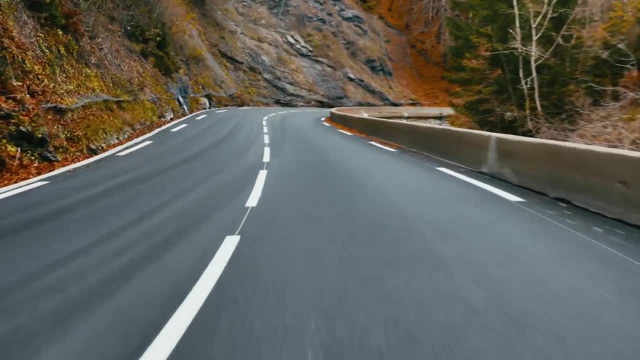 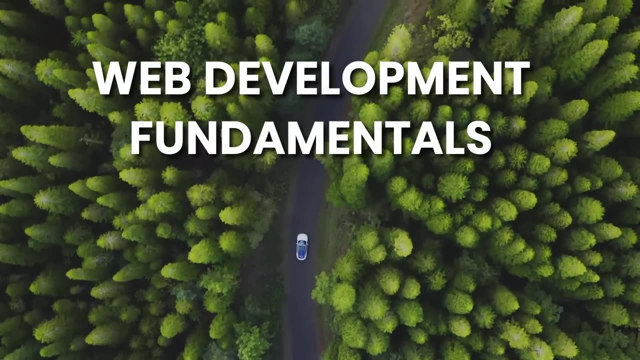 In every section you'll learn something new about web development and by the end of this course you'll put all of this together to build a beautiful web page. In this section, we're going to talk about the fundamentals of web development. 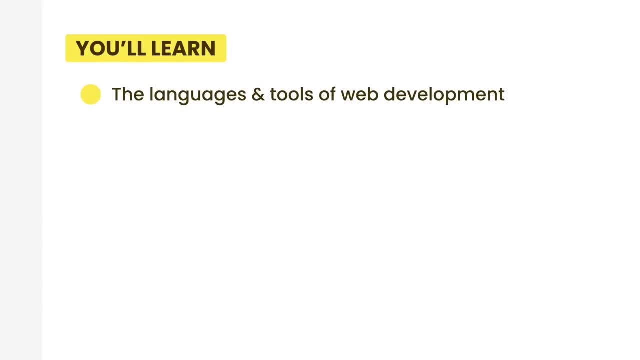 you'll learn the languages and tools used in web development, as well as the key concepts and vocabulary, such as URL, HTTP, DOM and so on. We're also going to talk about how websites work, so you will understand what exactly happens under the hood. 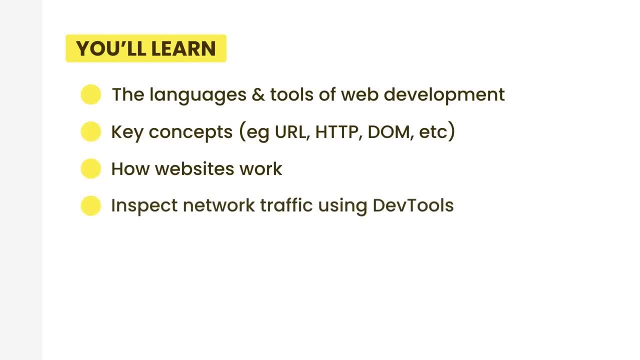 when you use your browser to visit a website. You will also learn how to inspect network traffic using Chrome DevTools, which is a very powerful tool used by front-end developers. We'll also talk about the basics of HTML and CSS and validating web pages, which is 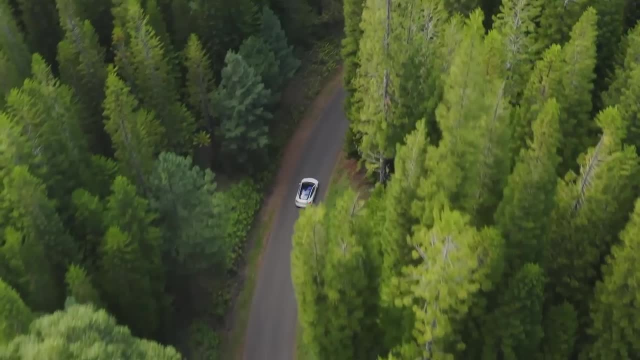 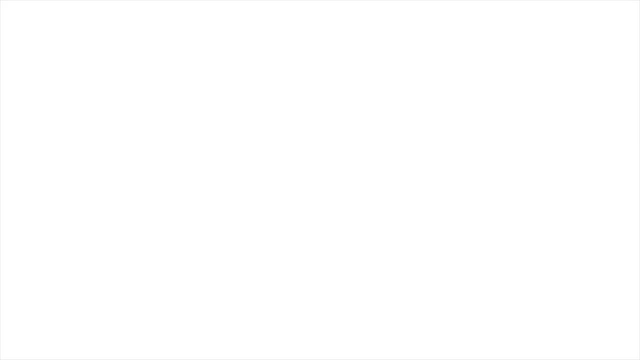 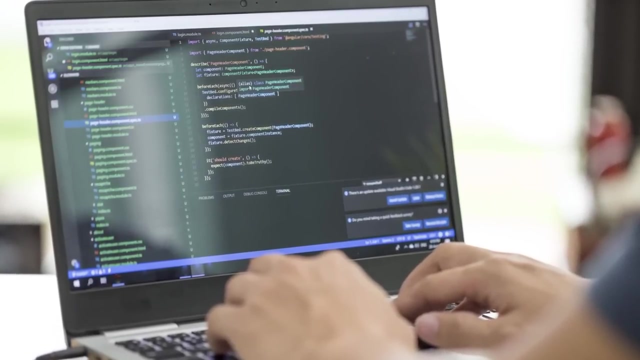 something a lot of developers miss. This is going to be an awesome journey, so let's jump in and get started. This course is your first step towards becoming a web developer, So let me give you a simple roadmap to know where you are and where you should go next. 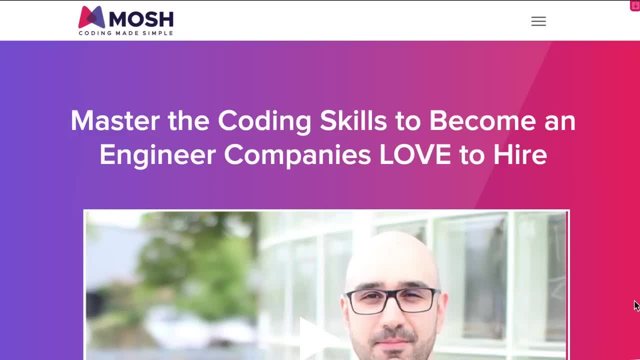 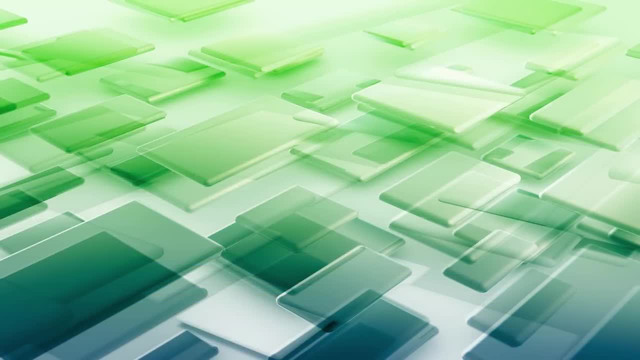 Every website has two parts: a front-end and a back-end. The front-end is the part where you can see in your browser and interact with all the visual aspects. The back-end is the part that powers the front-end. It's behind the scenes and it's mainly about 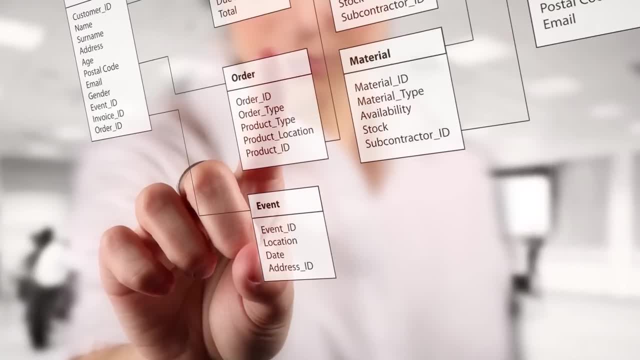 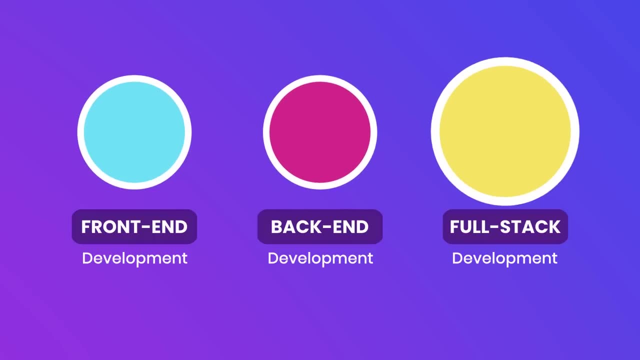 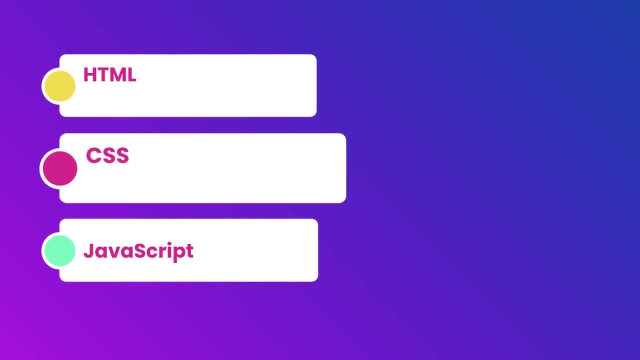 storing data in databases and providing it to the front-end. So web development jobs fall into three main categories: Front-end development, back-end development and full-stack development, which involves both front-end and back-end development. Front-end developers use HTML, CSS and. 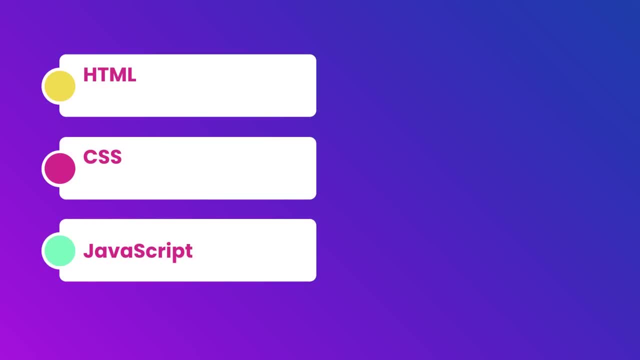 JavaScript to build front-ends. Back-end developers use HTML, CSS and JavaScript to build front-ends. Back-end developers use HTML, CSS and JavaScript to build front-ends. Back-end developers have different sets of tools available to them, which is outside. 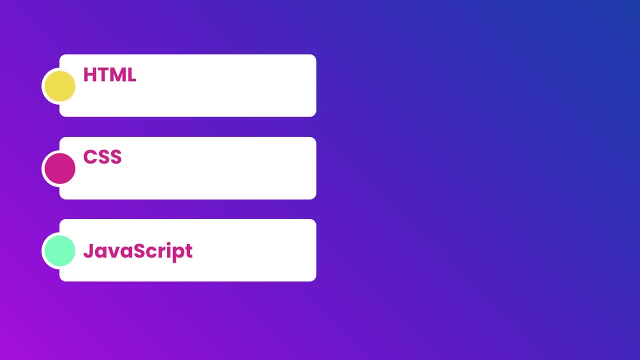 the scope of this course, So let's talk about HTML, CSS and JavaScript. HTML is short for Hypertext Markup Language. I know it's a mouthful, but basically we use HTML to define the building blocks of our webpages. CSS is short for 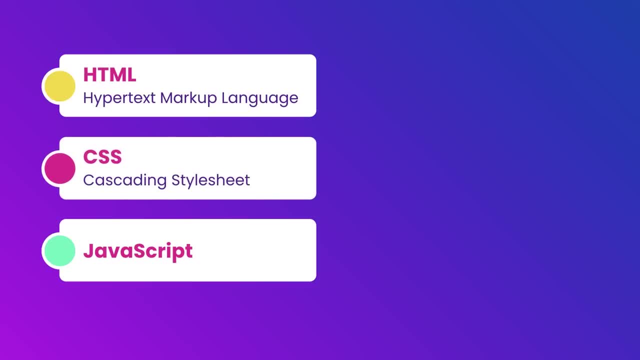 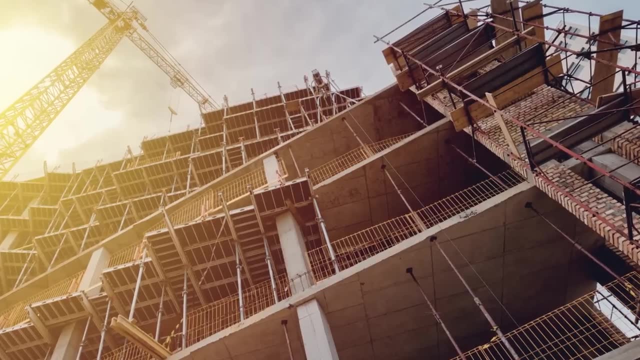 Cascading Style Sheet and is used for styling webpages and making them beautiful. JavaScript is used for adding functionality to webpages. Let me give you an analogy. Think of a building. A building in the real world is like a webpage on the internet. 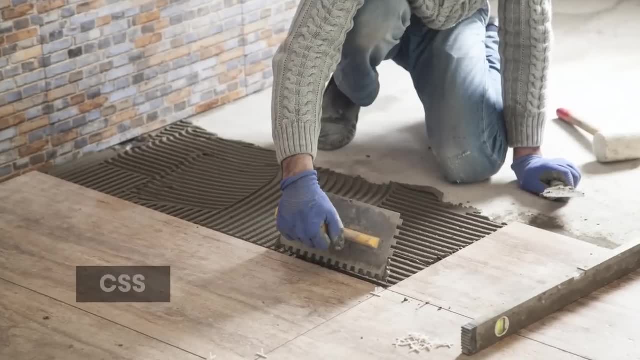 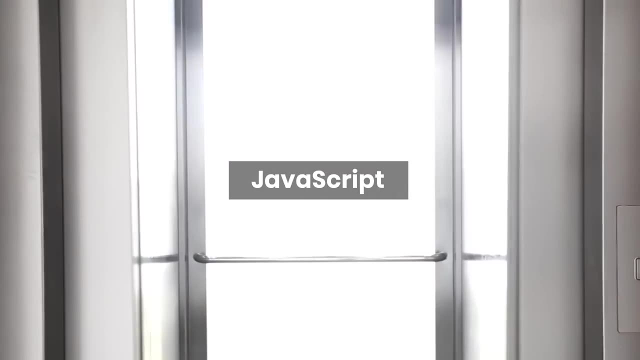 It has a skeleton or structure. it can have pretty walls, windows and tiles and it can have certain functionality. For example, when we press the elevator button it comes to pick us up. Here's a real example. Let's say we want to build. 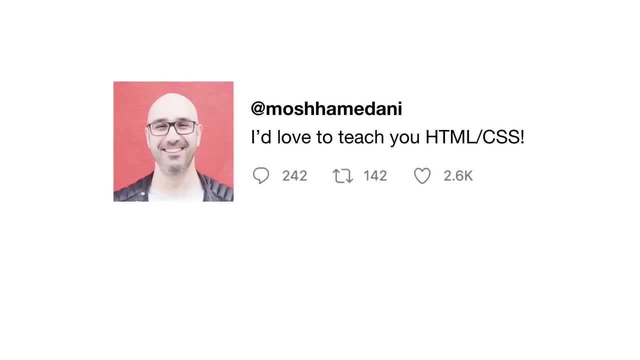 a website like Twitter. For each tweet, we want to have a layout like this. So first we use HTML to define all the building blocks of this layout. What are these building blocks here? An image, some text indicating the user's Twitter handle, another block of: 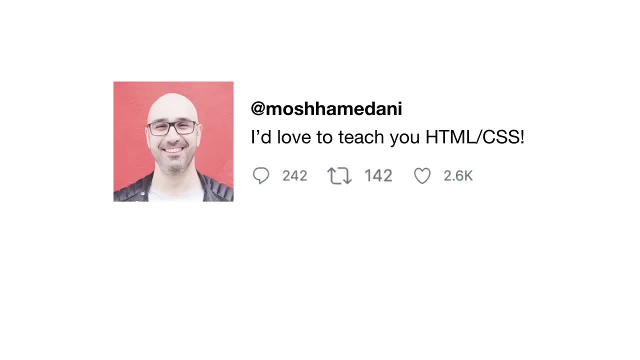 text containing the message and three icons for commenting, retweeting and liking the tweet. We use HTML to add these building blocks to our webpage. Then we use CSS to give it visual effects. For example, with CSS we can make the font bold. 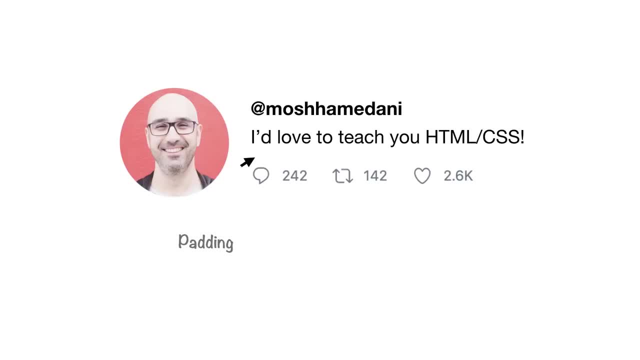 we can make our image round. we can add some padding around here. we can change the color of these icons and define their look when we hover over them. So CSS is all about aesthetics or visual effects. With CSS we can also create beautiful animations. 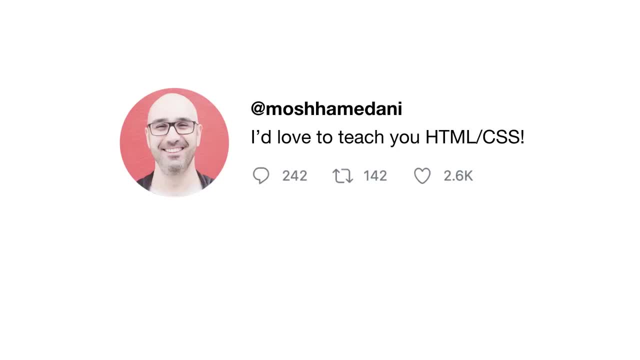 Now, most webpages these days are interactive. They respond to our actions, like clicks and scrolls. This is where JavaScript comes in. With JavaScript, we can add functionality or behavior to our webpages. For example, we can like a tweet, So JavaScript is a. 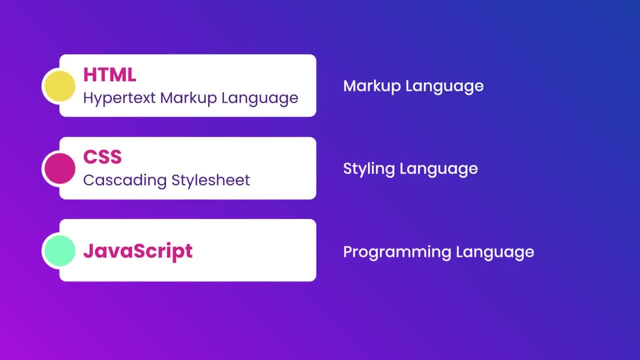 programming language, while HTML and CSS are not Meaning. we cannot use them to tell computers what to do. We use them to define the building blocks of our webpages and style them. Every webpage we have seen on the internet is built with these three. 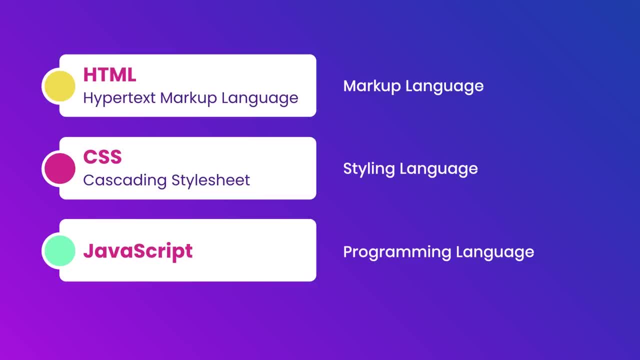 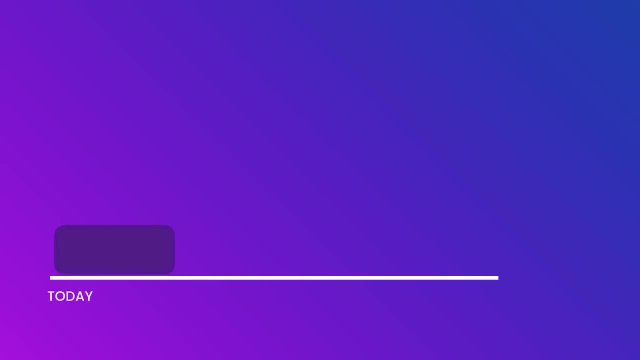 languages. So the better you learn and understand these languages and their features, the better you will be at front-end development. So your front-end development journey starts with HTML and CSS. I would say if you spend three to five hours every day studying and coding, you should be able to. 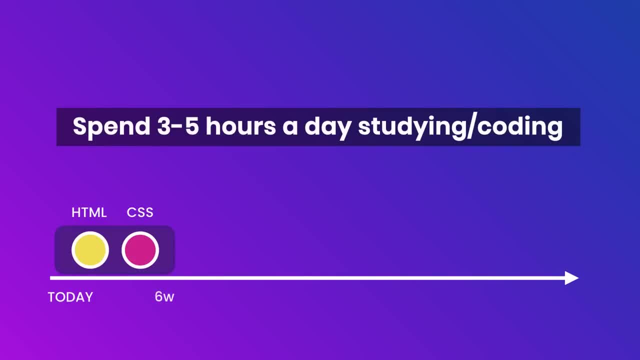 have a reasonable understanding of these two languages in about a month or a month and a half. Once you learn these languages, then you need to learn JavaScript. I have a separate series for learning JavaScript, So after finishing this series, you may want to enroll in that series. 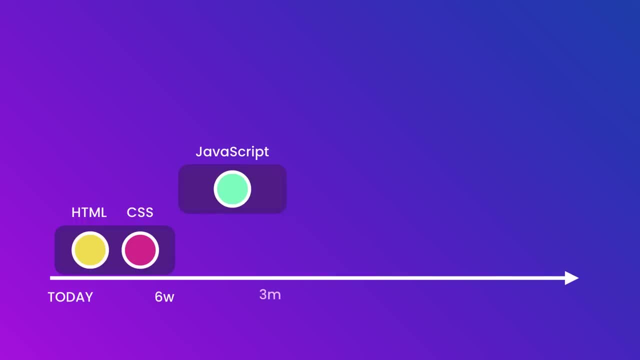 I would say learning JavaScript would probably take another six weeks of your time. Of course, you're not going to be a JavaScript expert in just six weeks, but you will have a reasonable understanding of it and you will learn more as you work on different projects. 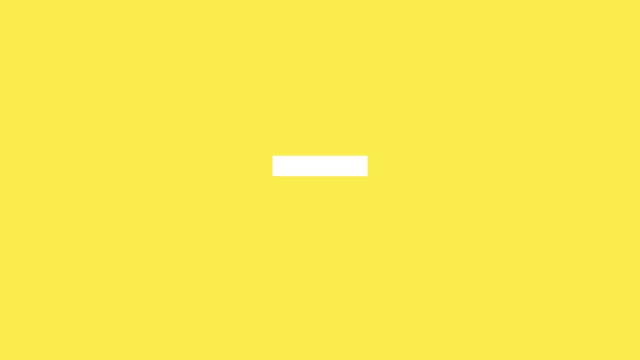 So the first three months is all about the fundamentals. Now, the first three months is a pretty big step for you. Building websites often includes a bunch of repetitive tasks. This is where front-end frameworks and libraries come in. A framework or a library comes with a lot of code that. 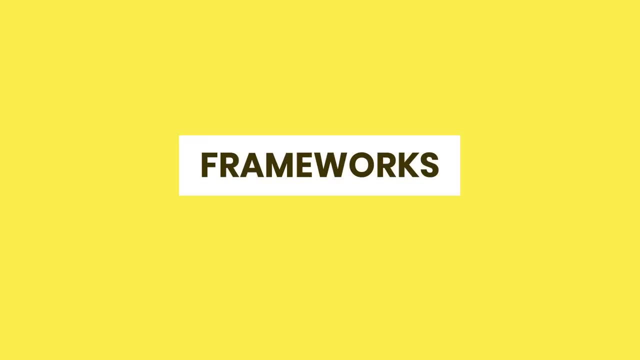 we can reuse in our websites, So they help us get the job done faster. That's why a lot of companies these days use one of these popular frameworks like React, Angular or Vue. Now, technically, React is not a framework, is a library. 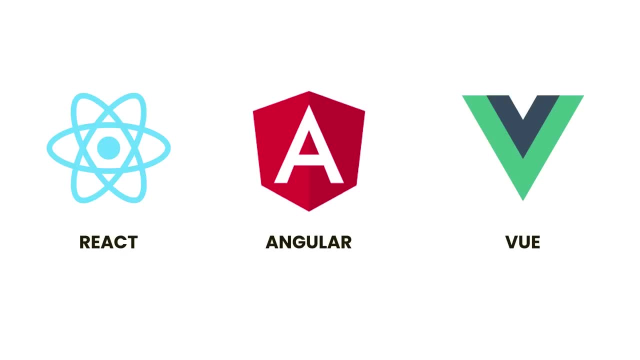 But, subtle distinction aside, all these tools serve the same purpose. They help us do it and they help help us build applications faster. Now you don't need to learn all of these to get started. Different companies use different tools for different projects. 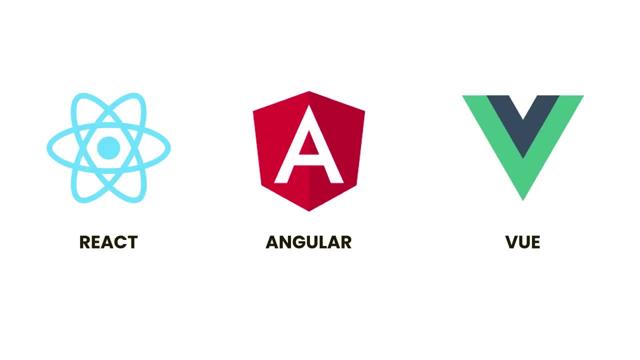 So as you move from one project to another, you may want to learn about the other tools. If you're starting out, just focus on React, because it's the most popular tool in this space. Once you learn React, you can always learn the other tools if needed. For React you would probably need. 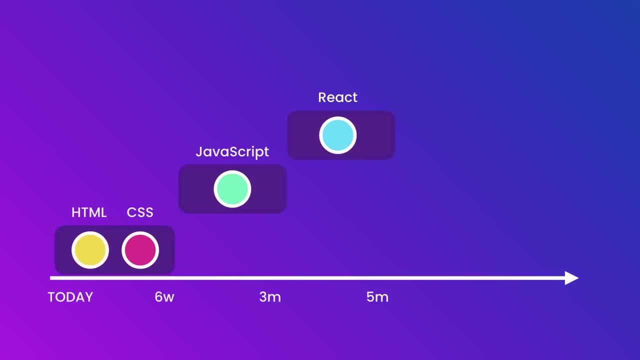 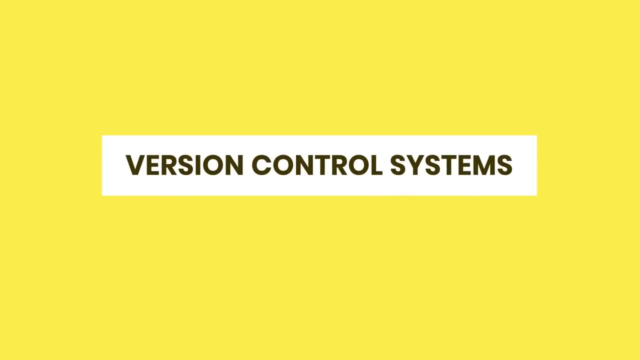 1-2 months Again, I have a comprehensive course on React. more than 40,000 people have taken this course and loved it Alright. what's the next step? Version control systems. We use a version control system to keep track of our project history and work. 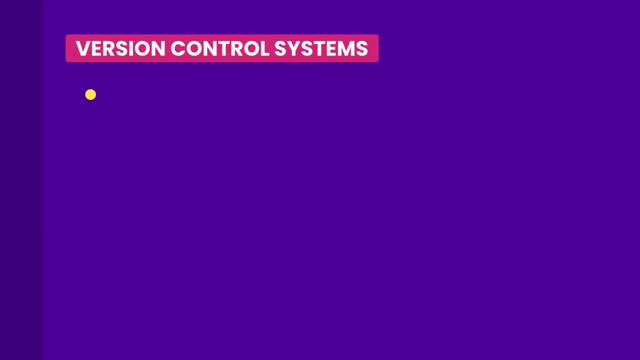 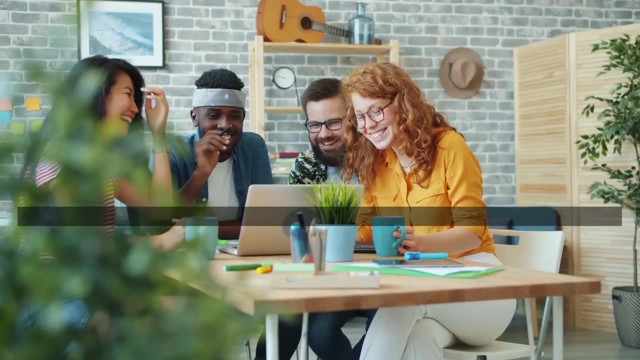 collaboratively with others. There are many version control systems out there, like Git, Subversion, Mercurial and so on, But Git is the most popular tool in this space and is used in more than 70% of software companies. That's why you'll see it in almost every job. 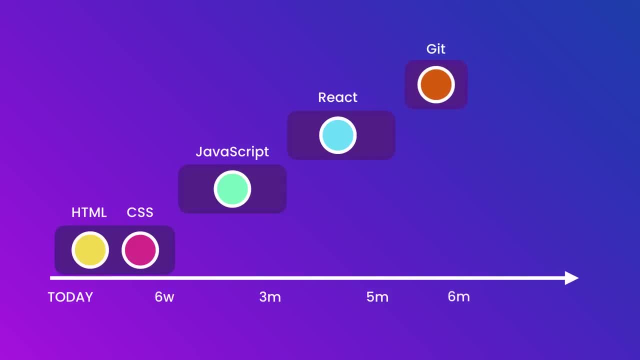 description. I would say you would probably want to learn about React, because it's the most popular tool in this space, and you'll probably need 2 weeks for learning Git And again, I have a comprehensive course for you. So these are the essential skills that every front-end. 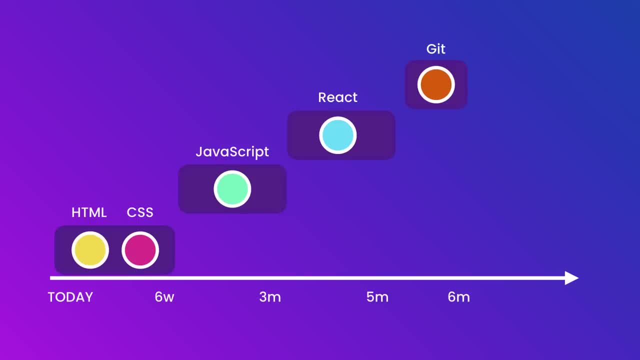 developer must have. You'll see these listed on almost every job description. Now, different jobs require other skills, but these skills vary from one company to another, So you can learn these additional things in the future or on the job. For now, just focus on these. 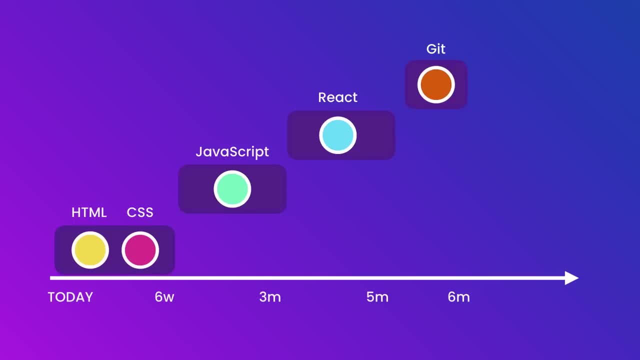 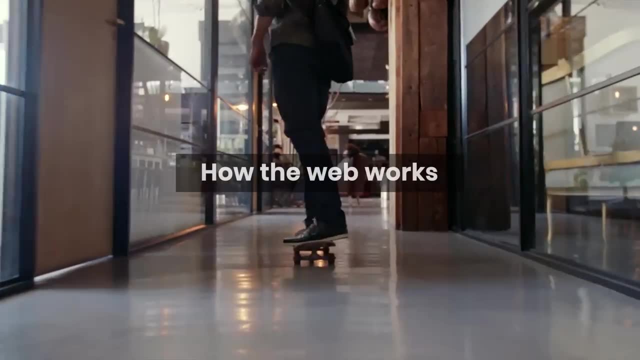 4 skills or 4 steps. Remember: less is more. Don't try to learn too many things quickly. You won't learn anything, You'll just waste your time. Alright, that's your road map. Next, we're going to talk about how the web works. 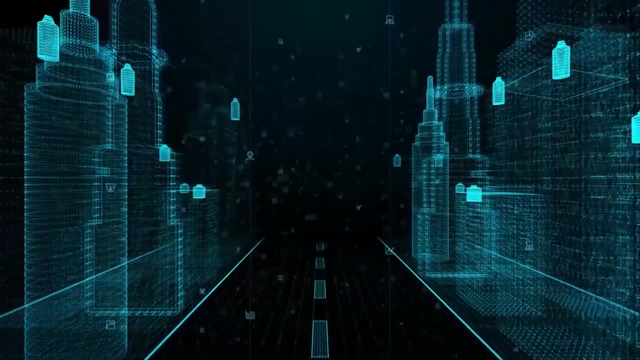 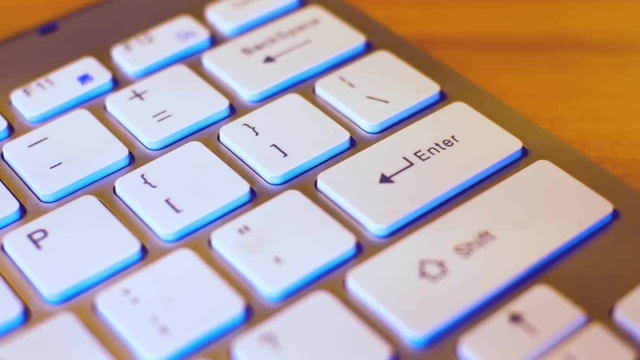 Have you ever wondered how the web works? In this lesson, I'm going to tell you exactly what happens the moment you type the address of a website into your browser and hit enter. As part of this, we're going to talk about a few important concepts and terms. 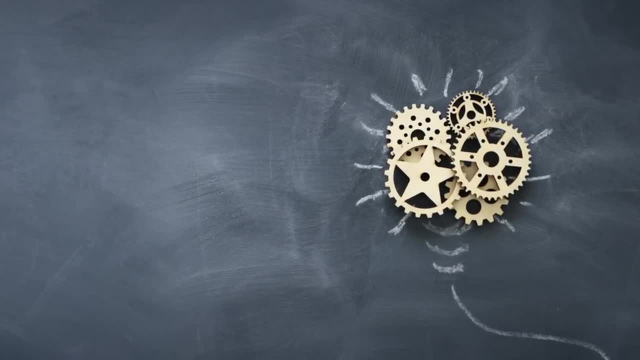 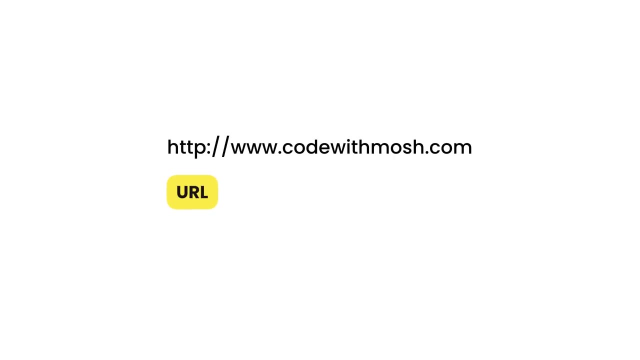 that you need to know as a web developer. So let's say we launch our browser and head over to a website like codewithmoshcom. Now this address that we have in the browser address bar is called a URL, which is short for Uniform Resource Locator. 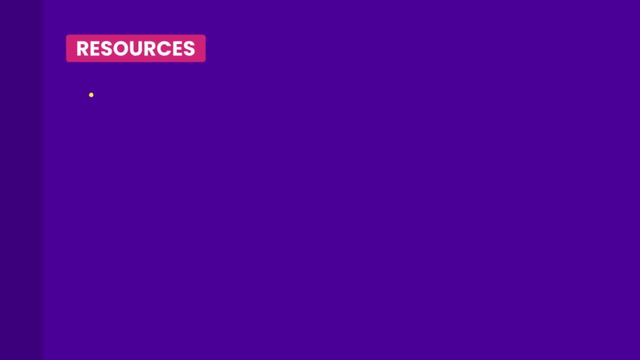 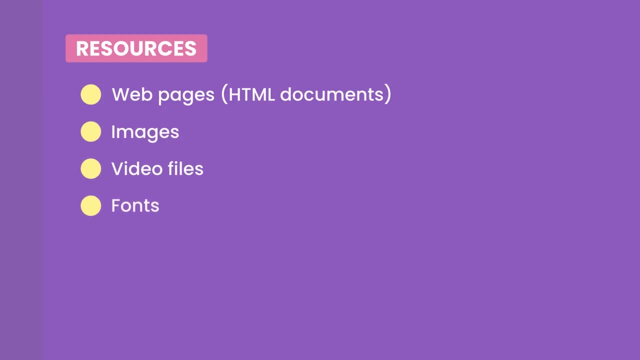 Basically, it's a way to locate a resource on the internet. Resources can be webpages, also called HTML documents. They can be images, video files, fonts and so on. So we type the URL of a website and hit enter. What happens now? Well, there are. 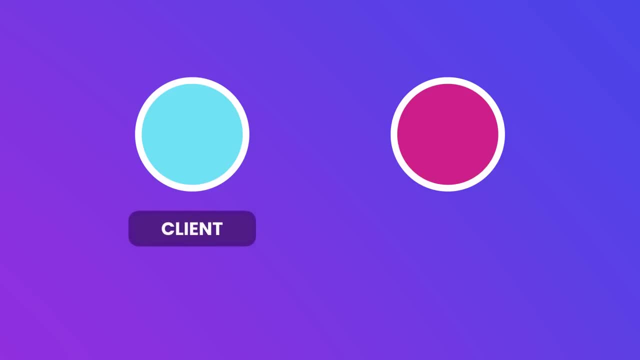 two pieces involved here, One of which is the user that you're talking to. So this user, AZ hashtag insbesondere, has correctly 残人 ABRUZ stressed in the browser, also called the client and the computer or computers that host our target. 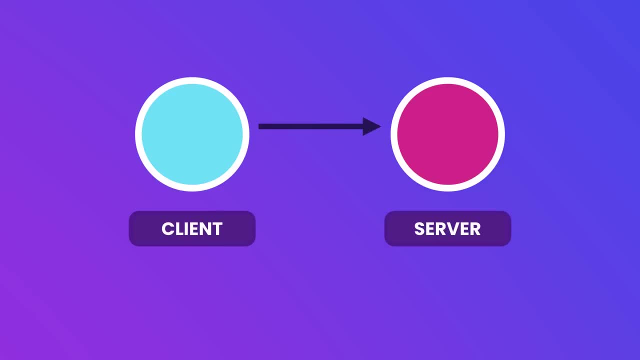 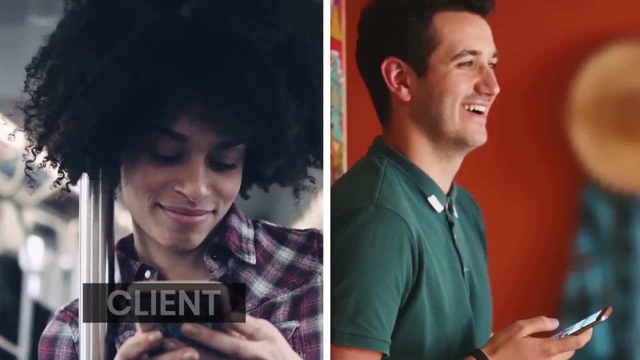 website. We refer to this as Web servers, or servers for short. This is what we call the client server model. The client requests a service, The server provides that service. So a browser sends a message to a server and says characterized. 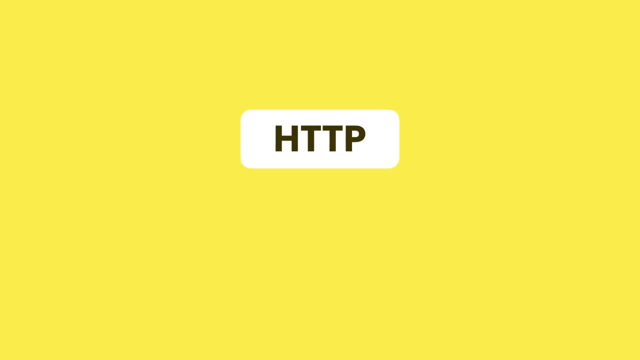 the server receiving the message. Now back to our example. this message is formatted based on a protocol called HTTP or hypertext transfer protocol. You've probably noticed it before, but never knew what it is. In simple terms, HTTP is a language that clients and servers use to talk to each other. It's not a programming. 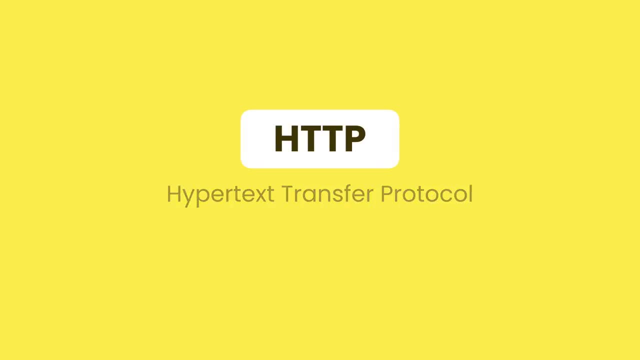 language. it's just a plain textual language for communicating over the internet. We also have HTTPS, which is HTTP with encryption, So the messages exchanged between the client and the server are encrypted. Here's a simplified example of an HTTP message With this message: 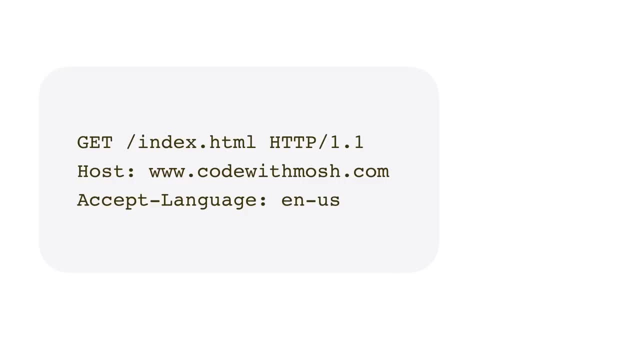 the browser tells the server what it's looking for. So on the first line it says that it wants to get a page or a file called indexhtml using HTTP version 1.1.. Indexhtml often represents the homepage of websites. On the second line we can see the host, that is codewithmoshcom. 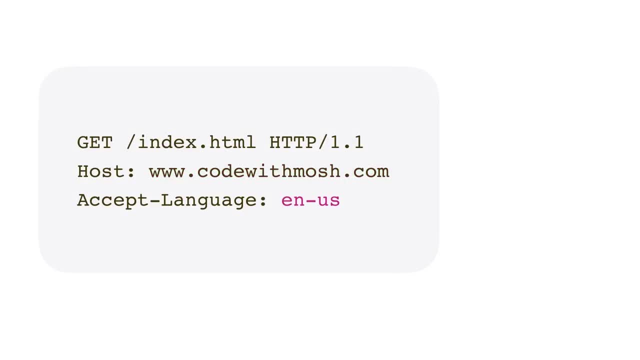 And on the third line, we can see the language that the client can accept, In this case, English. Now, don't worry about memorizing any of this. All I want you to understand here is that this message is structured based on the HTTP protocol that clients 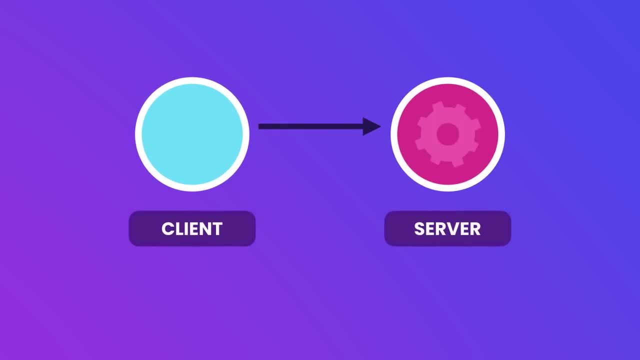 and servers understand. So the server receives this message, it figures out what the client is asking and then it will send a message back to the client. The first message is called an HTTP request and the second message is called an HTTP response. Every data exchange. 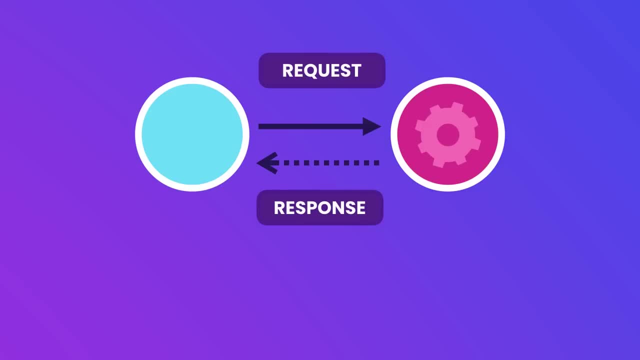 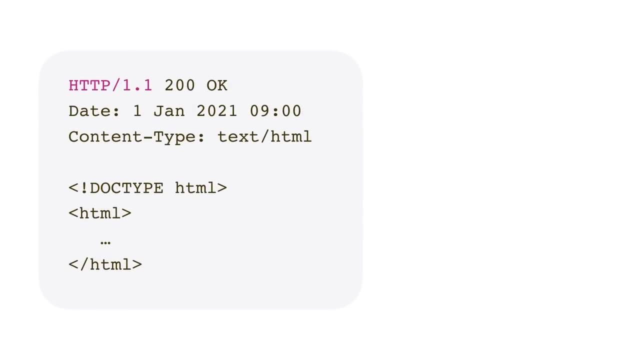 using the HTTP protocol involves two messages: a request and a response. Now what is in the response? Here's a simplified example. On the first line, we see the version of HTTP protocol used, followed by a number, which is the status code. 200 means successful or okay. 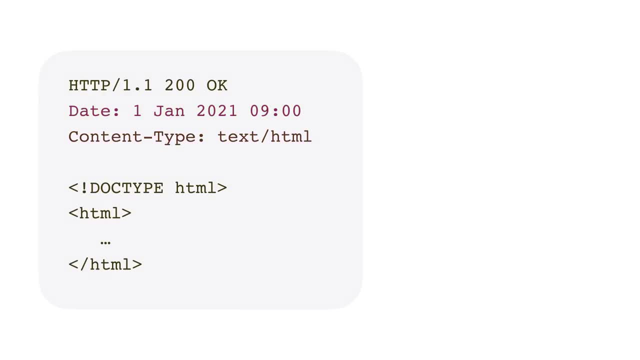 Right below that we can see the date and time of the response. Next, we can see the type of content the server is sending back to the client, In this case text slash HTML, And after that we can see the HTML code or the HTML document that represents the home page of code with moshcom. 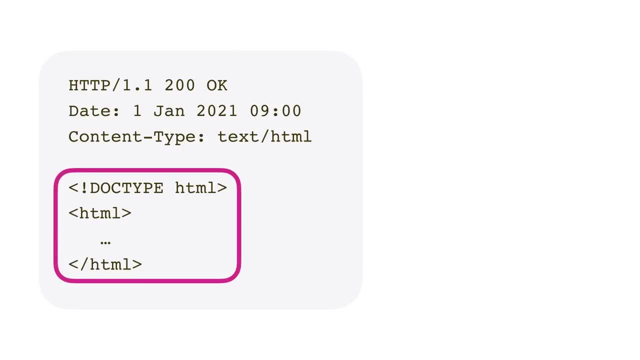 Of course, the actual HTML code is way longer. Now, as the browser reads this HTML document, it constructs what we call a DOM or a document object model. Don't let this fancy name scare you. This is a model that represents the objects, or. 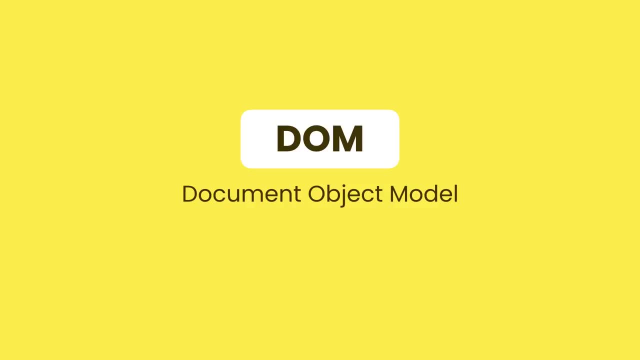 elements in our HTML document. What are these elements? All the building blocks of our page, like paragraphs of text, images, links and other stuff. You will see this in action in the next lesson. Now, as the browser is reading this HTML document that is returned from the server, it discovers, 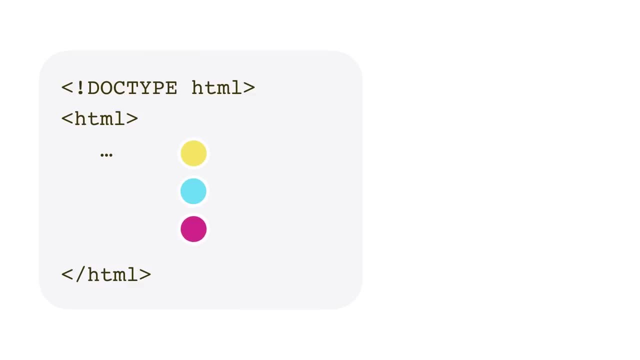 references to other resources in this document, like images, fonts and other stuff. Each of these resources has an address or a URL. So for each resource the browser sends a separate HTTP request to the server to fetch that resource. Many of these- 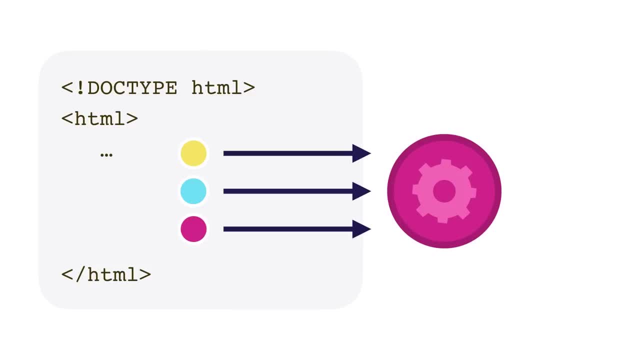 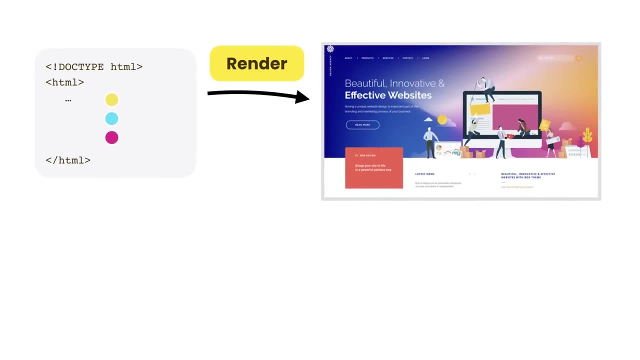 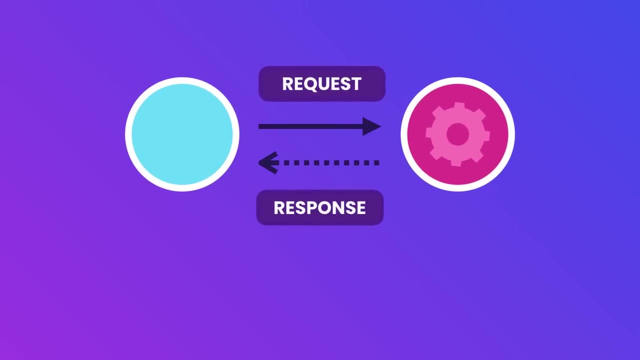 HTTP requests are sent in parallel, so we can see the page as quickly as possible. Once the browser has all the necessary resources, it will render the HTML document. Rendering an HTML document means displaying it. It's a fancy technical term we use often. So, in a nutshell, our browser. 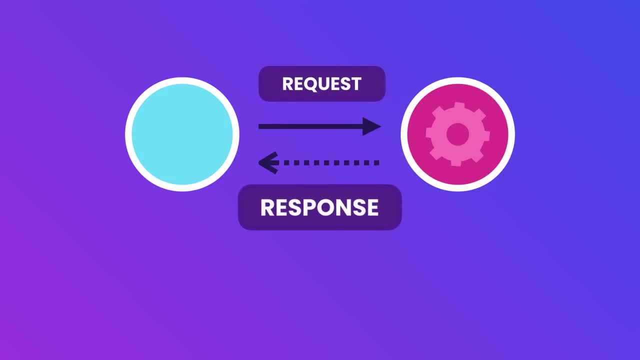 sends an HTTP request to the server and receives an HTTP response. This HTTP response contains an HTML document. The browser reads that HTML document to construct a document object model and render the page. In the next lesson I'm going to show you all of these steps in action. 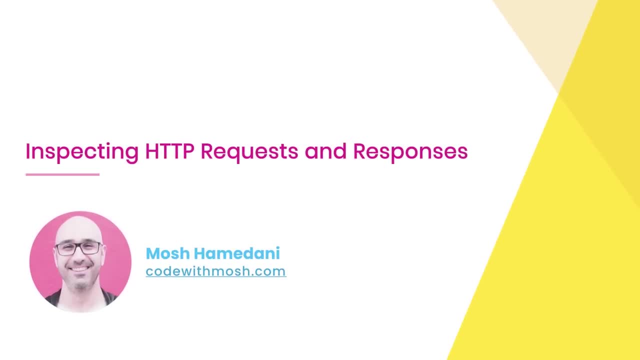 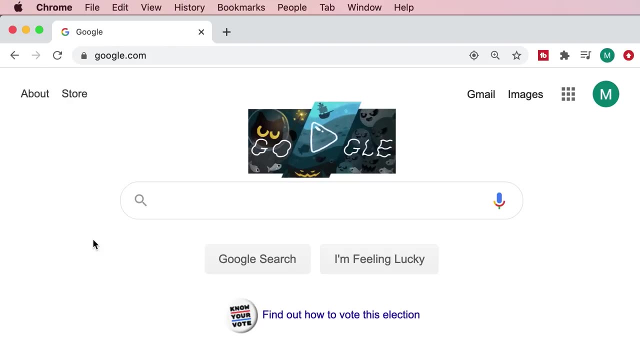 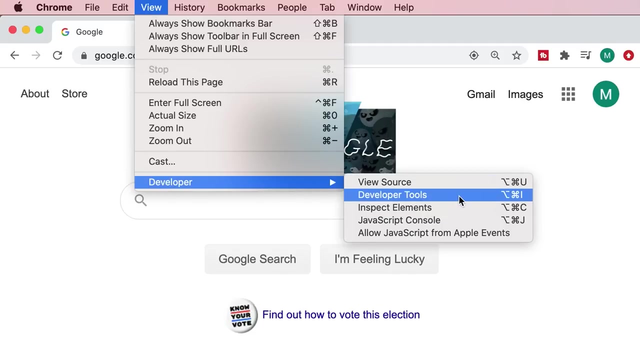 Alright, let's see HTTP requests and responses in action. So open up Chrome and head over to googlecom. Now we need to access Chrome DevTools. This is a very powerful tool used by front-end developers. So on the top, we go to view developer developer tools. Now look at the shortcut. On Mac, it's alt or option command and i. On windows it's obviously different, but remember the shortcut because it's much faster to access the devtools via the keyboard. 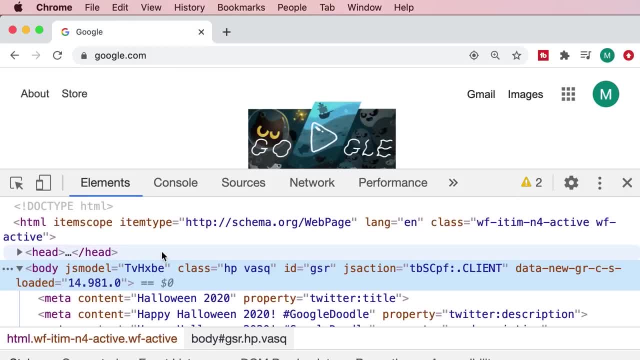 So here's the devtools. the first time you see it it might appear a bit intimidating, but trust me, it's much easier than you think. Throughout the course, you're going to learn more about the devtools. So here's the devtools. 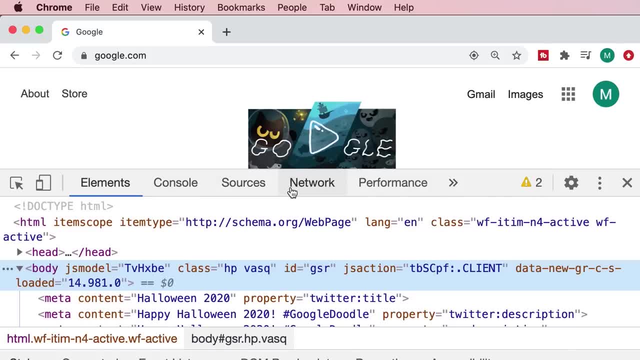 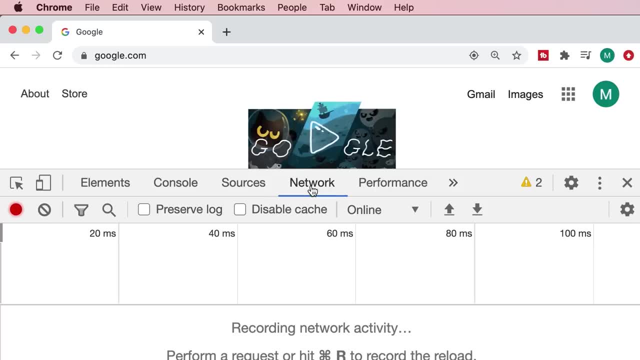 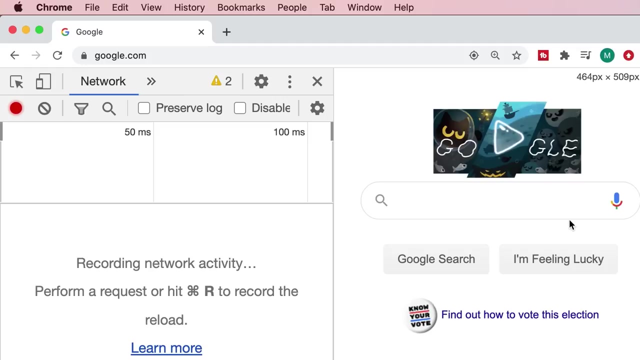 Here we have a few different tabs: elements, console, sources, network and so on. In this demo we're going to go to the network tab so we can inspect the network traffic to and from googlecom. Now, by default, devtools is docked to the bottom of the screen. We can dock it to the left, to the right or undock it as a separate window. So over here we can dock it to the left side. 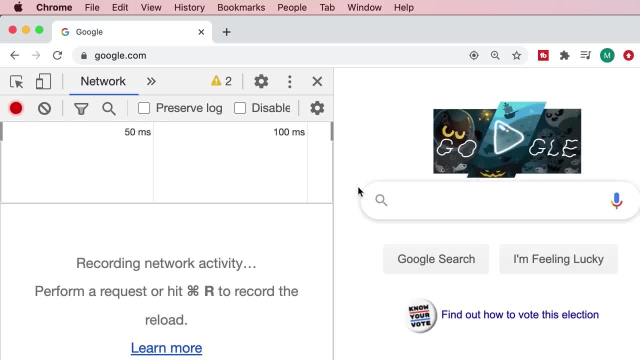 A lot of front-end developers like this layout, So they put devtools to the left side. they have their website on the right side. Now in this demo, I'm going to undock it as a separate window so we have more space to work with. 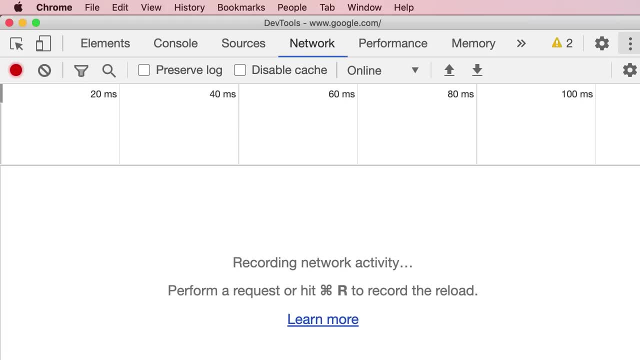 So let's undock it. good, Now we need to refresh our website. As you can see over here, on mac we can press command and r. on windows it's probably control and r. Alternatively, we can go back to this window and press the refresh button. 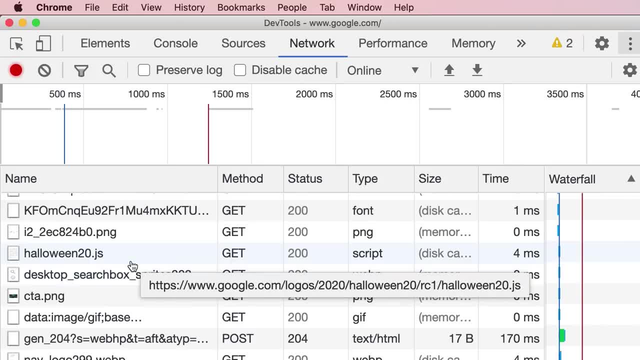 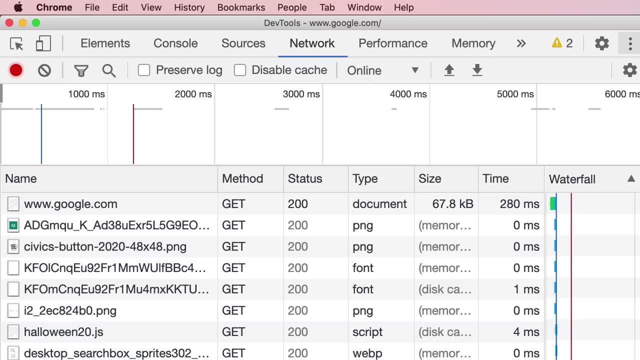 Now back to the dev tools. look at all these items over here. These are the http requests that are sent from our browser to googlecom. As you can see, they're totally 45 requests, and here's the amount of data transferred over the network, So in this case, just over 94 kilobytes. 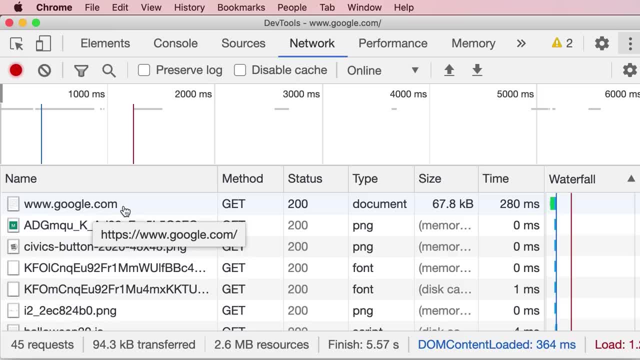 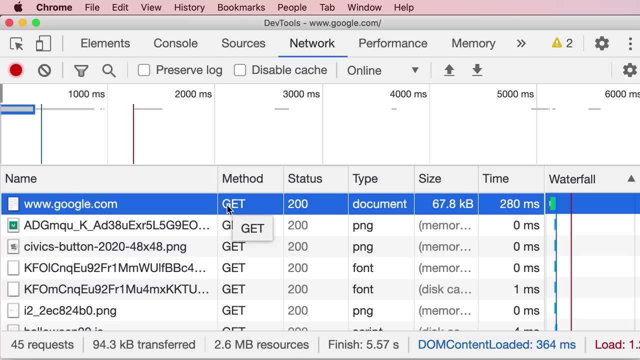 Now look at the first item in this list. This is the first http request that chrome sent to googlecom. As you can see, with this request the browser wanted to get a document, and this is the first request that chrome sent to googlecom. 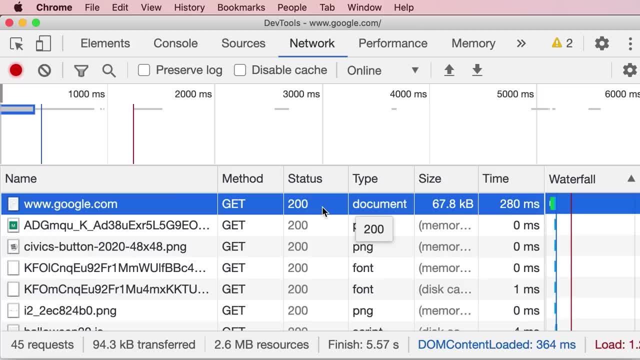 And the status of this request is 200, which means okay. Over here you can see the amount of data transferred over the network for this request and the time it took to get the response. Now, if we click on this request, we can see more details about it. 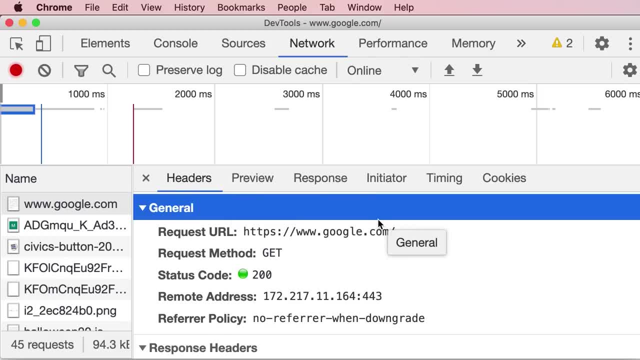 So here on the headers tab, we can see all the headers of our request and response. So here are some general headers like request url, request method, which is get status code, that is 200, we talked about it- remote address. this is the new make representation. 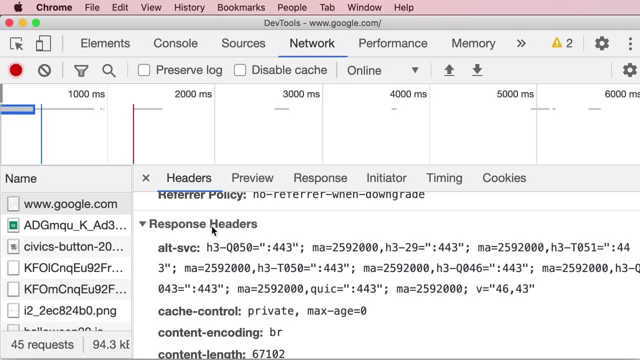 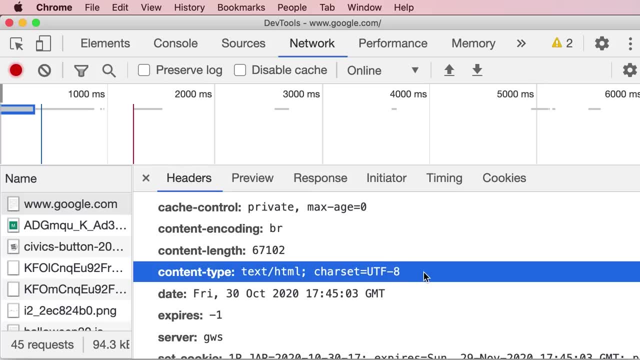 of googlecom. Now down below, we have response headers. there's so many headers here, you don't have to worry about them. but as an example, look at content type. we talked about this in the previous lesson, So the type of this response is text slash html Below that. 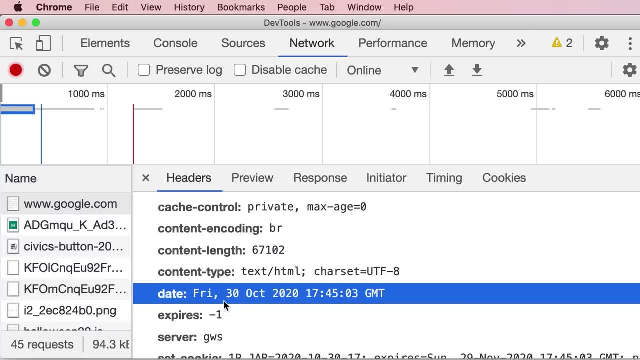 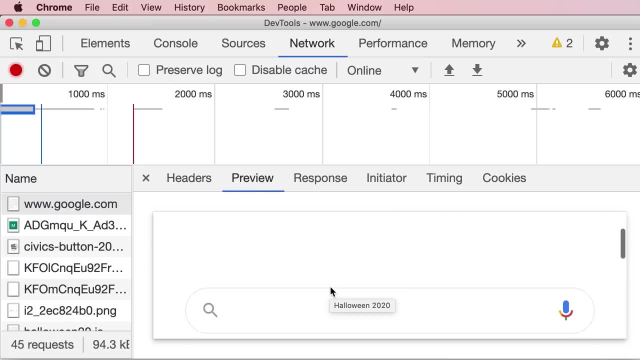 we have the date and time of the response. Now, if we click on the preview tab, we can see a preview of the html document that is returned from the server. so this is the homepage of google. Now, in this html document we have references to other resources. 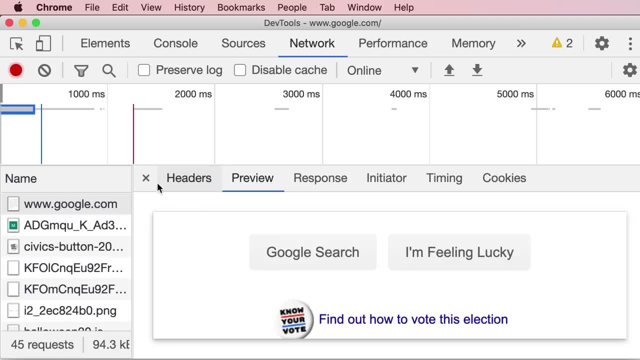 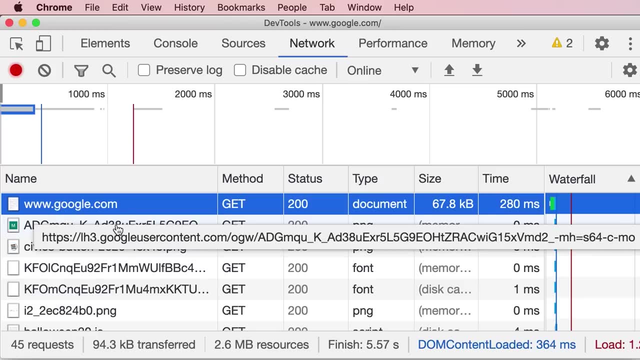 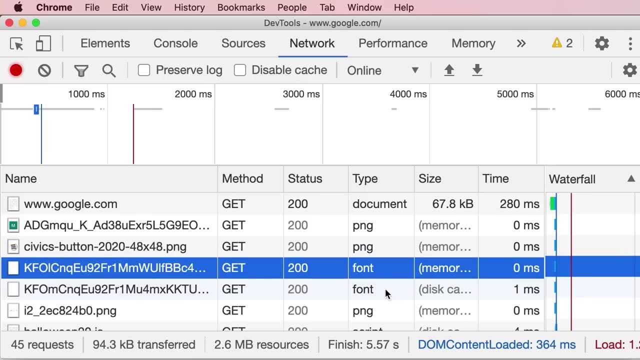 like images, fonts and so on. So all these subsequent requests are sent to download those resources. So right below the first request we have a request for downloading a png or an image file. Here's another request for getting another image. we have two requests for getting two different fonts, and so on. 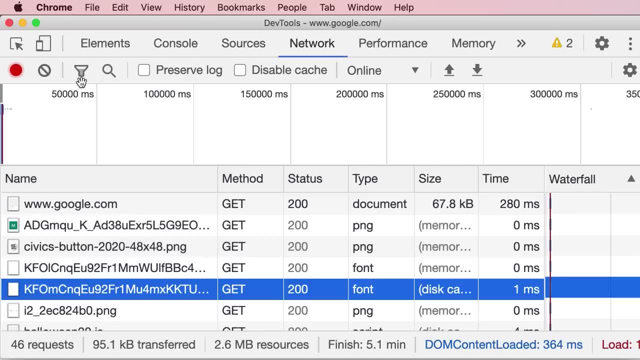 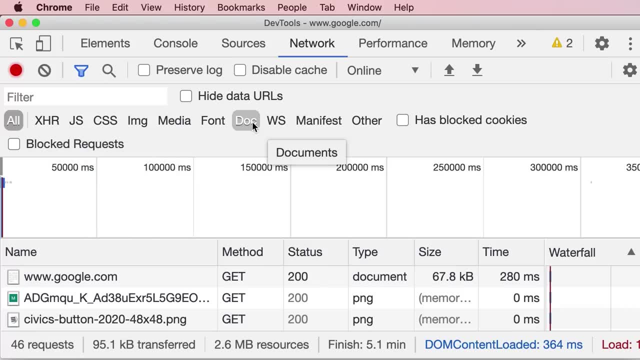 Now we can easily filter this list, so let's click on the filter icon here. By default, we see all requests, but we can filter by request type. For example, we can select doc to see requests for downloading html documents or font. 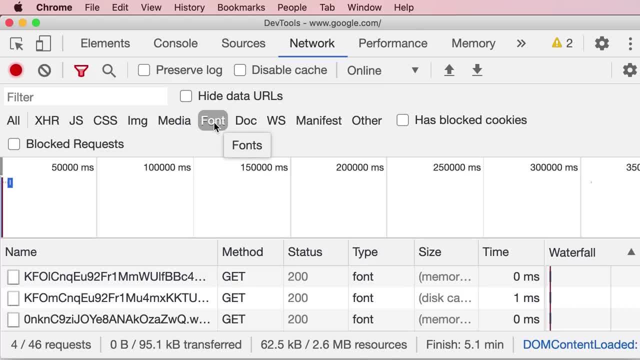 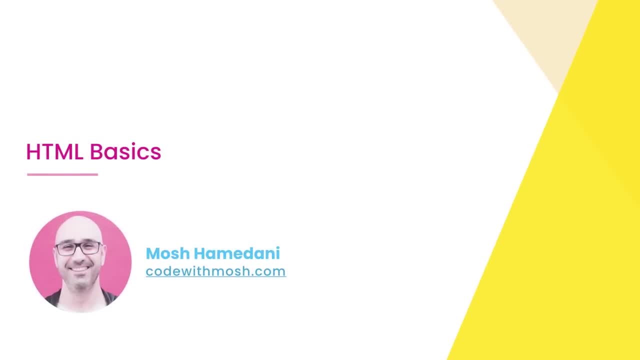 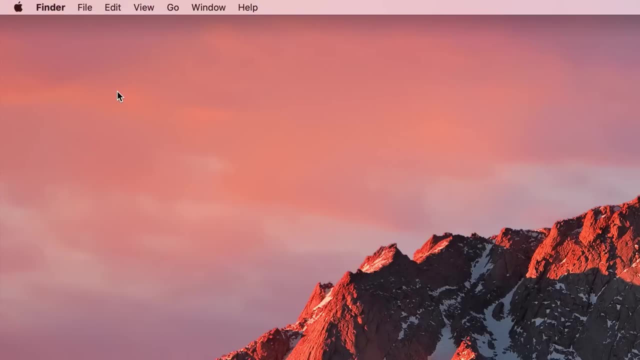 to see the requests that were sent to download fonts and so on. Next, I'm going to show you how to create your first html document. Alright, first things first, here on your desktop or anywhere on your computer, right click and create a new folder. I'm going to call this html. 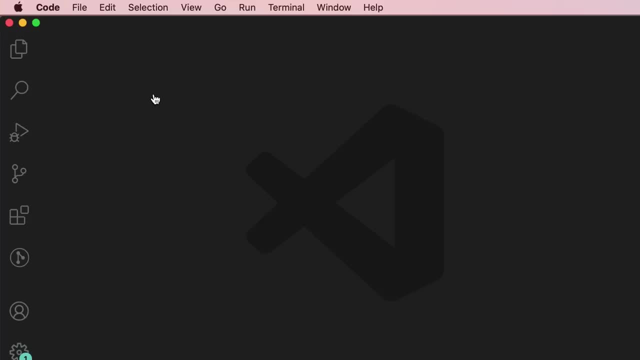 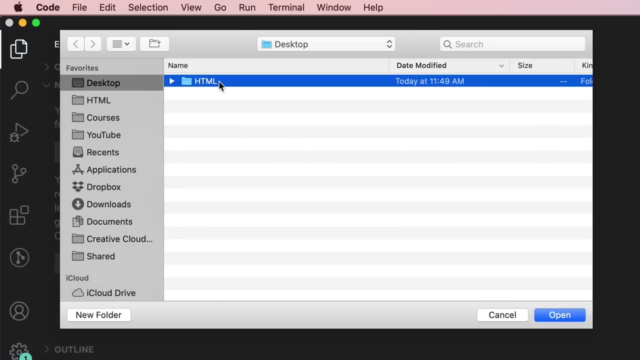 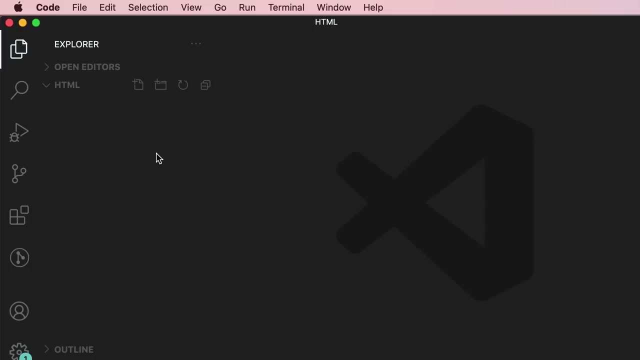 but we could call it anything. Now let's go back to vs code and open the explorer panel. Then we go to open folder and open the folder that we just created. Good, now this folder is currently empty, so let's add a new file here called indexhtml. 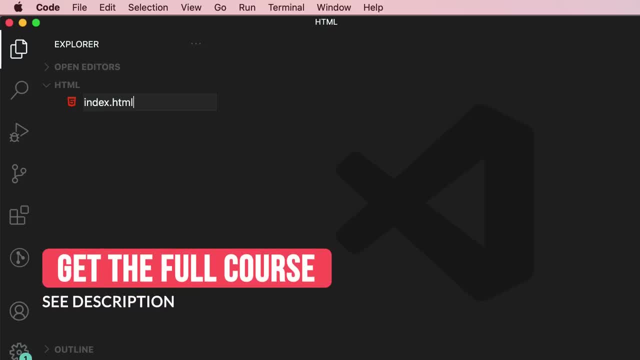 As you can see, this is the file that we just created, so let's add a new file here called indexhtml. As I told you before, indexhtml often represents the homepage of websites, So let's go with that. Now we can close the. 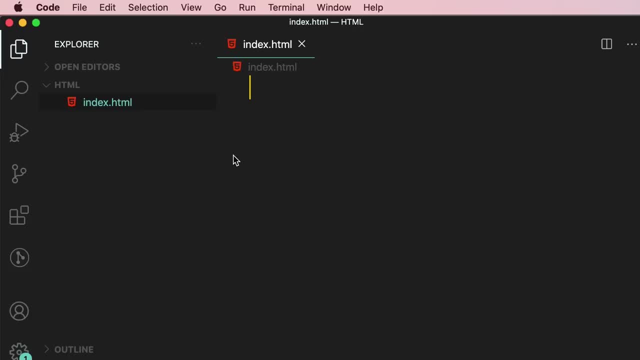 explorer panel by pressing command and b on mac, or control and b on windows. Good, Now the first thing we need to do here is to tell the browser that this is an html5 document. So we type a left angle bracket. now look at. 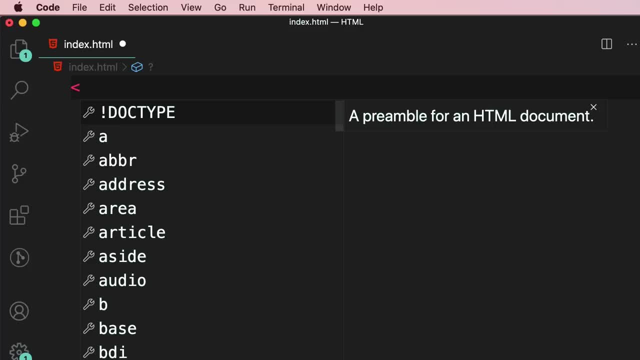 this suggestion list. the first item here is doc type or document type. Let's press enter Or tap vs. code generated this piece of code for us. So with this line of code we can tell browsers that this is an html5 document. This line of code here is called doc type declaration. 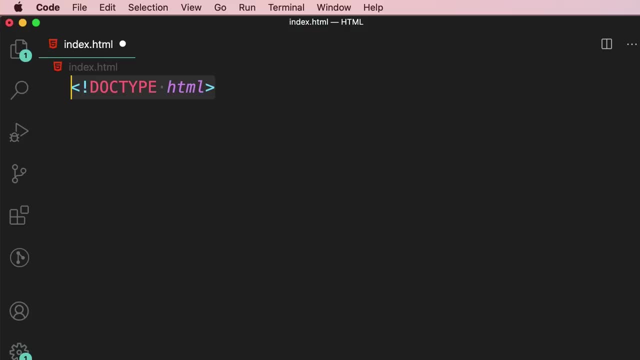 In the previous versions of html, our doc type declaration was so long, it was so messy, but html5 solved this problem, So all we have to type is doc type html. And, by the way, html is not a case sensitive language, which means it's not. 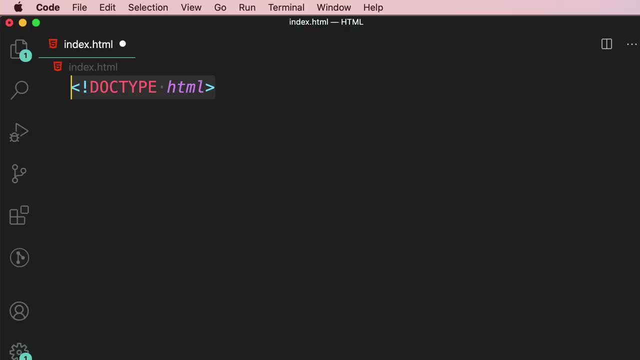 sensitive to uppercase and lowercase letters, But conventionally speaking, we type everything in lowercase except doc type. This is just a convention. We could type this in lowercase and that's perfectly fine. So let's revert it back Now, right after this. 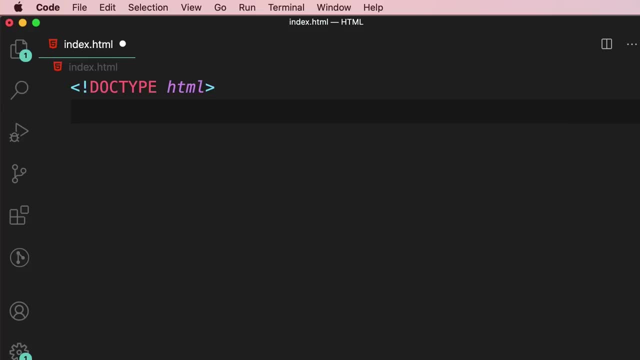 we need to use our html elements to define the structure of this webpage. The first element we're going to use is the html element, So we type html and then press tab or enter Once again. vs code generated this piece of code for us. 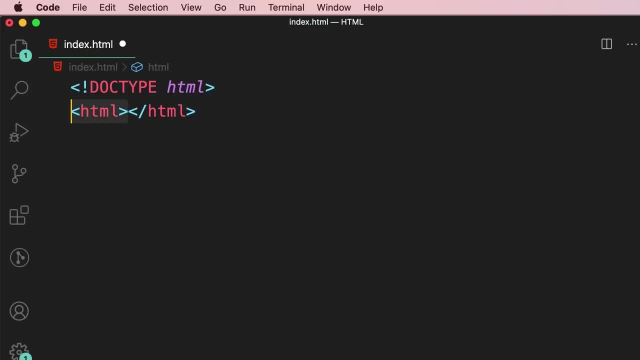 So what we have here on the left side is called the opening tag and what we have on the right side is the closing tag. So most html elements have an opening and a closing tag, but there are exceptions, as I'm going to show you later. 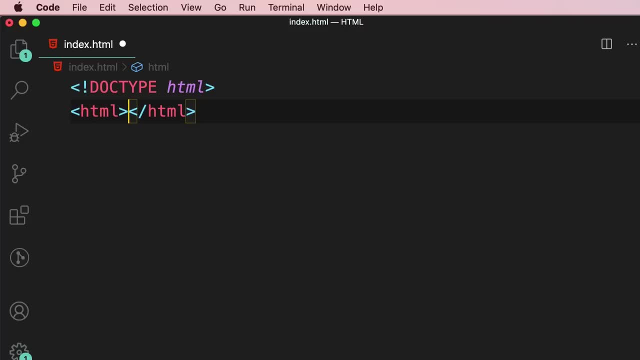 in this video. Now, inside this element, we're going to add additional elements. Now, because I don't want to type everything in one line, I'm going to press enter. that's better. Now, here we're going to add two elements: head and body. 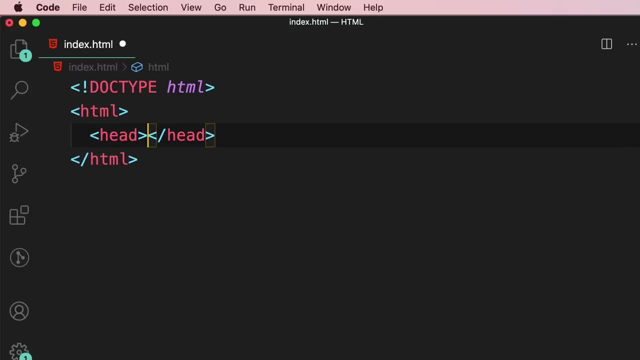 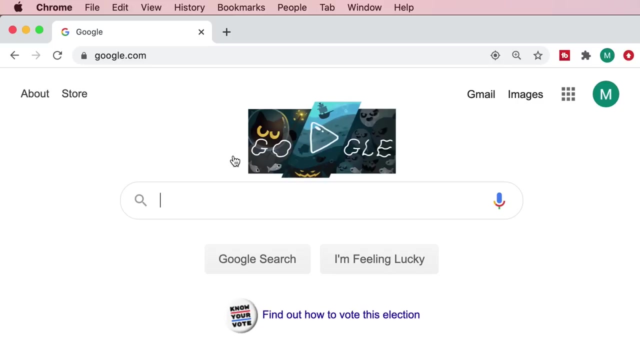 So I'm going to type this in here Once again. we type head, press tab good and then body. We use the head element to give browser information about this page. For example, here we can use the title element to specify the title of this page that appears. 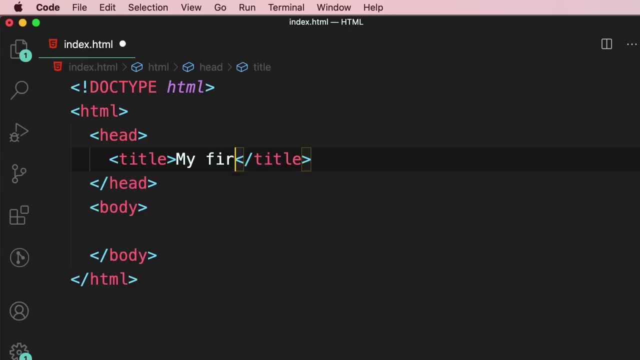 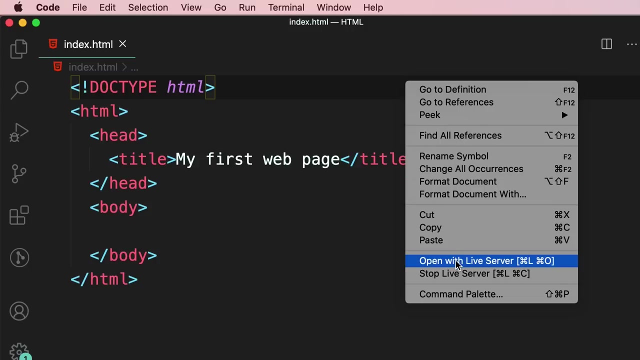 in the browser over here. So let's type my first webpage. Now let's save the changes by pressing command and s on mac or control and s on windows. Good, Now, before going any further, let's right click somewhere and go to open with live server. So we're going to open this page. 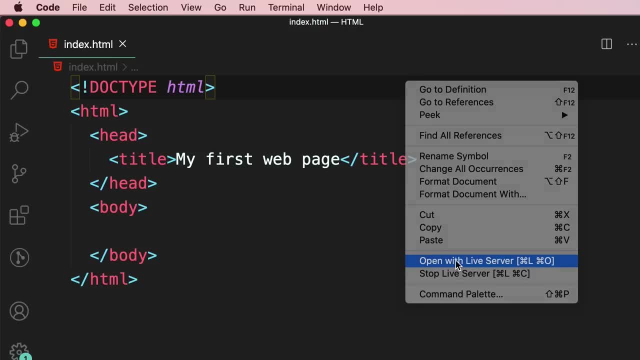 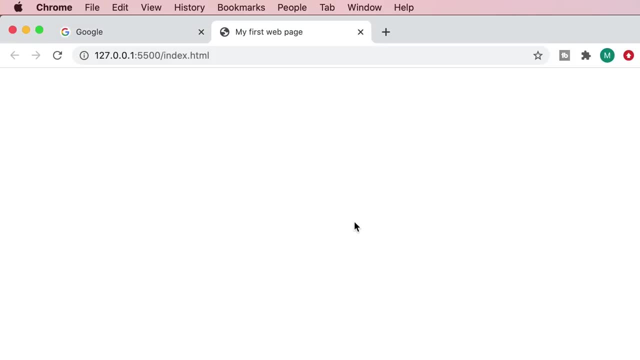 using the development server that we just installed. Okay, Alright, take a look. So our page is currently empty because we haven't added any elements inside this page and over here we can see the title that we just typed: My first webpage. 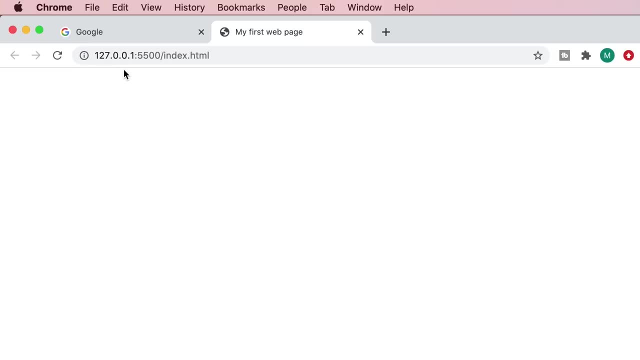 Now look at the url or address of this page. We have 127.0.0.1,. this number or this ip address represents the local computer. It's globally known, so everybody knows. 127.0.0.1 references the current computer. After that we have a colon. 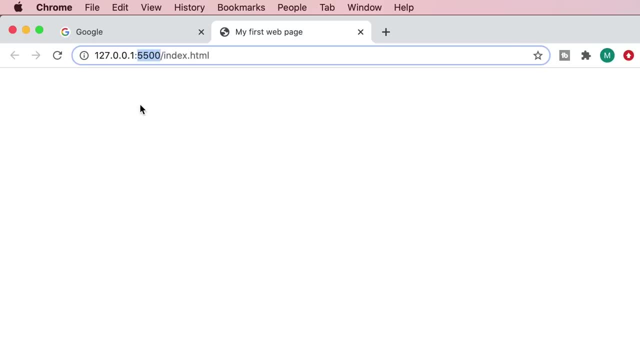 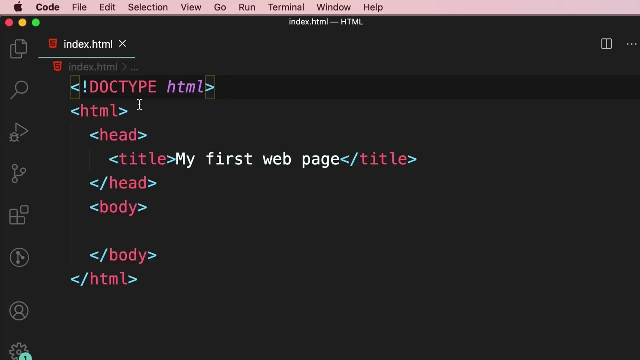 and then we have the port number on which our web server is listening. So our web server is waiting for http requests on this port. Okay, Then we have a forward slash followed by the name of our file, indexhtml. Now back to vs code inside the body element we're going to. 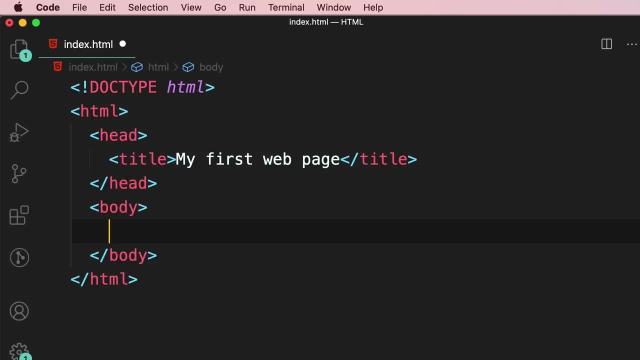 add elements that would appear on our page. So let's say, we want to display a tweet. What elements do we need here? An image and some text elements. So we type img, short for image and then press tab: Here's our image element. Now this image: 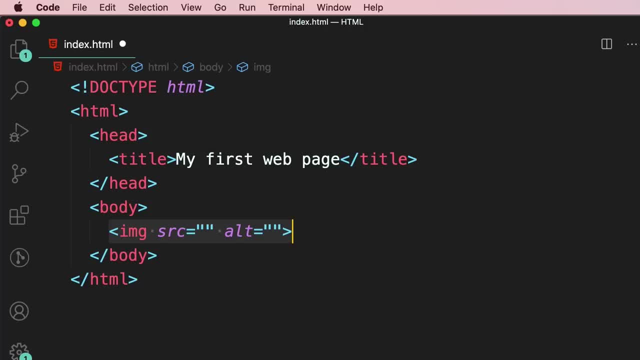 element is different from the other elements we have created so far. Can you tell the differences? There are two differences here. The first difference is that here we don't have a closing tag, We only have an opening tag, Because the image element cannot have any child elements. That's the reason Now in the previous 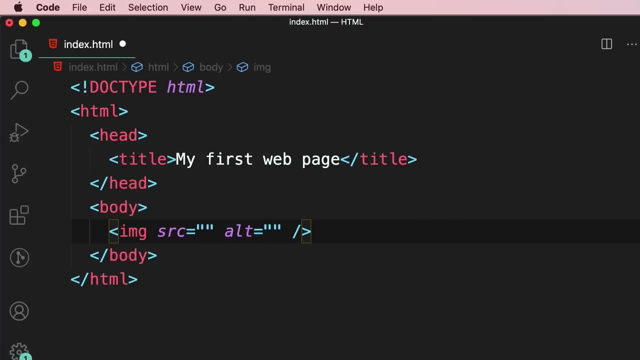 versions of html. we used to add a forward slash here, and this represents a self closing tag, But we don't have to do this in html5, so I'm going to keep the code simpler. Now, here we have two attributes: source and 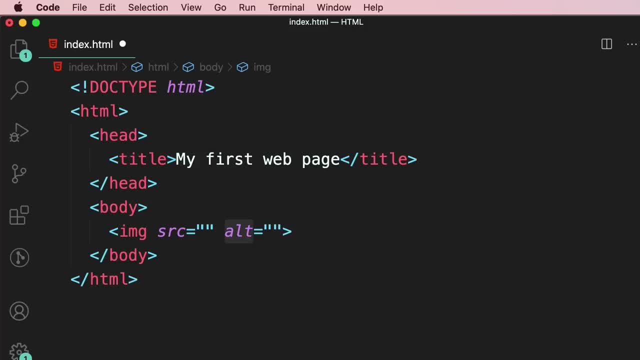 alt With these attributes, we can supply additional information about an element. So we use the source element to specify the path to our image. So let's open up the explorer panel one more time by pressing command and b on mac, or control and b on windows. 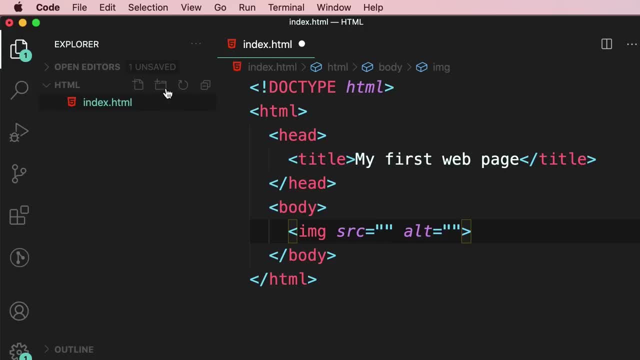 Here I'm going to create a new folder called images. Now, for this demo, I'm going to use my own image, which you can also download right below this video, but you can use any image that you want. So here's my image. I'm going to drop it. 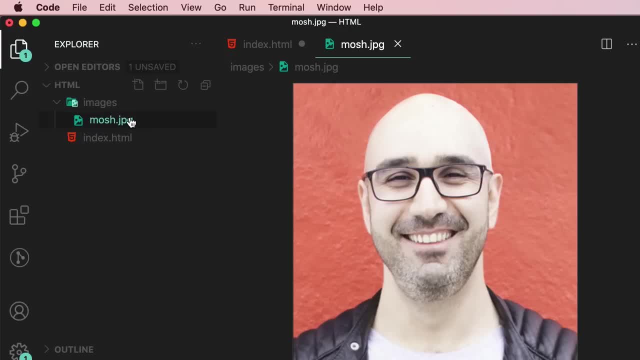 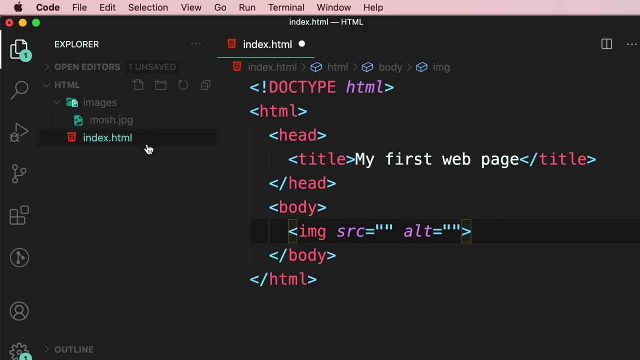 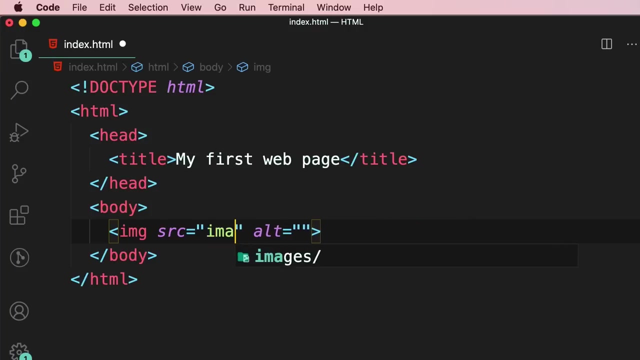 onto the images folder. It's right here. Now let's close this window. good. So where is this image relative to our indexhtml file? It's inside the images folder, right? So here in double quotes we type images: slash moshjpg. 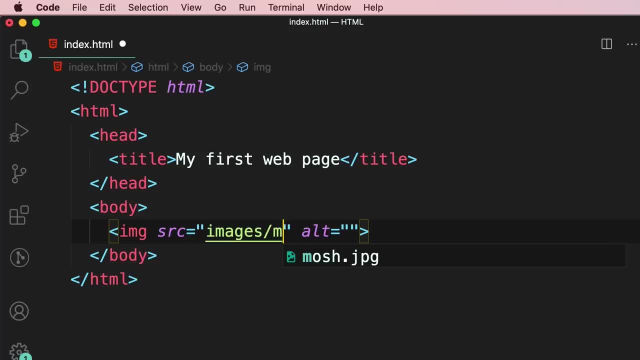 Now. vs code is suggesting this name, so we can press tab to complete the code. Beautiful Now. alt is short for alternative text and we use this attribute to give the browser some text to display in case the image cannot be displayed. We'll talk about this in more detail in the future. 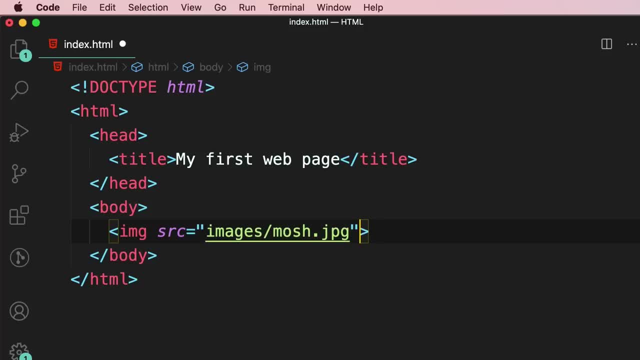 So for now, I'm going to delete this attribute. good, Now, after the image, we're going to add a text element. So we type p, that is short for paragraph tab, and here we can type my twitter handle. so after that, we're going to add another text element. 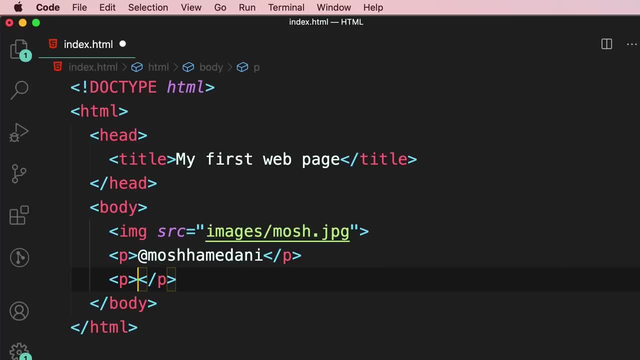 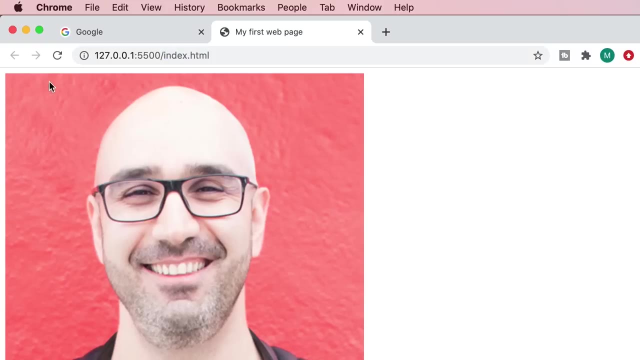 and here we can type the body of our tweet. So I love to teach you HTML Perfect. Save the changes. now back in the browser. our page refreshed automatically. This is one of the beauties of live server, So we don't have to manually refresh the page every time we make changes. 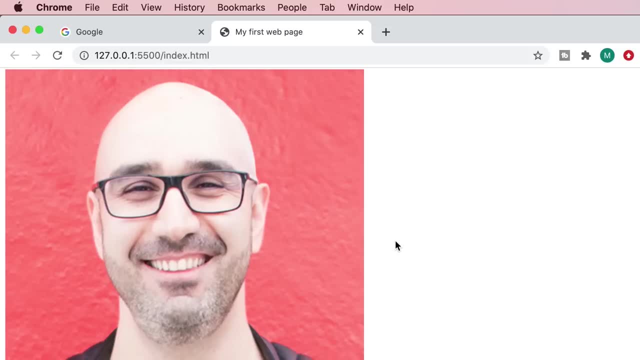 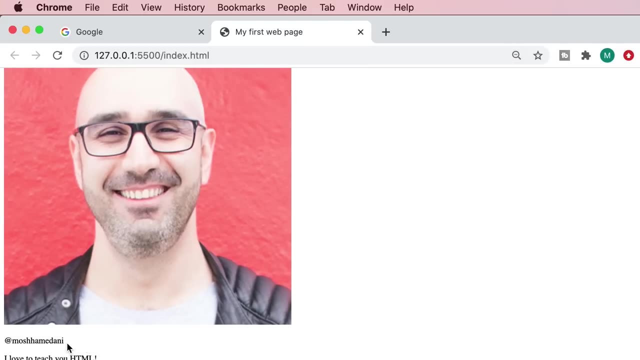 Now look at what we have here. So we have my image and right below that we have two text elements. Take a look. unfortunately, they're not very visible. Obviously, this doesn't look like a tweet Because we haven't applied CSS yet. As I told you before we use HTML, 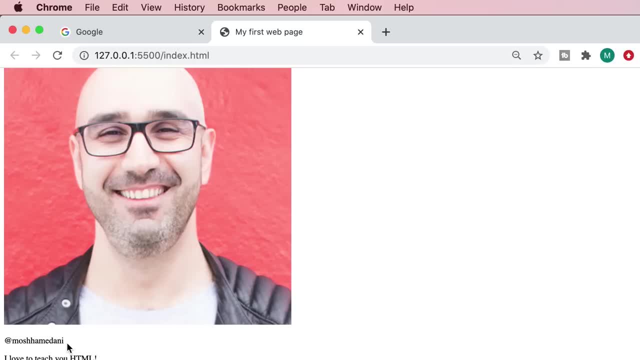 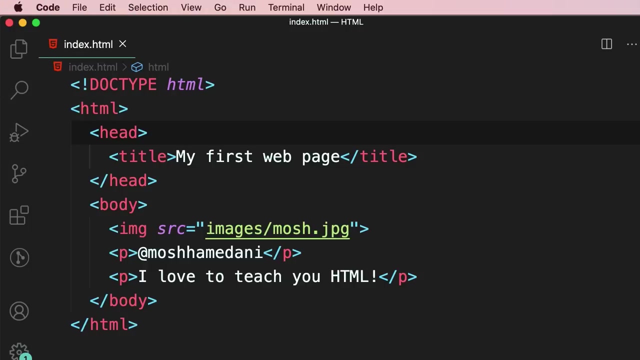 to define the structure, or the building block of our webpages. In the next lesson, I'm going to show you how to apply CSS. so our page looks kind of like a real tweet. Alright, now let's see how we can use CSS. 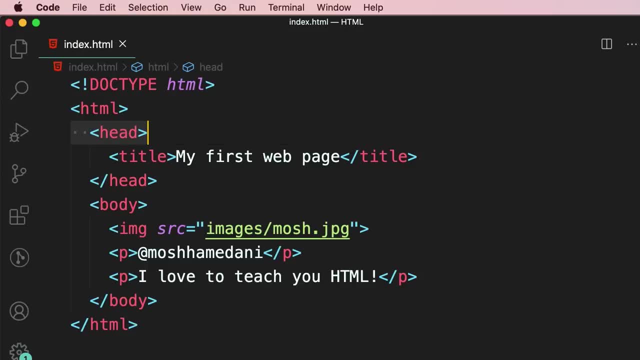 To improve the look and feel of this page. Look at our head element. Currently, we have a single element inside the head element. That is our title element. right Now, after the title, we're going to add another element called style. This is where we're going to write. 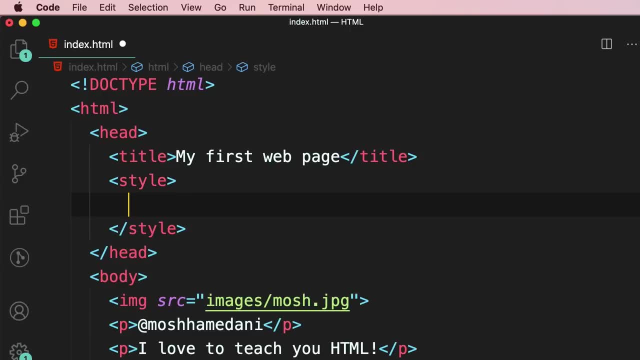 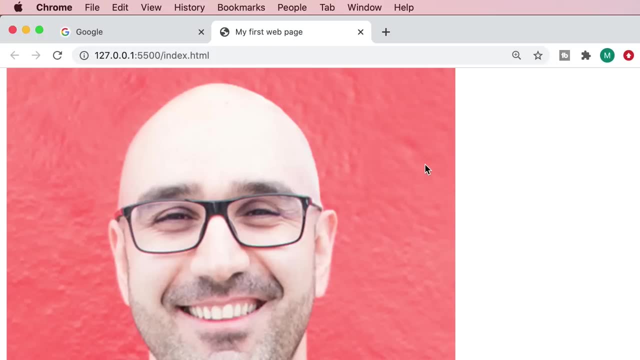 our CSS code. So in between style tags, we're going to write a bunch of CSS rules. First, we're going to work on this image. Our image is currently too big, so let's make it a bit smaller. Back to VS code. 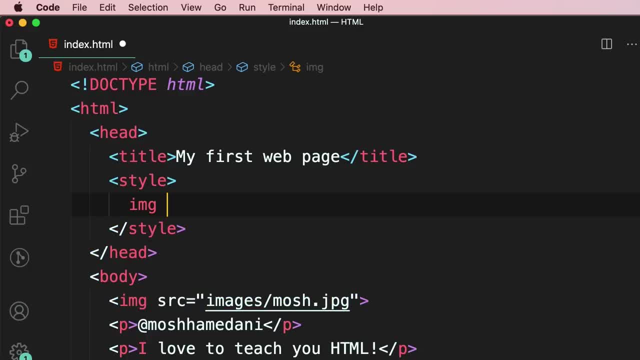 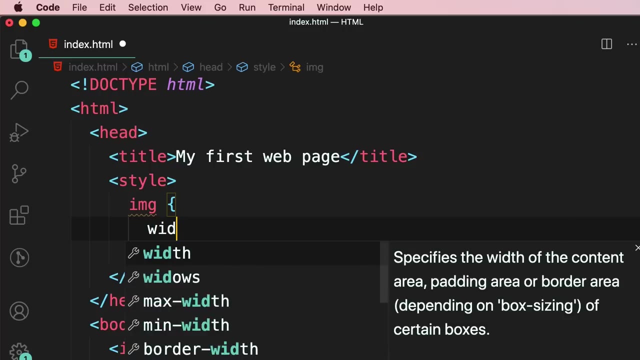 Over here we're going to type img to reference our image element. Then we type a pair of curly braces and inside the braces we write one or more CSS declarations. Each declaration contains a property and a value. So here we can set the width property to, let's say, 100. 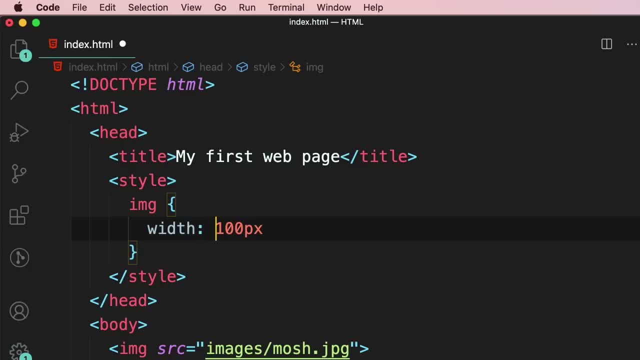 pixels. So we type the property colon and then the value, And then we terminate this line using a semicolon So we can write multiple CSS declarations. Now let's save the changes Back in the browser. our image looks smaller. that's a lot better. 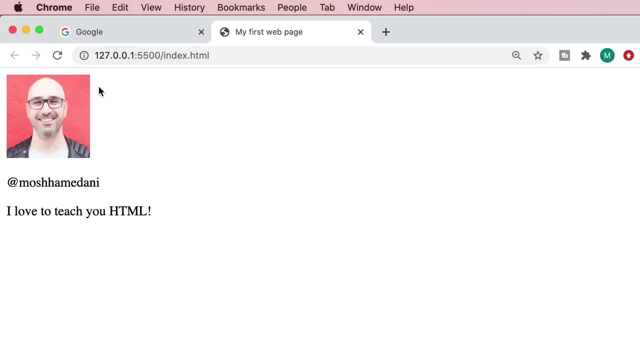 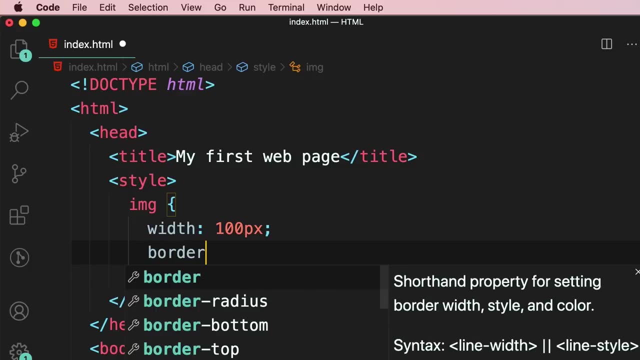 But look at the edges. the edges are so sharp, I would like to make them a bit round so they appear softer. Now back to our rule. here we're going to set the border dash radius property to, let's say, 10 pixels. Now don't worry about memorizing. 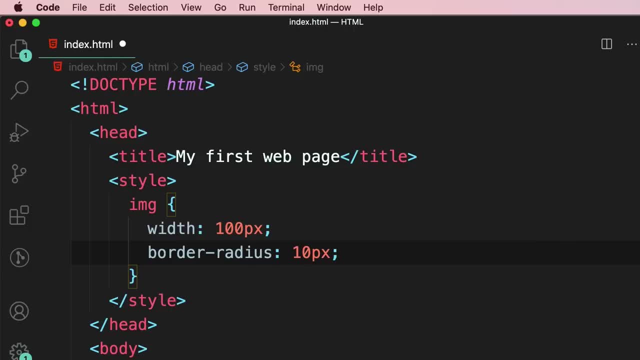 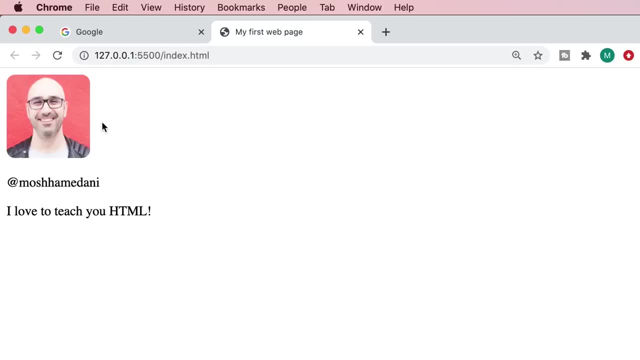 any of these properties. we're going to go over them several times throughout the course. In this lesson, I just want you to get a sense of what it's like to use CSS. Okay, So same changes. now look, the edges are round and look softer. Now let me show you a trick. 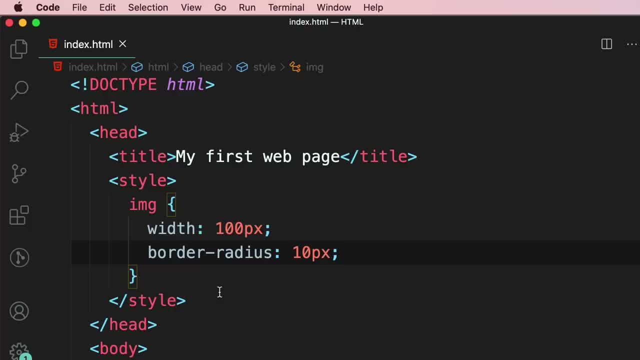 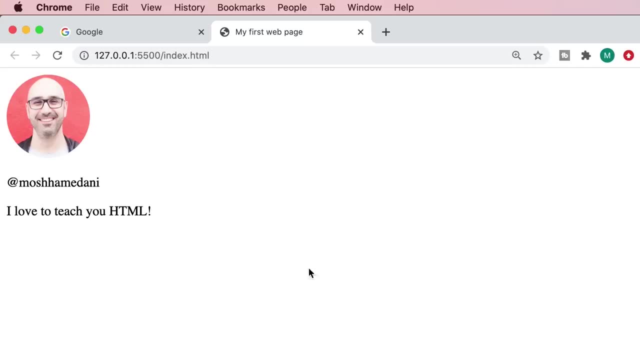 If we set border radius to a value that is half of the width, we'll get a round image. So I'm going to set this to 50 pixels, and here's the result. That's a lot better. Now our elements are stacked vertically. I want the image. 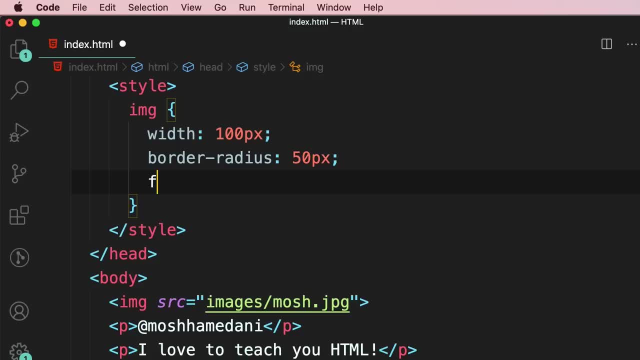 to be pushed to the left side. So let's set the float property to left. This will push the image element to the left side of our text elements. Take a look, So that's a lot better, but our image is so close to the text I want to add. 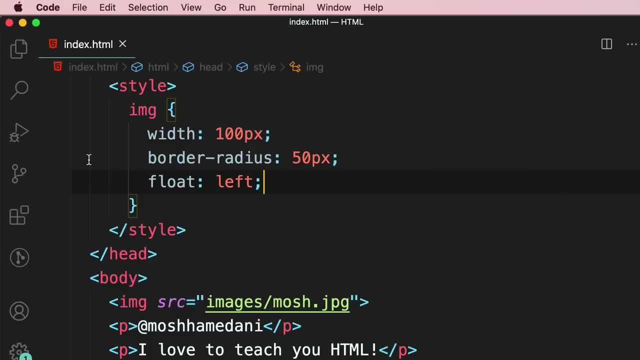 some space after the image. So here we use another property called margin dash right, We can set it to 10 pixels. Save, and that's a lot better. Now let's make the user name bold. So we're going to repeat one more time. This time we're going to apply a rule. 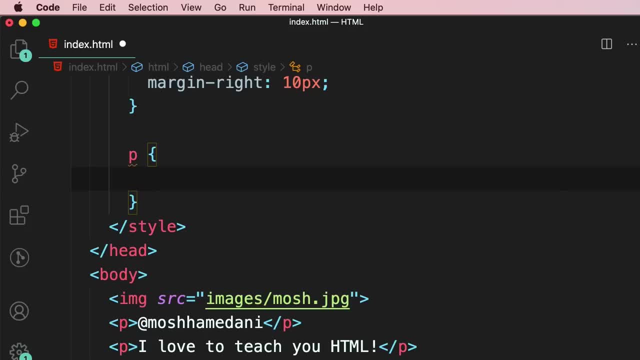 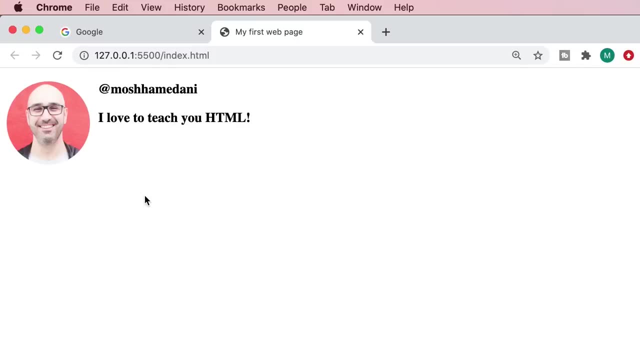 to our paragraph element. So here we're going to set the font dash weight property to bold. Take a look, See what happened. Both our text elements are bold, But what if you want to apply this style only to the user name? 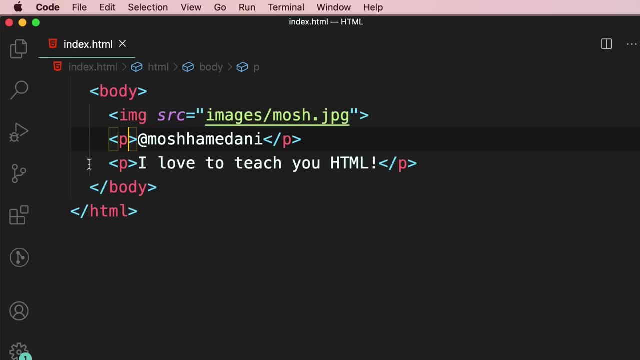 Well, we have to separate these two paragraph elements, So I'm going to give the first paragraph element an attribute called class. So class equals double quotes. Class is short for classification and we can use this attribute to put this element inside a different class or a different category. 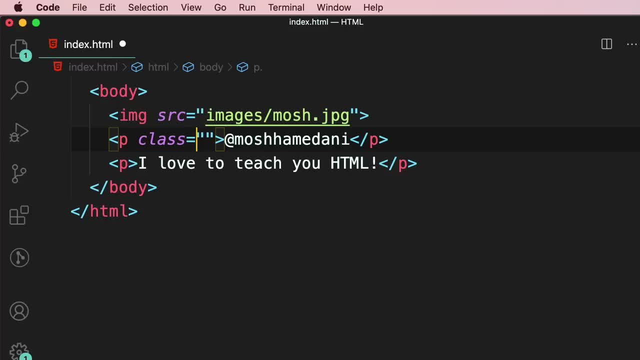 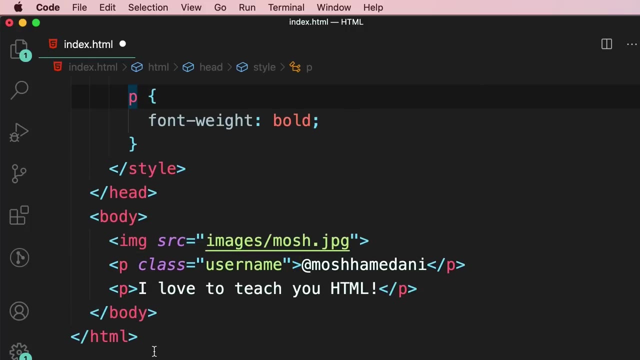 Just like the products in a supermarket. In a supermarket, we have products in different categories, right? So I'm going to put this paragraph element inside a class or inside a category called user name, And then I'm going to change this rule. So this rule is: 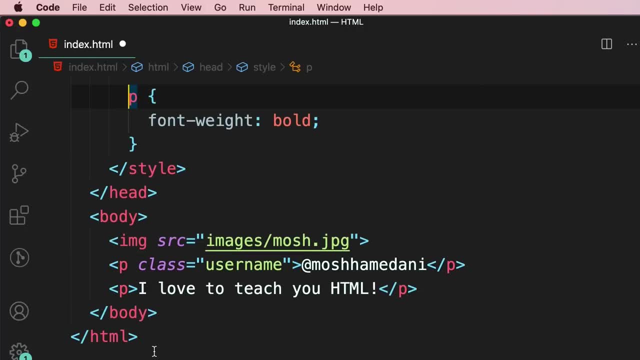 currently applied to all paragraph elements, but I want it to be applied only to paragraph elements with a user name class. So right after p we type dot user name. Now we can also remove p and this rule will apply to all elements. 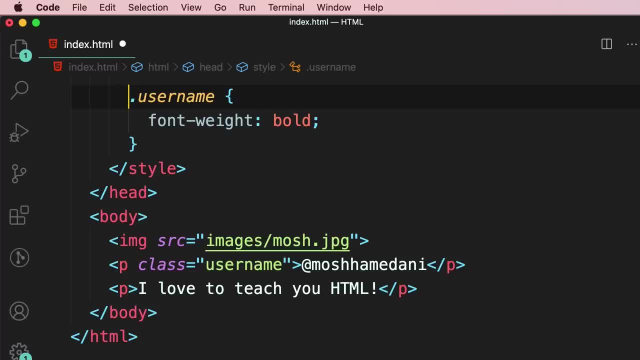 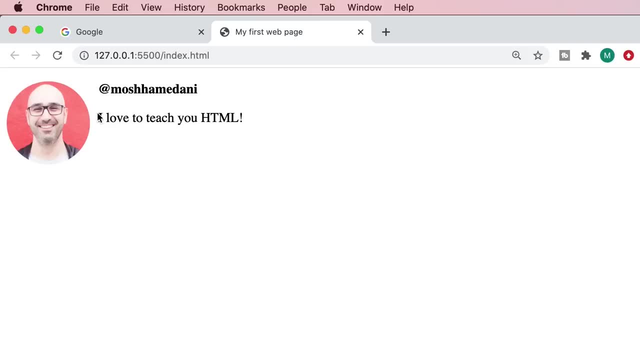 that have the user name class, Whether there are paragraph elements or other types of elements. Now save the changes and take a look. So that's a lot better. So this is CSS in action, As you can see. CSS. 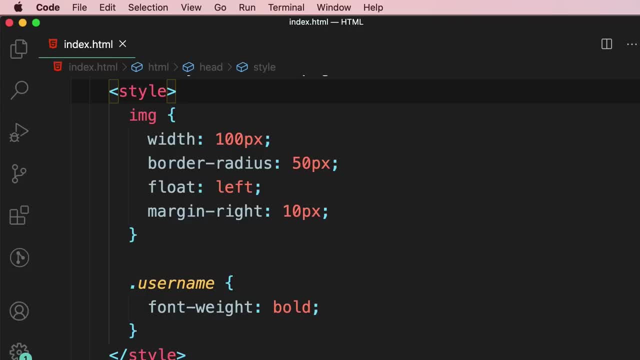 has a different syntax or a different grammar than HTML. Throughout the rest of the course, you're going to learn both these languages in detail. Next, I'm going to show you how to format your code using prettier. Hey guys, Mash here. I just wanted to let you know that. 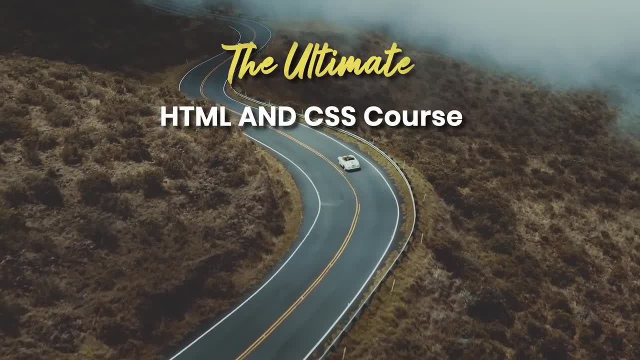 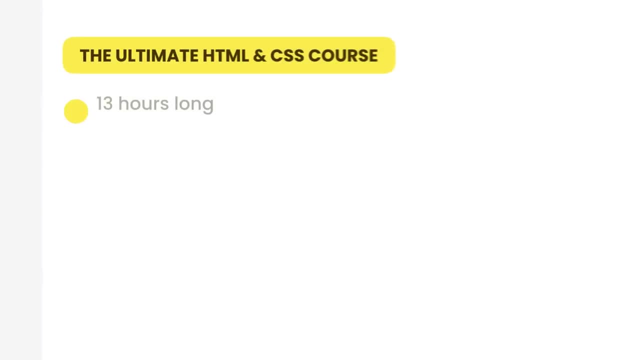 this video you've been watching is the first hour of my ultimate HTML and CSS series. So after you watch this video, if you want to learn more from me, you can enroll in the full course, which is about 13 hours long, and. 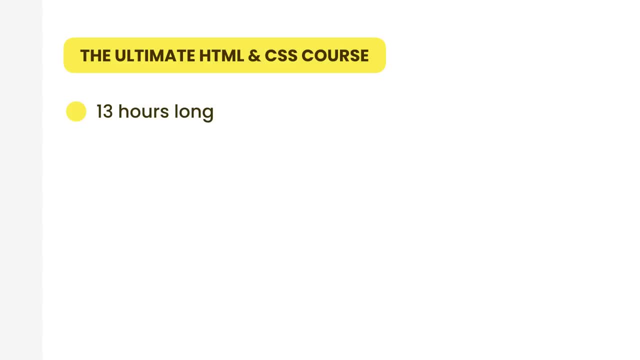 covers everything you need to know to build professional quality websites with HTML and CSS. It also includes summary notes, exercises, a real project, a certificate of completion you can add to your resume and a 30-day money back guarantee to get a refund if you're not satisfied. 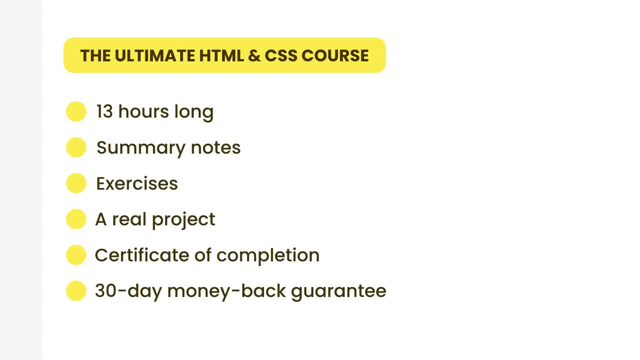 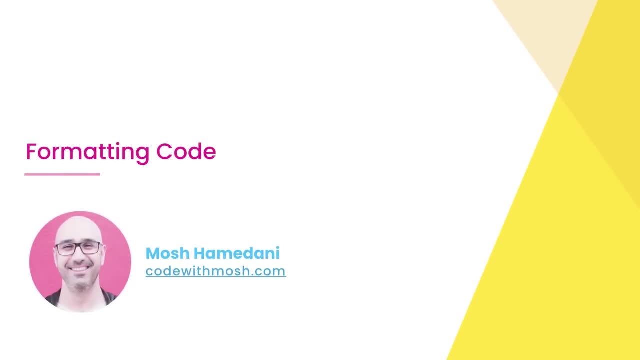 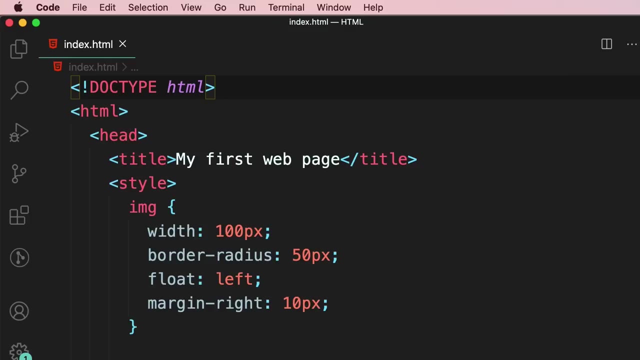 So you have nothing to lose and a lot to learn. So if you're interested, I put the link in the description box: Music, Music. One thing you need to know about browsers is that they ignore white spaces in HTML and CSS code, For example. I can put all these elements on a. 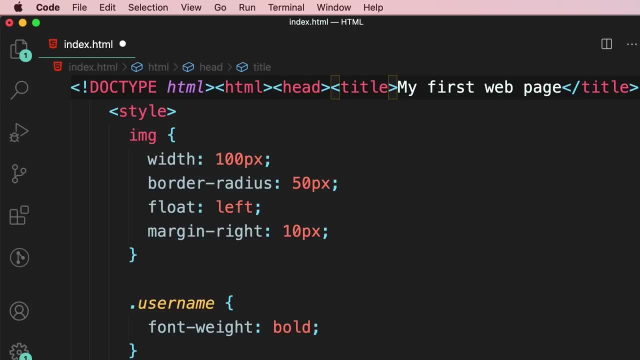 single line and everything still works. Let me show you so. save the changes back in the browser. we have the same result as before, Because browsers don't care how we format our code, But formatting is very important when it comes to reading and maintaining code. 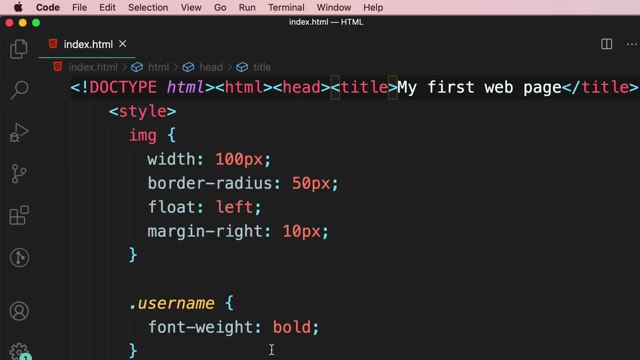 We want our code to be beautiful and perfectly formatted, just like an article. This is where we use the Prettier plugin. With Prettier, we can format our code in a consistent fashion. This is super important when you're part of a team. 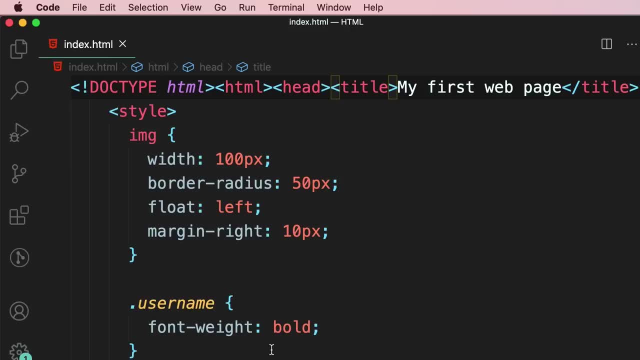 because different people have different ways of formatting their code. but if everyone on the team uses the Prettier plugin, the code will be consistently formatted. So let me show you how to use Prettier. On the top, we go to the view menu. look at the shortcut for the command. 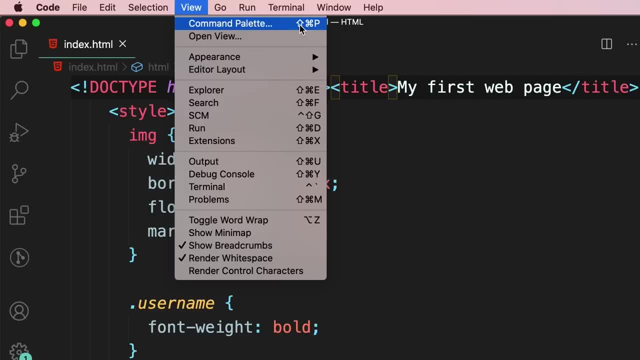 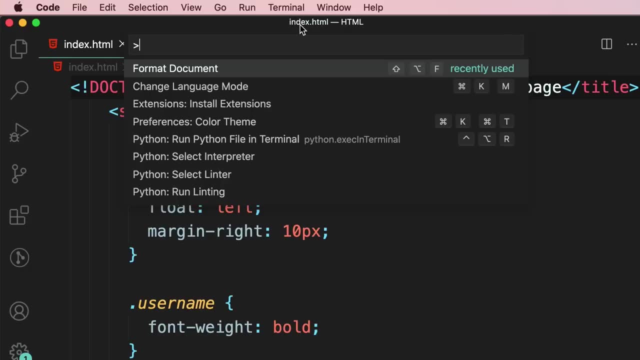 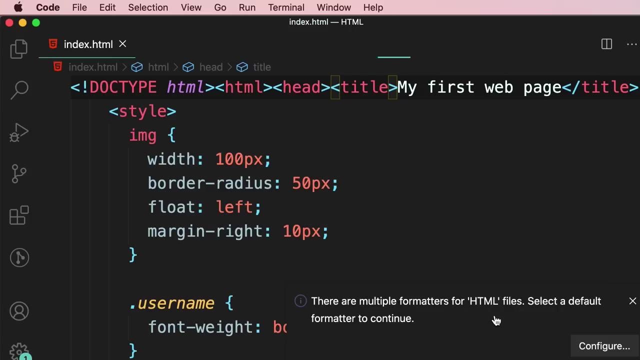 palette. On mac it's shift command and p. on windows it's probably shift control and p. So let's bring up the command palette and here we search for format document. Now we press enter, we get this message saying there are multiple formatters for HTML files. select the default formatter. 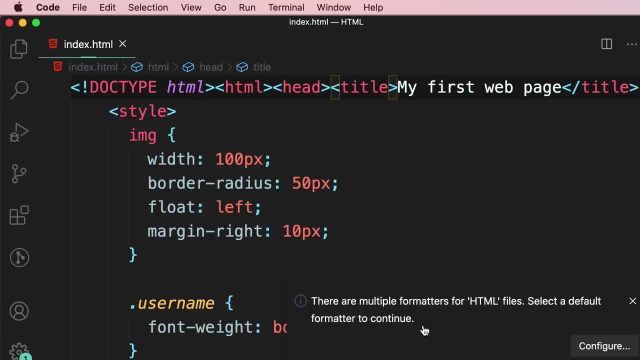 to continue. The reason we're getting this message is that vs code by default comes with a formatter for formatting HTML files, But we have installed Prettier, which is a separate formatter. So let's go to configure and tell vs code to use Prettier. 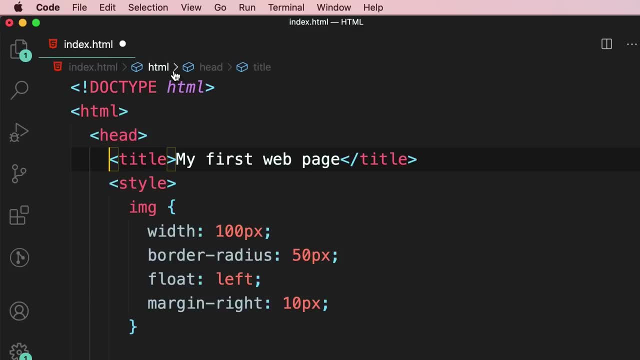 to format HTML and CSS files. Okay, Now, Prettier formatted my code, so none of those elements are on the same line. this is a lot better. But let me show you a trick. We don't want to format our code every time we make a change, So we can. 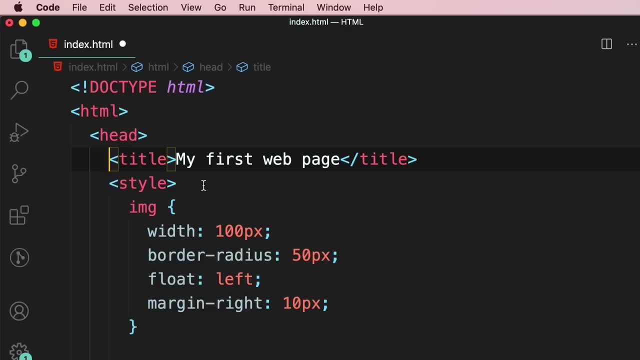 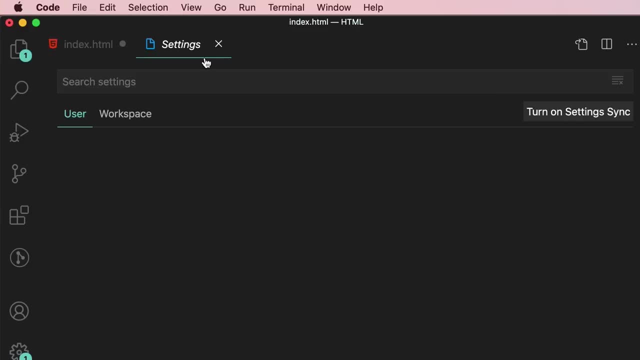 configure vs code to automatically format the code the moment we save the changes. So on the top let's go to the code menu, then preferences and settings And here search for format and save. Here's the setting. let's enable the setting now, every time we save. 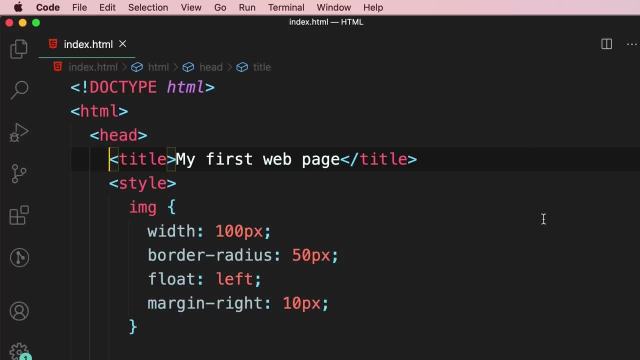 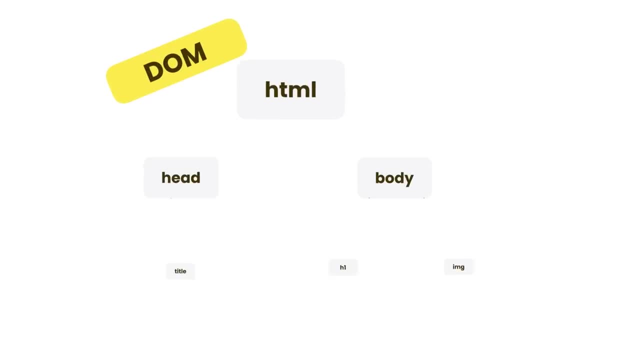 the changes vs code automatically formats our code using Prettier. Earlier we talked about the DOM, or document object model. I told you that when the browser reads the HTML document that is returned from the server, it constructs a document object model. Now let me show you this document object model in action. So once again we're going to. 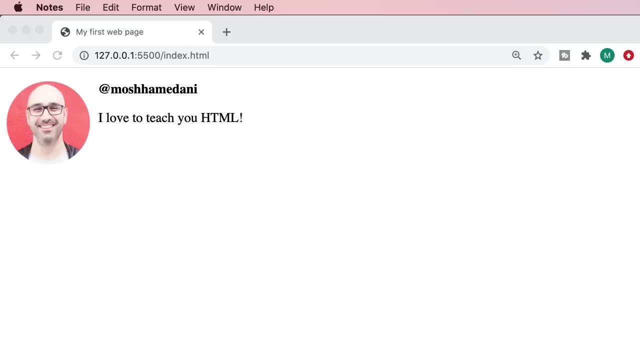 use chrome dev tools. The shortcut on mac is shift command and i on windows is probably shift control and i I'm not really sure. So let's open up dev tools now. in this lesson we're going to look at the elements tab. Now what we have here: 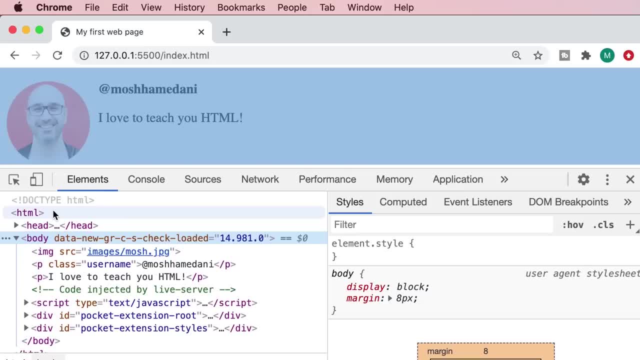 on the left side is our document object model, So we see the same elements that we created earlier in the course. We have the HTML element, head body and so on. But we have some additional elements that are injected by live server. For example, we have the script element and two divs. 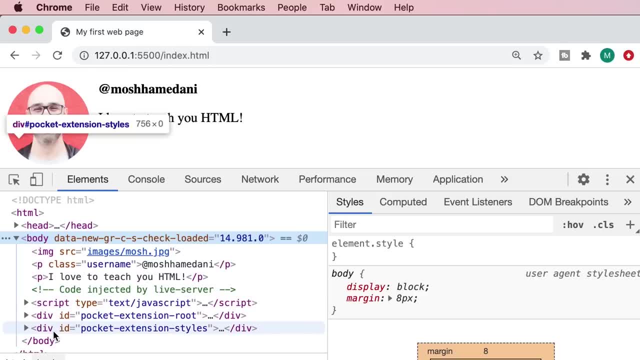 Don't worry about these. these are purely used by live server, so it automatically reloads our page. Now we can hover over any of these elements and you can see that element highlighted here. Now we can click an element and on the 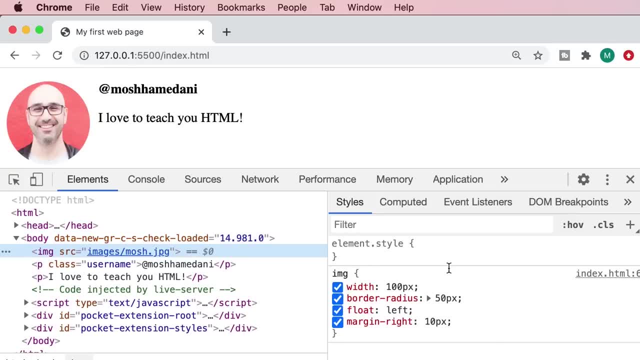 right side, we can see the styles applied to this element. So look at the styles we defined for the image element: width, border radius and so on. We can enable or disable these styles. so we can disable the width property and now our image is big, We can bring it back. 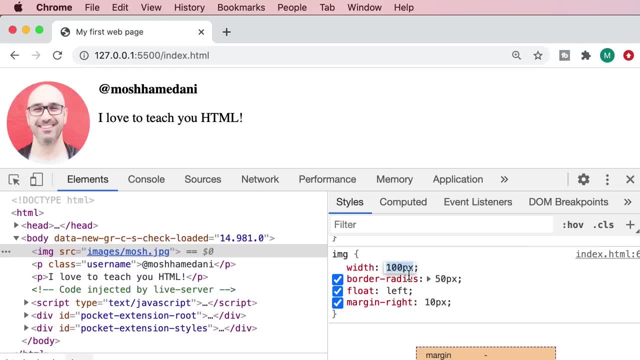 we can also change its value, so we can set it to, let's say, 50px. now our image is smaller. we can use the up and down arrows to change this value. this is pretty handy, so a lot of front end developers. 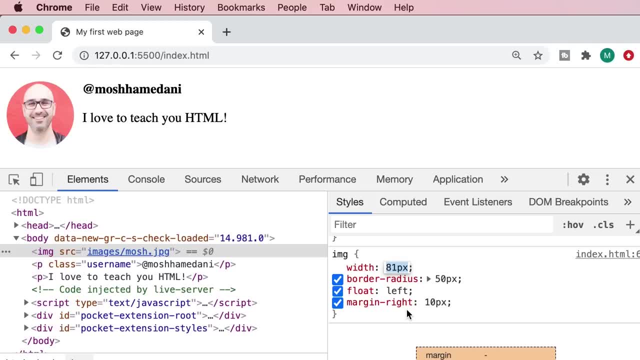 use dev tools to play with these styles and get the look they want. Once they figure out the exact styles and their values, then they apply them in the code. Now one more thing: over here we can see where these styles have been applied. So in indexhtml: 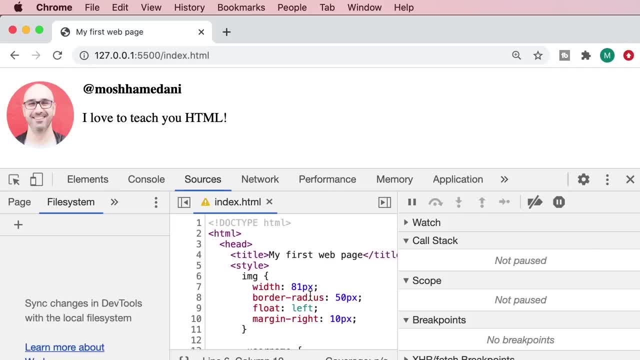 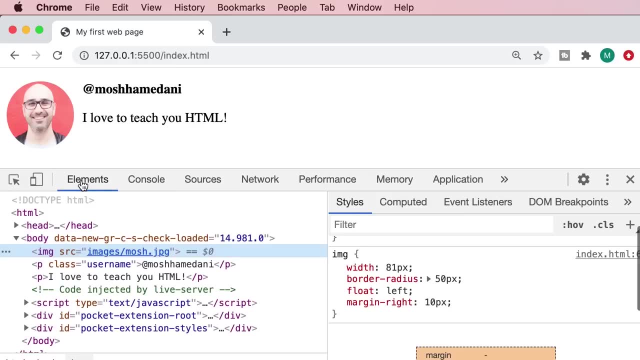 on line 6, we can click on this link and this takes us to the exact line of code where we wrote that style. Now we are currently on the sources tab, so we can go back to elements and inspect other elements. So this is the basics of inspecting elements. 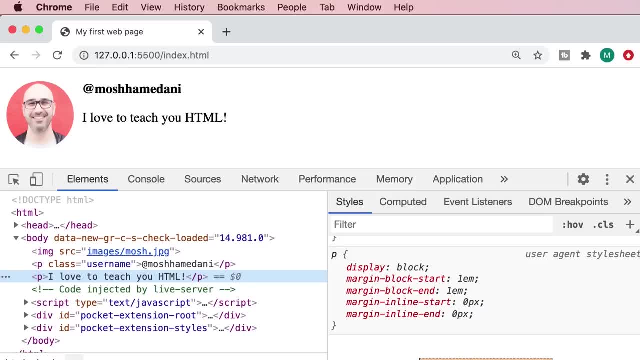 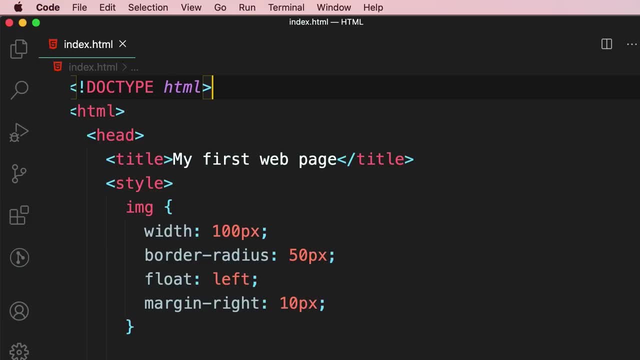 using dev tools. we're going to talk about this in more detail in the future. The last thing we're going to cover in this section is validation. So as we write code, we may run into problems If you have a typo in our code or don't use the right syntax or grammar. 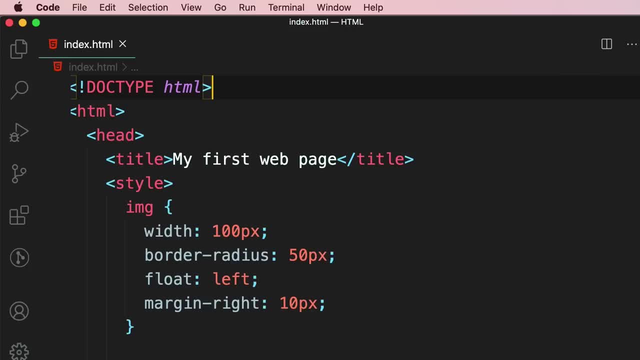 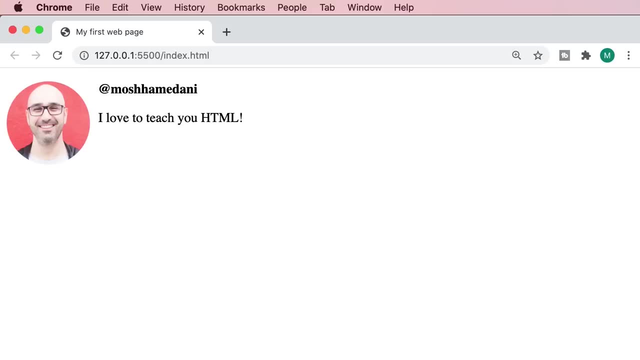 our web pages may not look as expected. In this situation, we can use a validator to identify the potential errors in our code. Now, currently, we don't have any problems on this web page. it looks perfectly fine to me. but let's run it by the standard html validator. 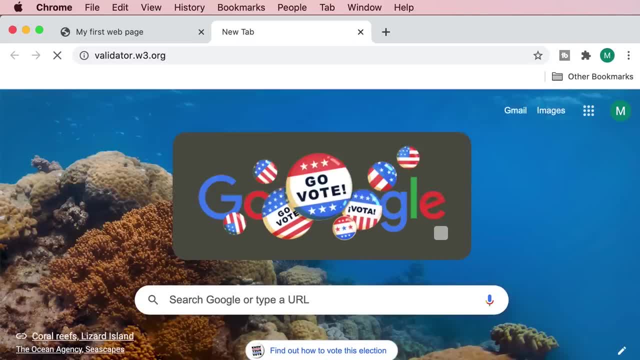 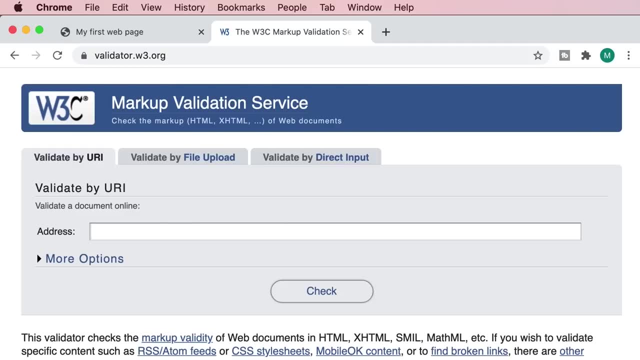 So we go to validatorw3.org. this is a standard markup validation service. we have three methods for validating our html markup. We can validate by an address if our website is livev3.org, But this doesn't work for us because our website is currently. 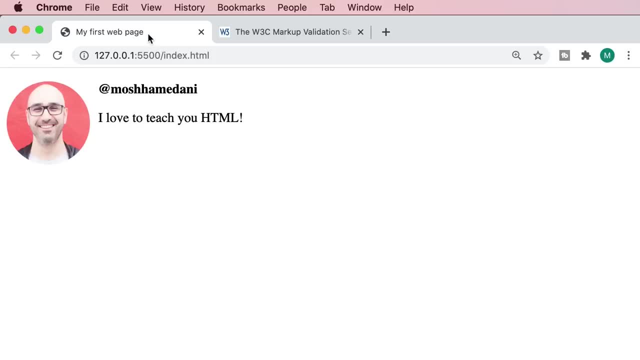 hosted locally in our development server. So this IP address that we have over here- 127.0.0.1,. this is a local IP address, so no one else can access our website. So here we have two other methods we can validate. 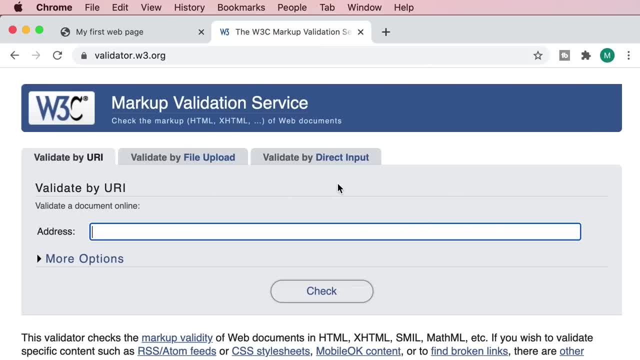 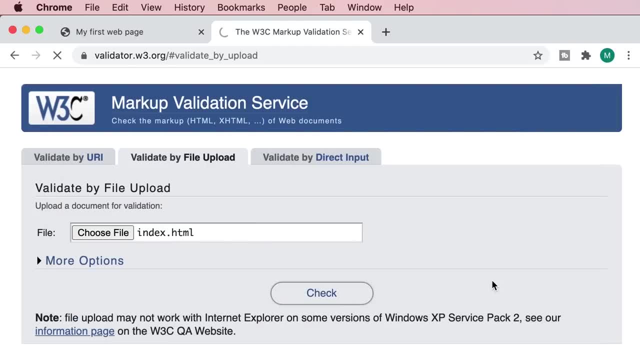 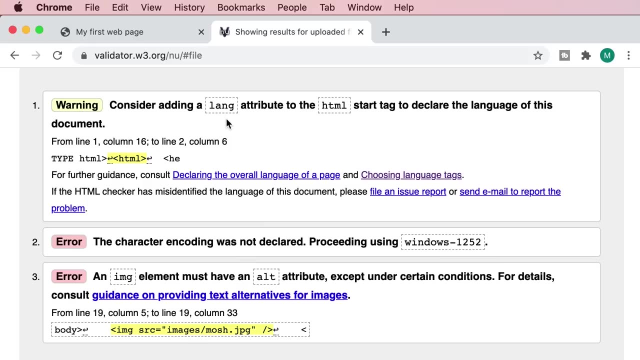 by file upload or by direct input. In this case, I'm going to go with file upload. so let's upload our indexhtml file And check. so look, we have one warning and two errors. The warning is saying that we haven't added the lang or 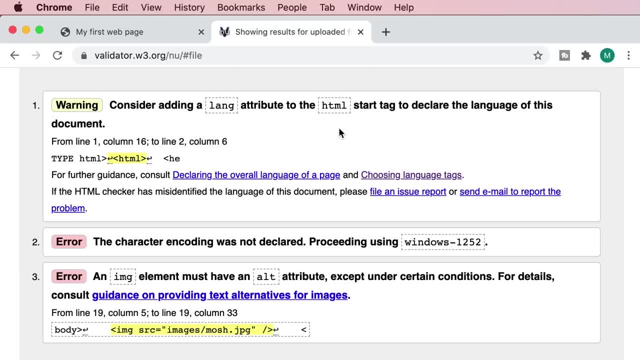 language attribute to the html start tag. This is a common best practice because with this we can tell search engines what is the language of this web page, So they can do a better job at displaying the results. This is very easy to fix, so here's our html tag. 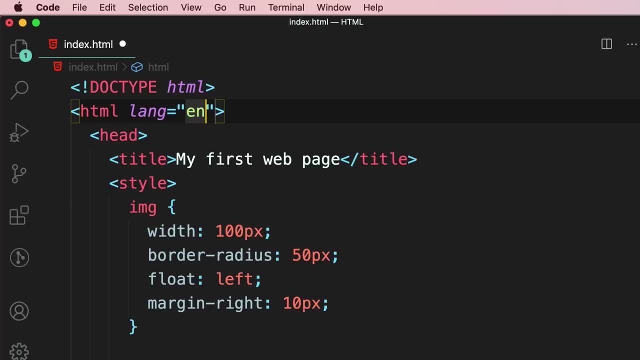 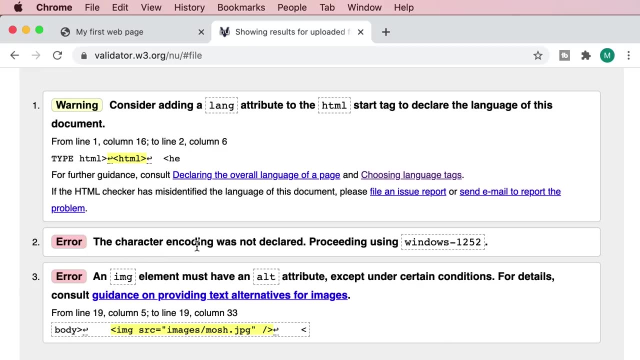 we're going to add the lang attribute and set it to en, which is short for English. Now what is next? We have an error saying the character encoding was not declared. Don't worry about this. we'll talk about this in the next section. So let's look at the second. 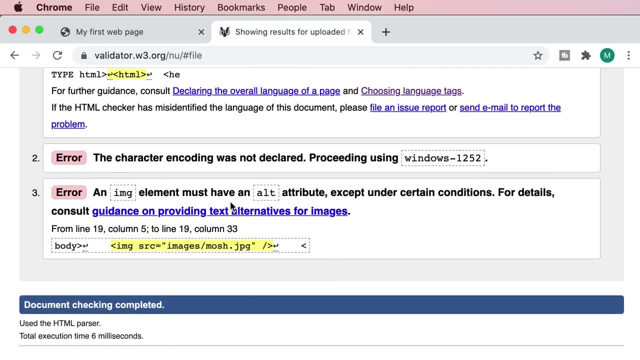 error. It's saying that an image element must have an alt attribute. So earlier we had this alt attribute. I told you that use the alt attribute to provide a description for our image. So if the image cannot be displayed, the alternative text will be displayed. 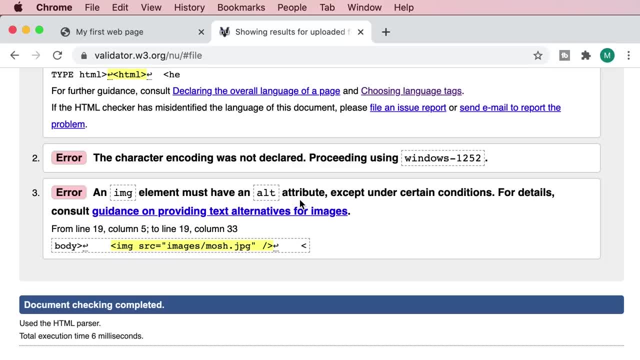 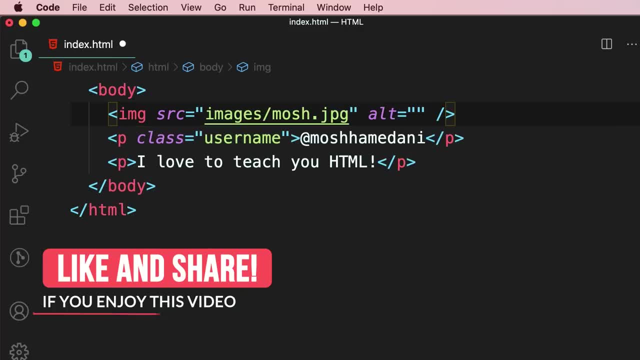 Again, we're going to talk about the alt attribute in more detail in the future. So back to our code. let's fix this error real quick. Here's our image tag. let's add the alt attribute and for the description, I'm going to say an image of mosh hamadani. 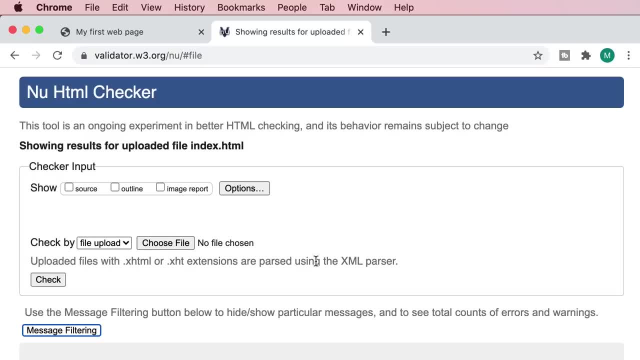 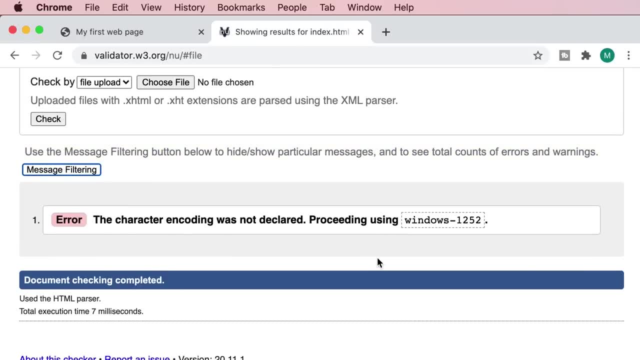 Now save the changes. let's reupload the file and validate it one more time. Okay, this time we have only a single error, and that has to do with character encoding, which we're going to talk about later. So this is all about HTML validation. 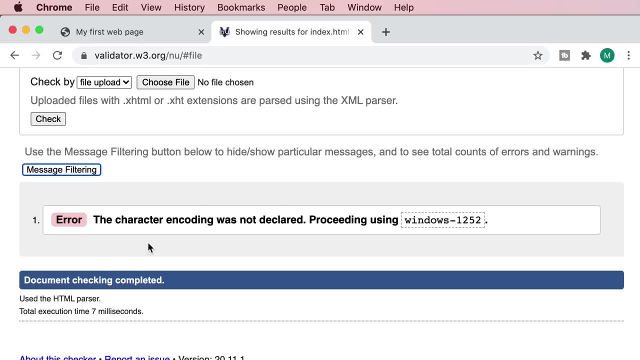 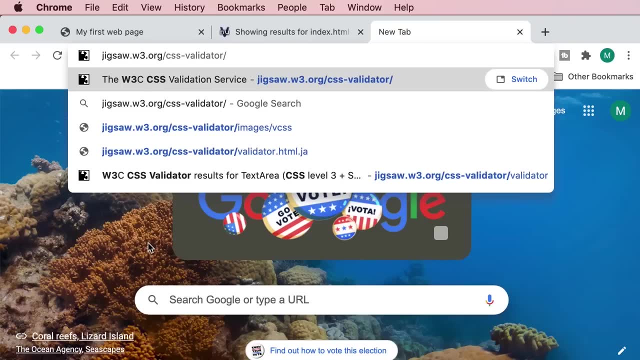 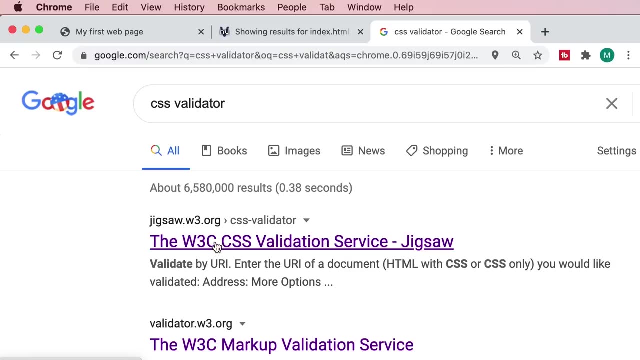 Now for CSS. we have a different validator. So we go to jigsaww3.org: slash css-validator. Now you don't have to memorize this address. simply go to google and search for css validator. Here's the first link. So we have the same interface. 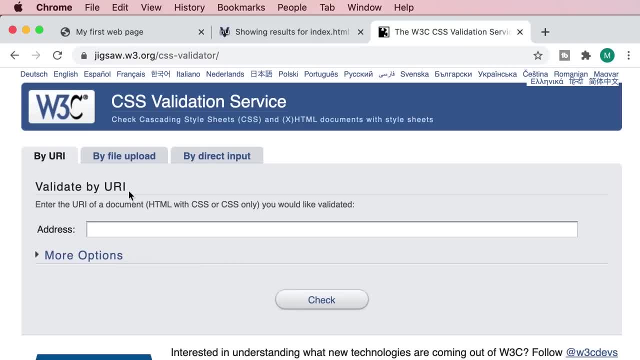 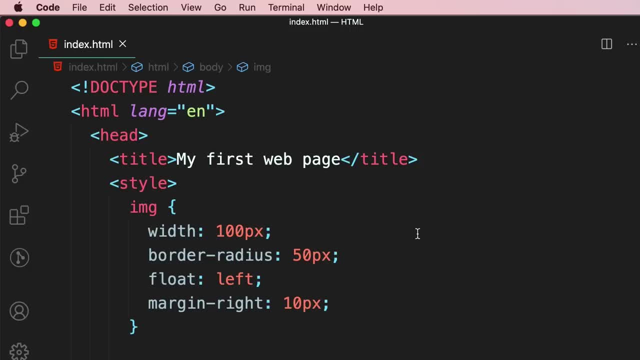 we can validate our css code using an address, or by file upload or direct input. Now, in this case, we have embedded all of our css code inside our html markup, But as our webpages get more complex, we want to separate our css code. 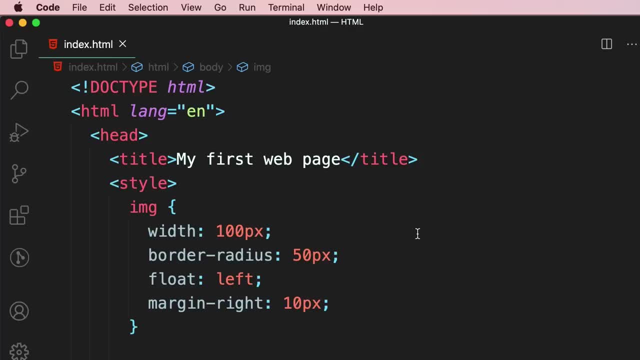 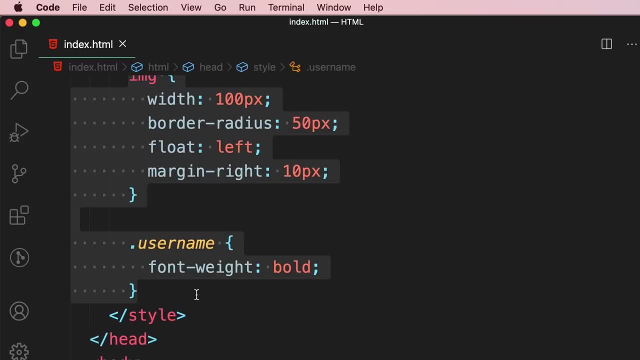 into separate files, so our code is better organized. We'll talk about this in more detail in the future, So for now I'm going to copy all of our css code and then go to the third tab, paste it over here and validate it. 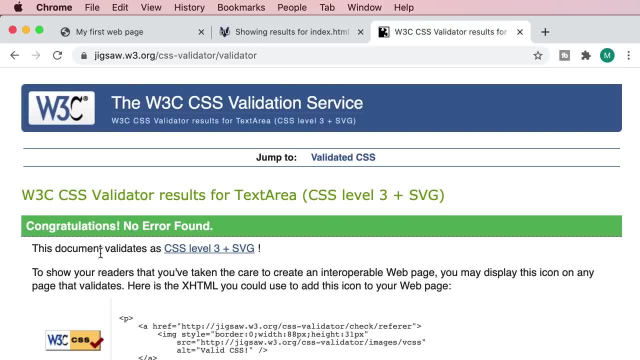 So we don't have any errors. everything is perfect. So this is all about validation. Validation is very important. if your webpages aren't displayed as expected, always start with a quick validation, because this can often point you in the right direction. Alright, that brings us to the end of this section. 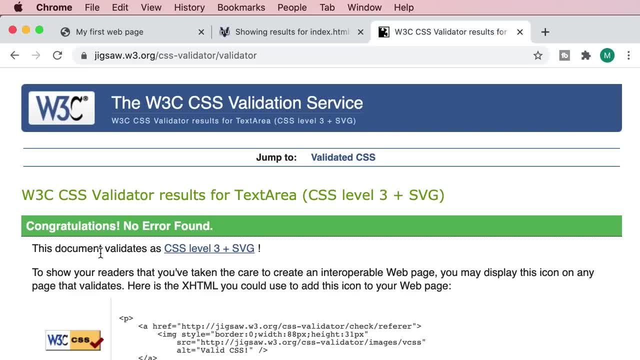 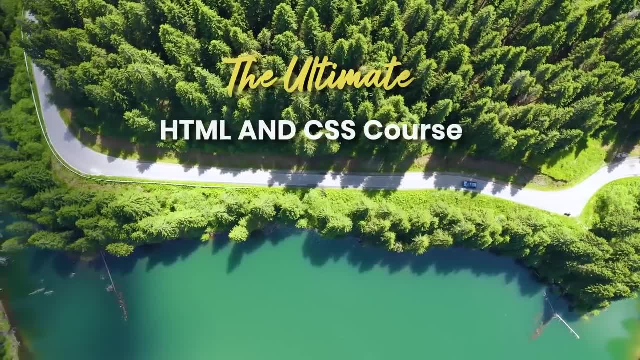 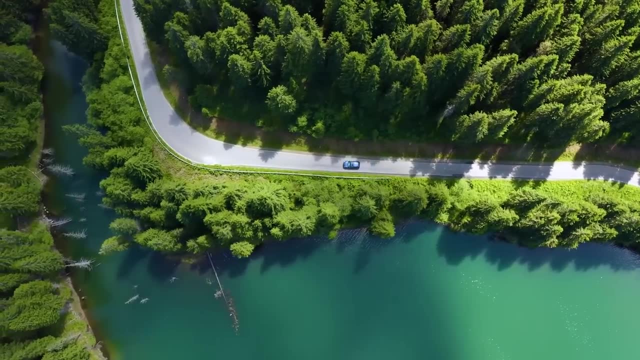 In the next section we're going to explore HTML in more detail. We're going to continue our web development journey and explore HTML in more detail. So in this section we're going to cover the essential HTML elements you need to know to build webpages. 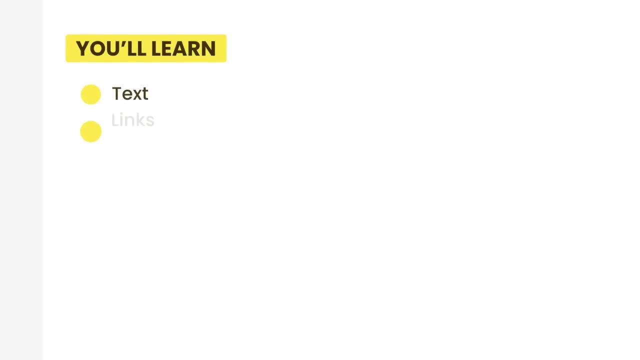 You will learn all the elements used for displaying text, links, images, lists, tables, as well as container and structural or semantic elements. Even if you know the basics of HTML, I would still encourage you to watch this section thoroughly, because a lot of people don't use these elements the right way. So let's jump in. 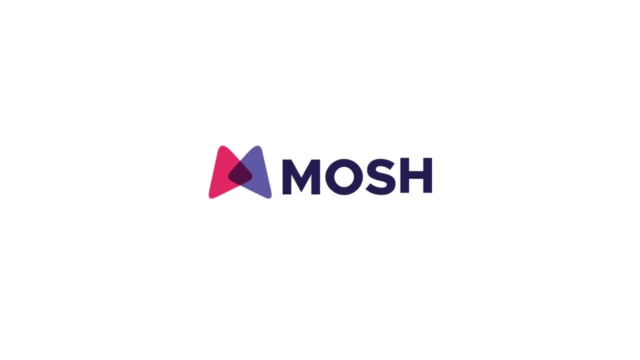 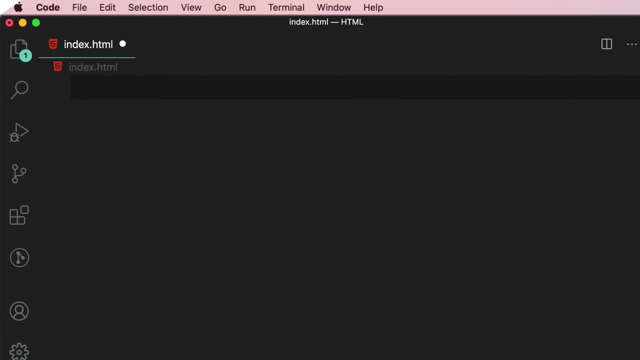 and get started. Earlier in the course, I told you that we use the head section to give browsers and search engines information about a web page, So let's explore it in a bit more detail. I'm going to start with a blank document. 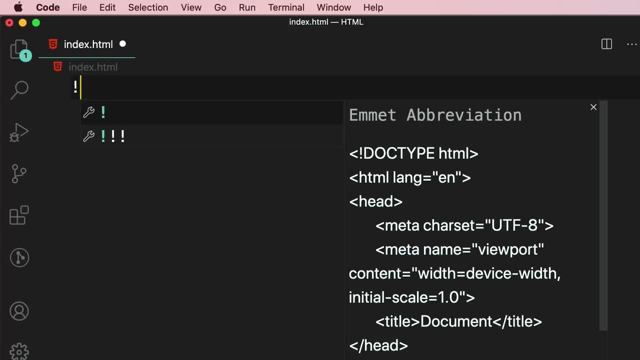 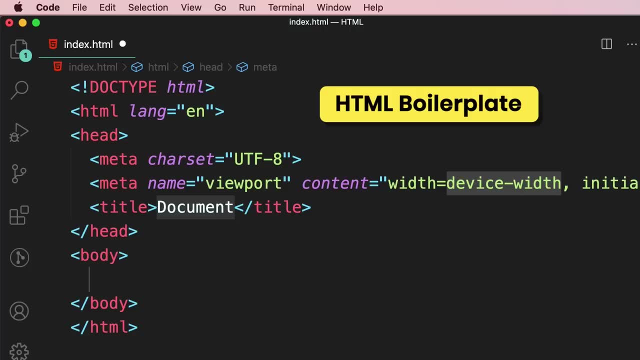 now let me show you a cool trick. If you type an exclamation mark and then press tab, we get a basic HTML boilerplate, which means a basic HTML template. So on the top we have our doc type declaration, below that we have our HTML element. 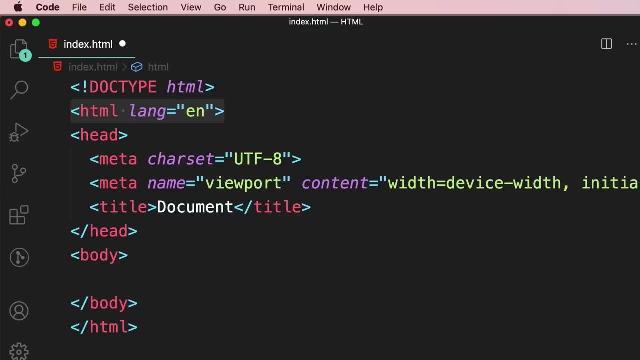 with the lang attribute, which is a common best practice. Next, we have our head section, with a bunch of elements we're going to talk about in a second, followed by the body section. So this is a very basic HTML boilerplate. Now, what do we have in the head section? Well, 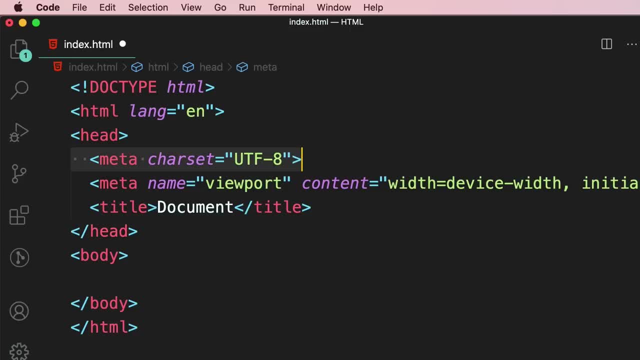 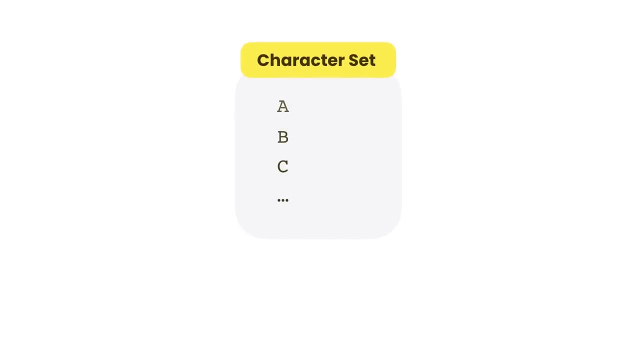 we have a couple of meta elements for giving information about this web page. The first meta element is for defining the character set. What is a character set? Well, computers don't understand characters like ABC and so on. They only understand numbers which are represented. 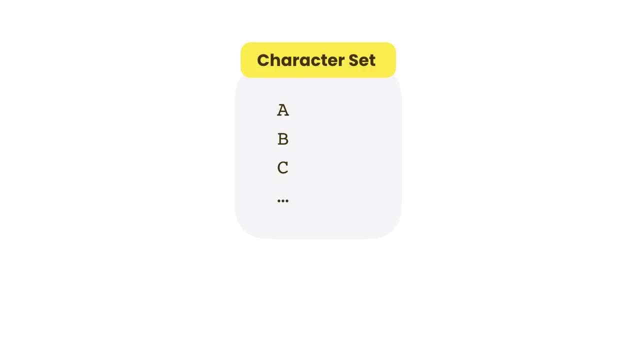 in the binary format zeros and ones. So using a character set we can map a character to a numeric value. The first character set that was designed was the ASCII character set, which is short for American Standard Code for Information Interchange. ASCII can only represent the characters in the English language. 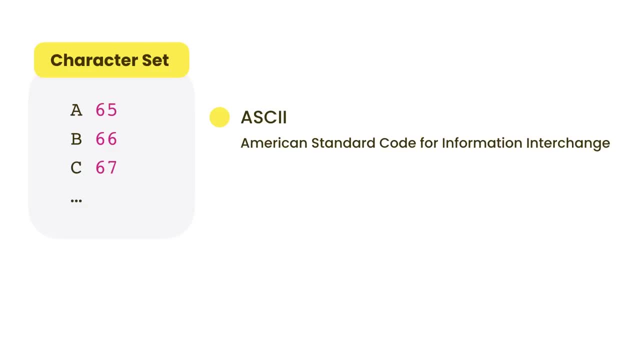 So it's very limited. So over here, different character sets have been created to represent more characters in international languages. The character set that we use most of the time these days is UTF-8,, which can represent almost all characters in the world. 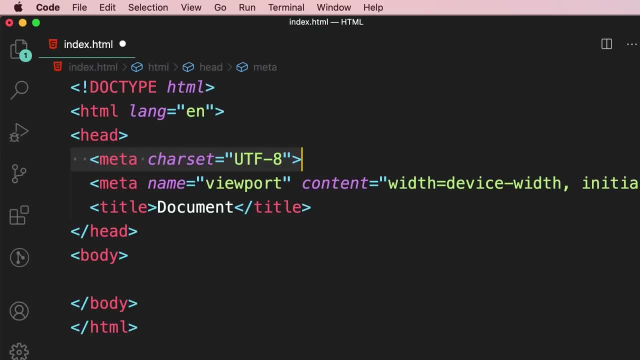 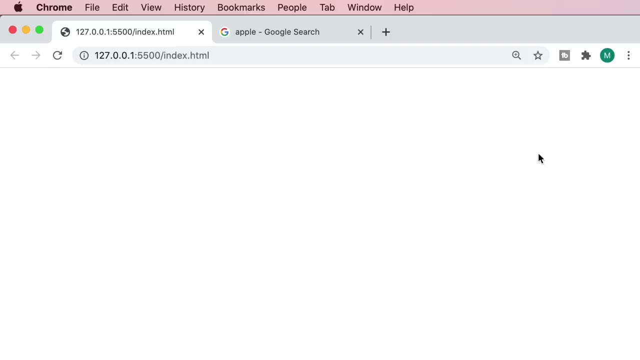 So back to our code. with this meta element, we're defining the character set used in this HTML document. Now, below that, we have a meta element for configuring the viewport. The viewport is the visible area of a web page, So it is this area over here, Obviously on a mobile device. 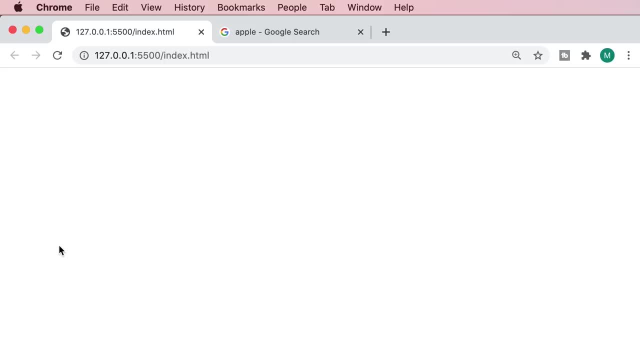 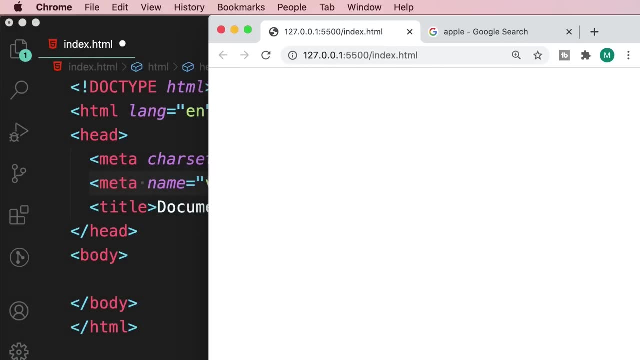 or on a tablet, our viewport is smaller. But here on desktop, we can change the size of the viewport by resizing the browser. So now our viewport is smaller. Now back to our code. With this element we're defining the initial width. 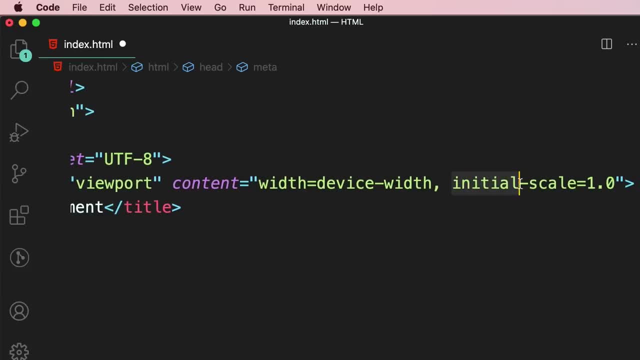 and zero The zoom factor for the viewport. We'll talk about this in more detail in the future. For now, all I want you to know is that we need this element so our web pages look good on all devices- mobiles, tablets. 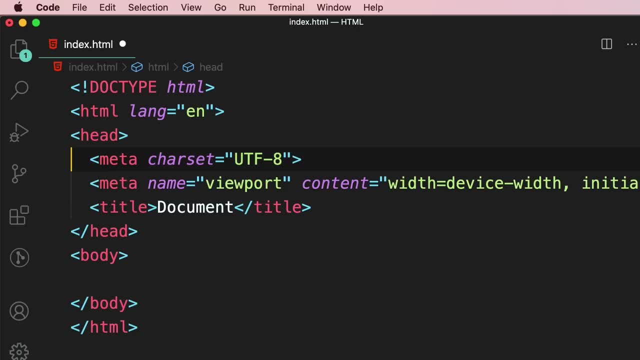 and desktop computers. So as a best practice, every web page should have at least these two meta elements. But we have additional meta elements. Let me show you. So if you type meta in this list, you can see all possible meta elements. For example: 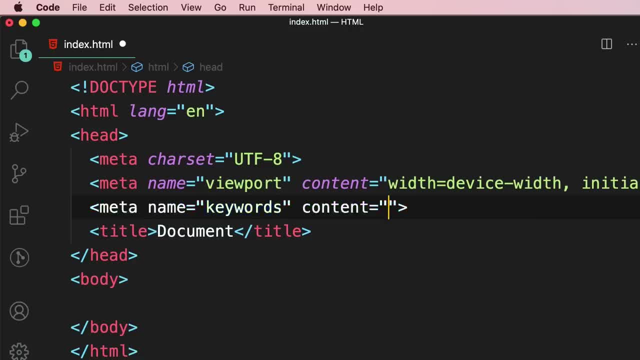 we have this element for defining keywords on a web page, So let's select this. Here we can type multiple keywords like HTML, comma, CSS and so on. In the past, these keywords were heavily used for search engine optimization, but these days, most 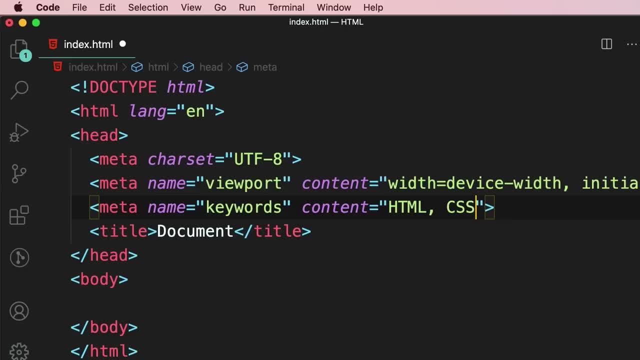 search engines don't put too much weight on these keywords, But we can still use them to define the keywords that represent this page. We have another meta element for defining a description for this page. So if you type meta colon, desk, and then press tab or enter, 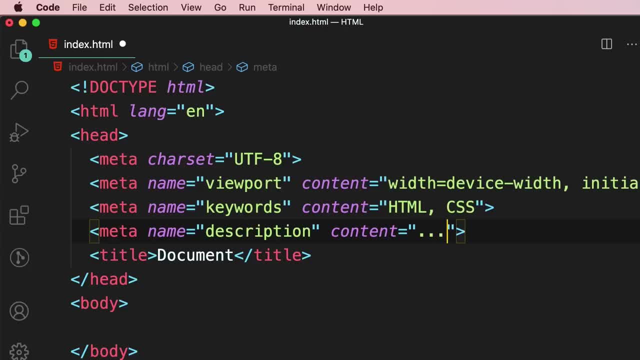 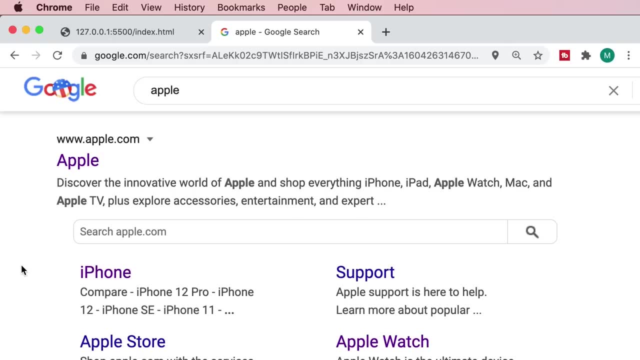 here we can type a description for this page. What we type here will appear on Google or other search engines when someone searches for a website. For example, if we search for apple, here's what we get. Now look at this text. What you see here. 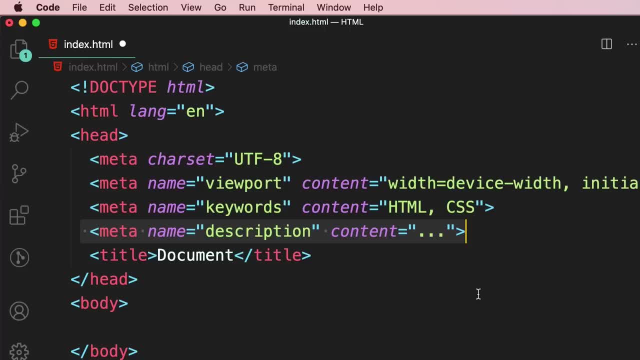 comes from this element over here. So this is the purpose of meta elements. With this meta element, we can give information about a web page, Alright. next we're going to talk about data, The elements you need to know for working with text. 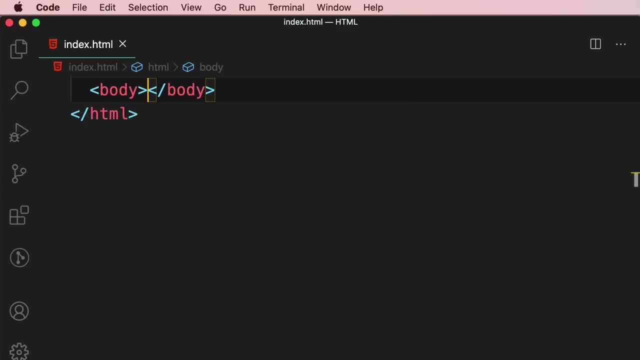 Alright, now let's talk about the most common elements for working with text. So you learn about the p or paragraph element which we use for displaying some text. So here I'm going to say I love to teach you HTML. Now, sometimes we want to emphasize. 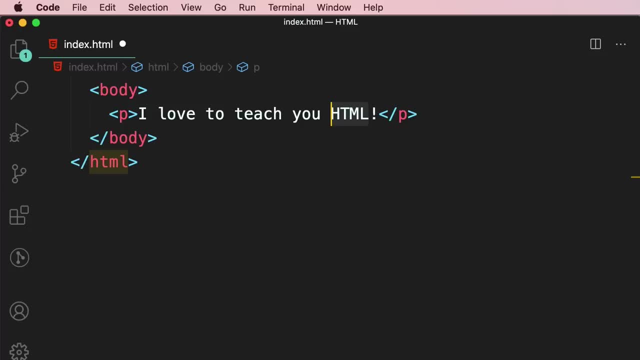 a part of our text. Let's say the HTML word here. To do that, we can wrap it inside an m or emphasis element. So here I type m, press tab. here's the emphasis element. let's hover over it and see what the tooltip says. It says: 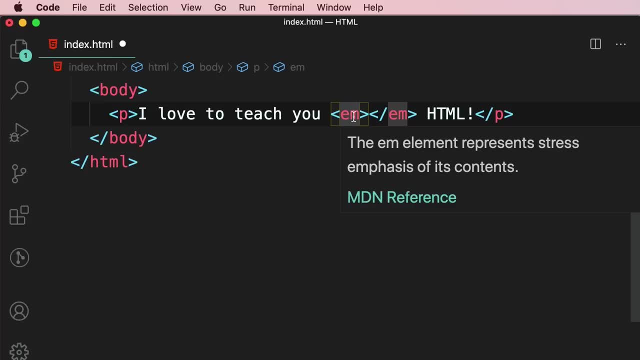 the m element represents stress, emphasis of its content. So whenever we want to emphasize some content, we can wrap it inside the m element. So in this case I'm going to move HTML inside these tags. Now let's save the changes. 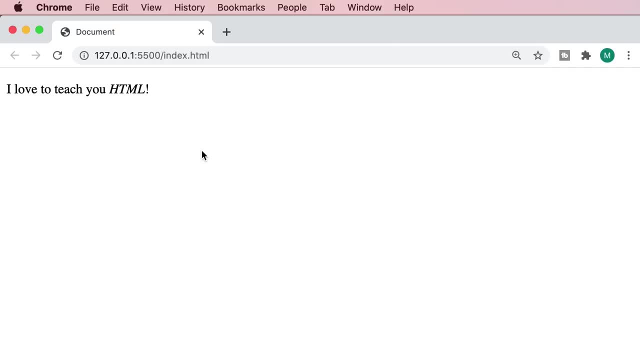 here's what we get. So, by default, browsers display emphasized content in italic, But don't assume that whenever you want to display italic content, you should use the m element, Because the purpose of the m element is to emphasize content in our HTML document. 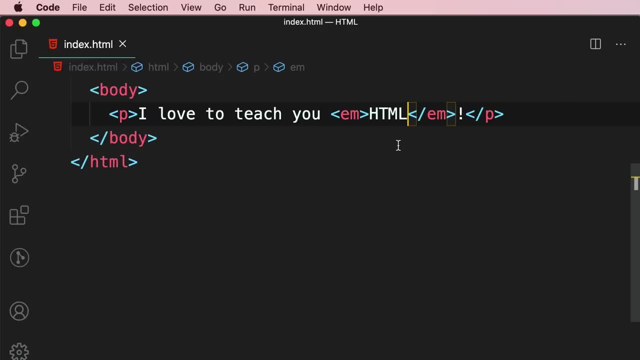 And this helps search engines extract important content in our documents. Anything to do with styling should be done in CSS. For example, here we can change the default style of emphasized elements and remove the italic. Let me show you So. here we can change the default style of emphasized elements and remove the italic. Let me show you. 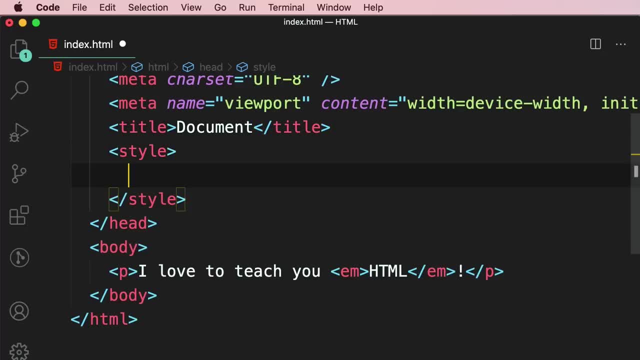 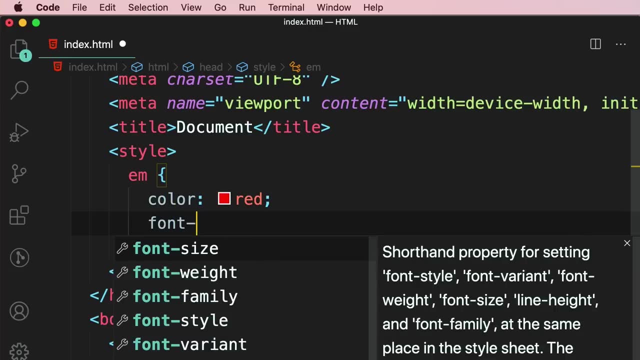 So in the head section we add the style element and here we define a rule for emphasized content. We can set the color to red and font style to normal. Now don't worry about memorizing any of these CSS properties. we're going to go over. 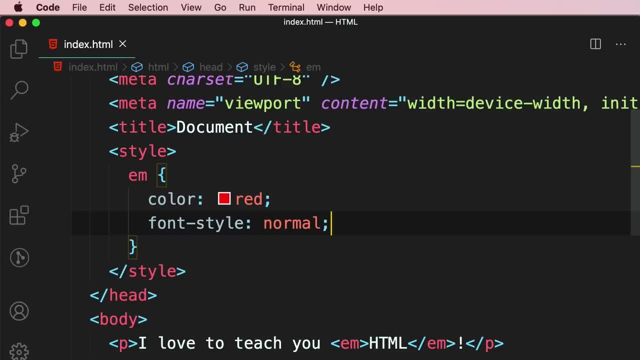 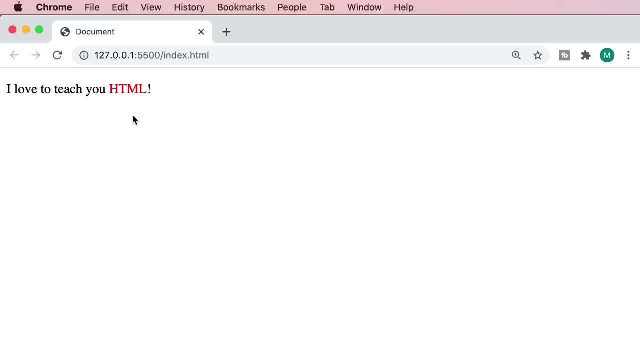 them multiple times throughout the course. But let's see what happens now that we apply these styles. So our emphasized content is displayed in red and is no longer italic Now, in the past, we had an element called i, which was short for italic. 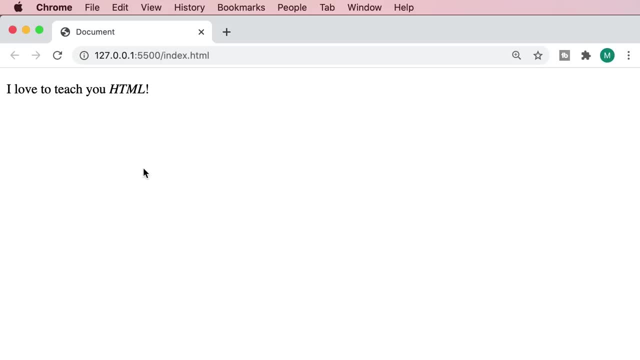 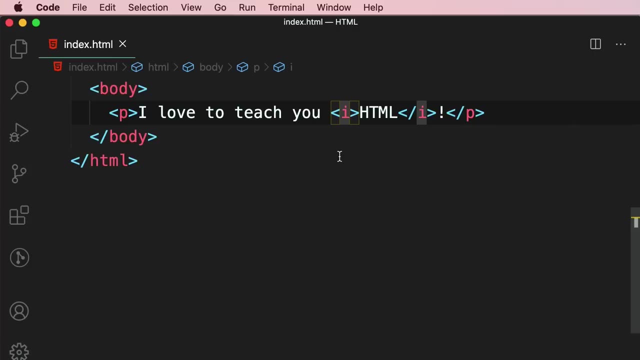 If we use this element, we get the same result as before. Our content is displayed in italic, But this element is considered deprecated because HTML is not meant for styling. It should only be used for structuring content. So don't use the i element to display content as italic. 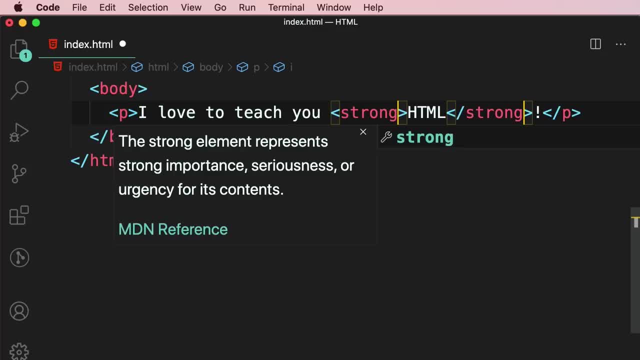 Now we have a similar element in HTML called strong. Let's hover over it and see what the tooltip says. The strong element represents strong importance, seriousness or urgency of its contents. Conceptually it's kind of similar to the emphasis element. so where you should use it really depends on your context. 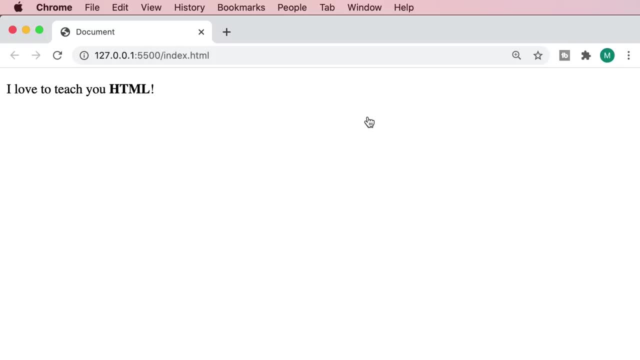 on your content. Now let's save the changes and see what we get. So by default, strong elements are displayed as bold, But once again, we can always change the styling Now. in the past we had another element called b, which is short for bold. 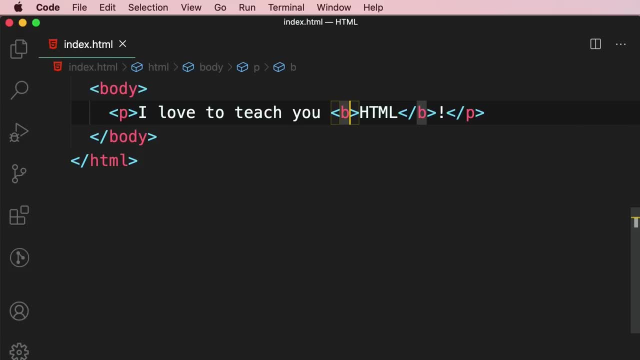 So whenever we wanted to make something bold, we use this element. But once again this element is considered deprecated because styling should be done in CSS and not in HTML. So don't use b or i elements. Now I'm going to remove this element. 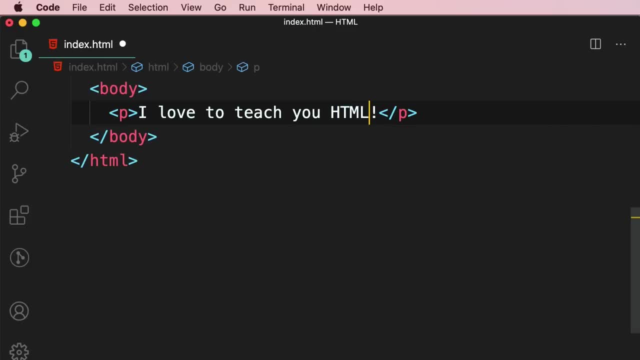 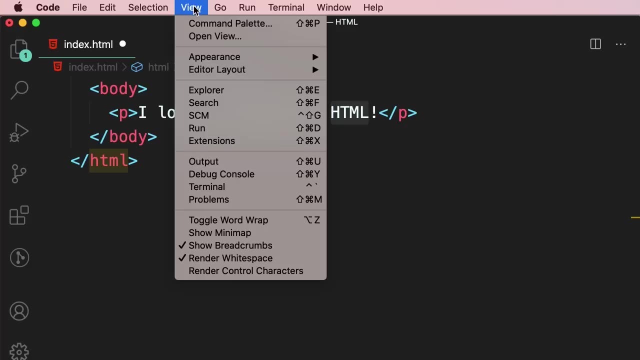 and just add HTML. Let me show you a cool trick. Let's say we want to wrap this word with the m element. There is a shortcut for it. So on the top we go to the view menu. look at the shortcut for the command palette. On Mac it's shift command and p. 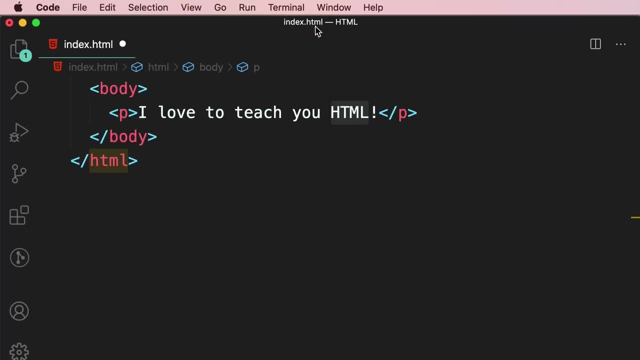 and on Windows it's probably shift, control and p. So let's select HTML and then bring up the command palette. With this command palette we can execute commands in VS code. So here I'm going to search for a command called wrap, with abbreviation. That is the first command on the list. 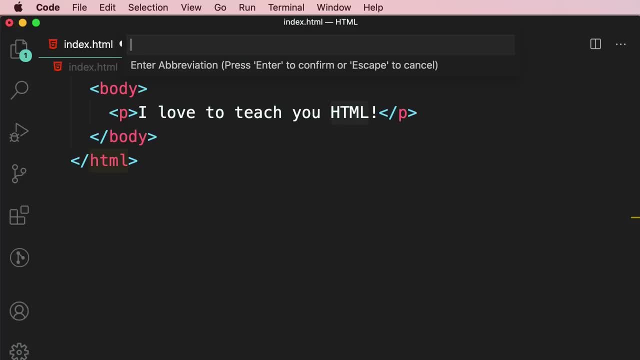 Now we press enter and here we type the element that we want to use to wrap our selected content, In this case m. Press enter. done So I didn't have to manually create an m element and then move HTML inside it. It's very handy. 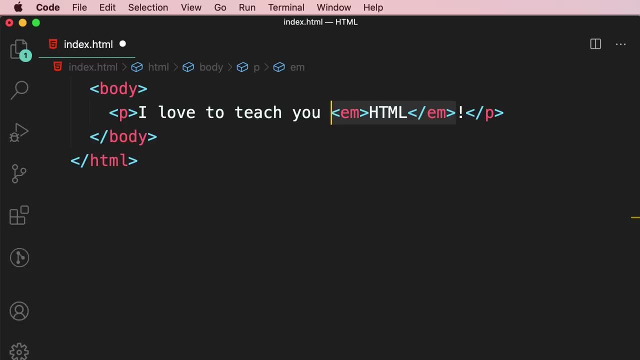 So this is all about text. now let's talk about headings. So in HTML we have 6 heading elements: h1, we have h2, h3, h4, h5, and h6.. So let's see what we get. So 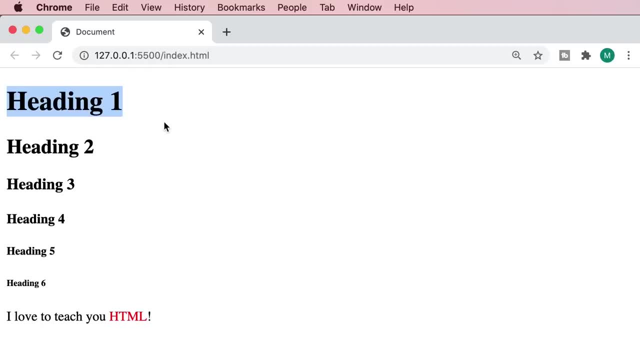 heading 1 represents the most important heading and heading 6 represents the least important heading. Now, one common mistake that I see amongst a lot of people is that they choose these headings based on their size. So if they want to have a heading with this size, 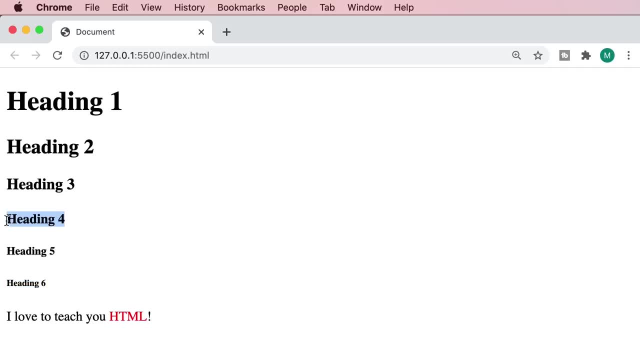 they would just use heading 4.. That is not how you're supposed to use headings, Because the size can always be changed with CSS. It's a matter of styling. We should use these headings to create a hierarchy, So every webpage should have one and only one h1 element. 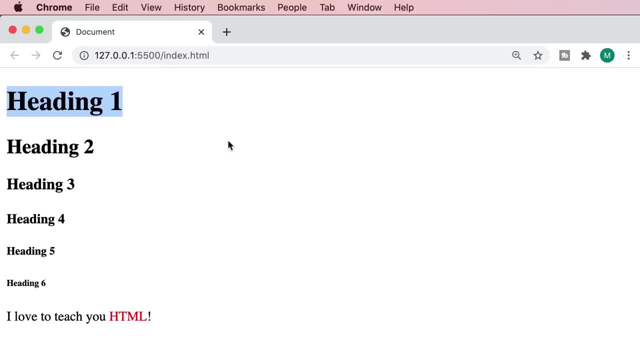 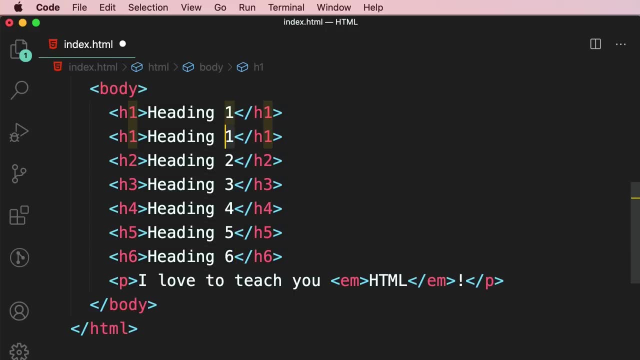 This heading represents what this page is all about. Now, nothing happens if you have multiple h1 elements. for example, I can duplicate this line and say heading 1 plus. Now, look, we have two h1 elements, but this is going to confuse search engines. 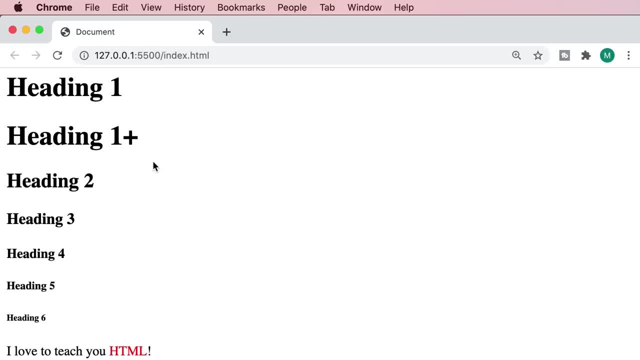 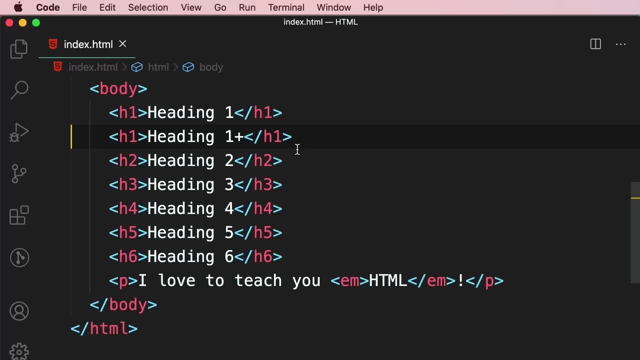 They're not going to figure out what this page is really all about. So every page should have a single h1 element. So I'm going to remove this line now. after we use h1, then we should use h2,, we should not jump to h4.. 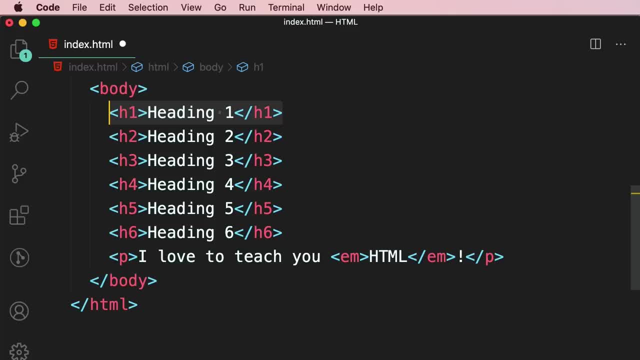 So let's say, on this page we're going to have two sections, one for html, the other for CSS. So my next heading should be h2, and here we can type html. obviously, below this heading we can have some text. so I'm going to say html. 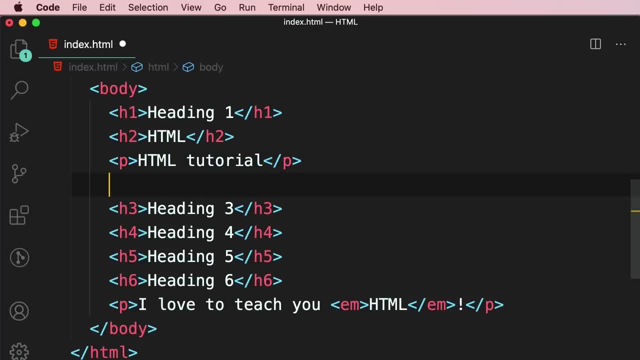 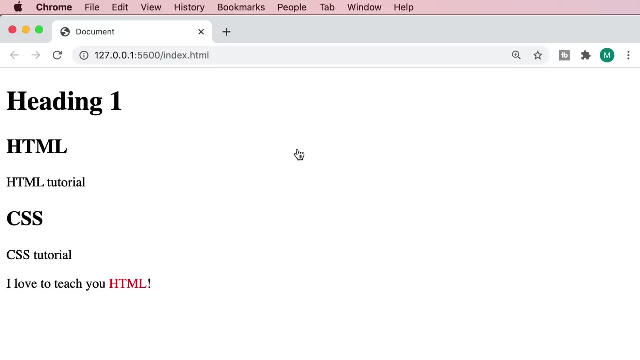 tutorial. Our next heading should be h2.. So this is the CSS section, and in this section we can have some additional text. let's say CSS tutorial. Now I'm going to delete these four headings, so let's take a look. so we have a hierarchy. 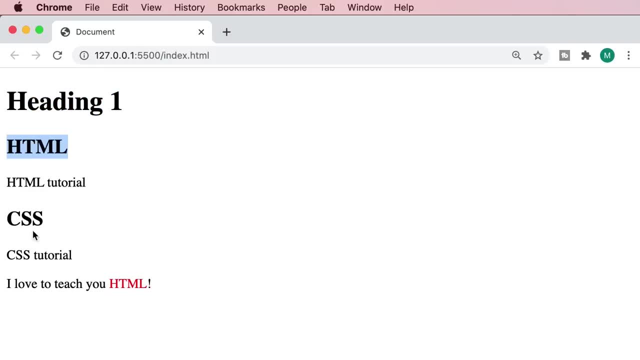 On the top we have an h1 element. below that we have two h2 elements. Now let's say, in this section we have two h1 elements. we're going to have two subsections there. we should use h3 elements. So here's our html section. 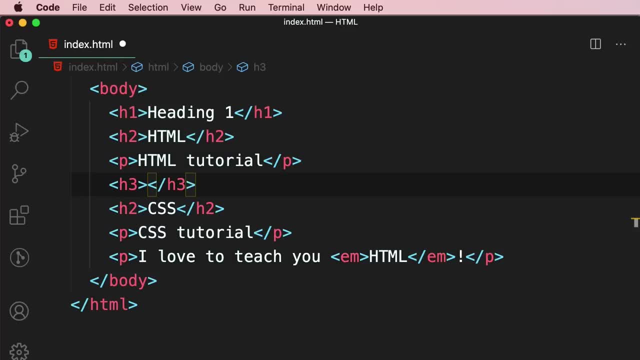 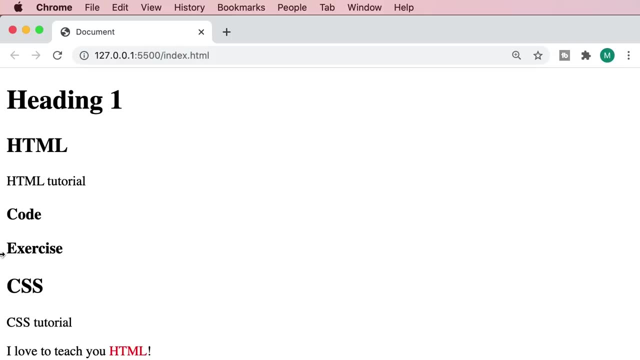 in this section we're going to have two h3 elements. let's say code and exercise. Now take a look. So we have a hierarchy. this is how we should use these heading elements, the better we can represent the structure of our document. 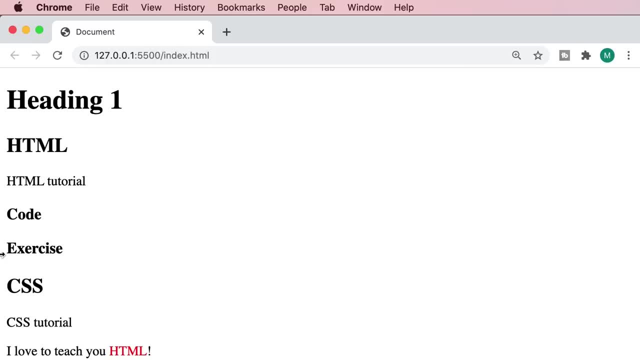 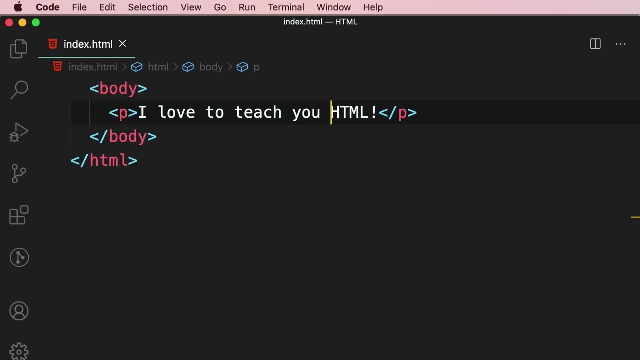 using html, the better search engines can read and understand our content. So that's all about text. next we're going to talk about displaying special characters in html. Some characters are reserved in html and to display them we have to use a special notation. For example: 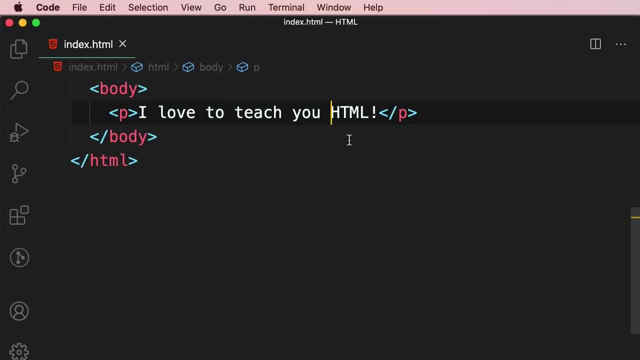 let's say we want to wrap the word html with angle brackets. see what's going to happen. So I type a left angle bracket and a right angle bracket. see what happened. Vscode thought we're adding an html element, so it automatically generated the closing tag. 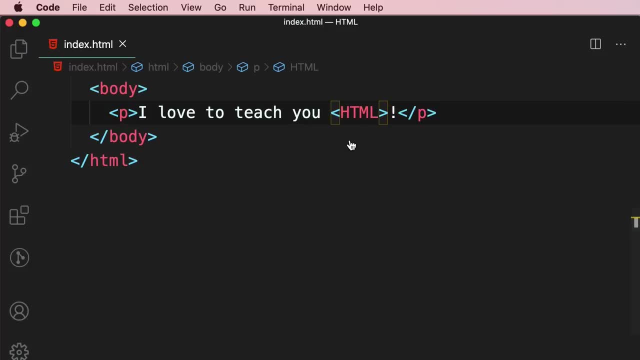 We don't want this, so let's delete it. now back in the browser. look where's our html word. It's not here, because the browser interpreted this as an html tag. This is not what we want. we want to display this exactly as is. 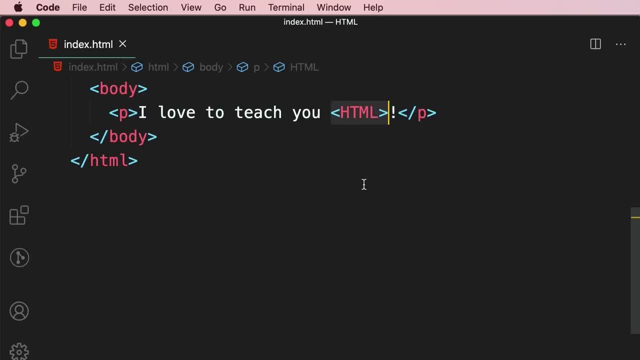 So to solve this problem, we're going to use html entities. All these entities start with an ampersand and end with a semicolon. In between these two characters, we type a few characters that determine the type of the html entity. So we have an entity. 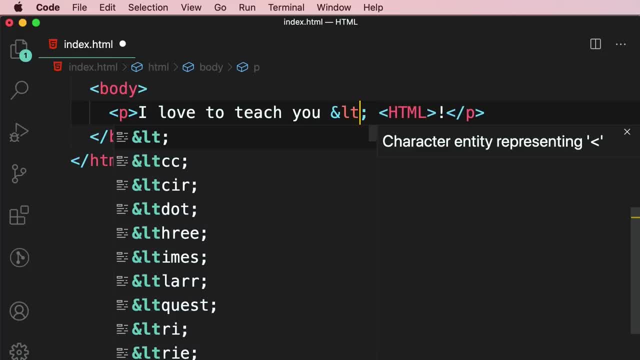 for displaying the less than sign. that is lt, short for less than. Now. let's remove this. similarly, we have another html entity for displaying the greater than sign, So we type an ampersand: gt, which is short for greater than. 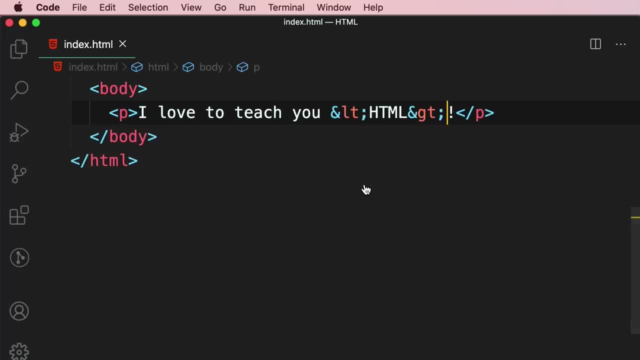 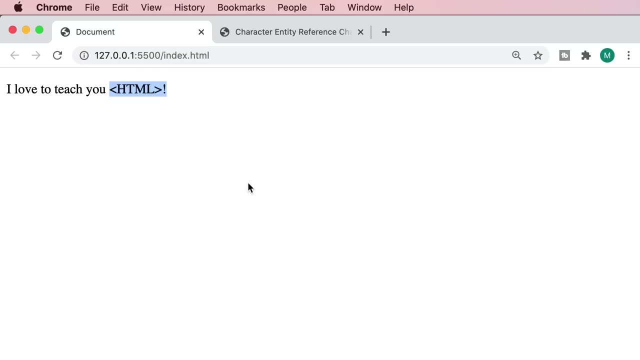 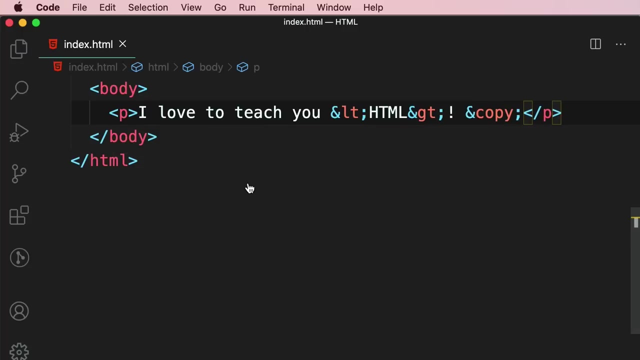 followed by a semicolon. Now back to the browser. that's exactly what we wanted, Perfect. Another common html entity is the copyright symbol, So at the end I'm going to type an ampersand copy and a semicolon. Now take a look. 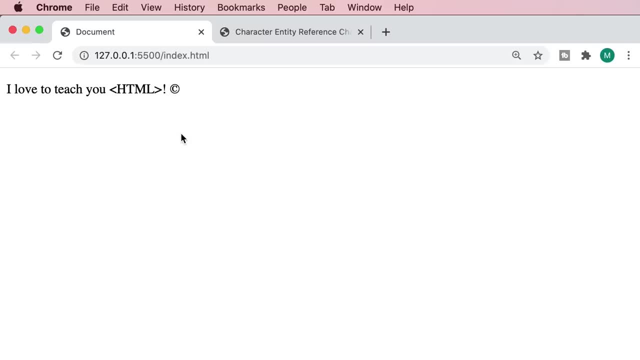 Here's our copyright symbol: beautiful. Now, we have so many entities in html and, quite frankly, you don't need to memorize any of them. In fact, you're not going to use 99% of them, but in case you're curious. 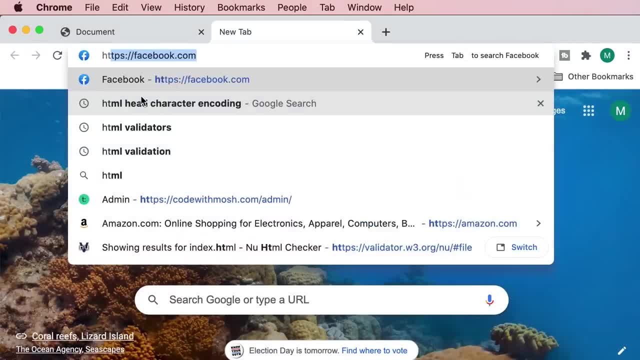 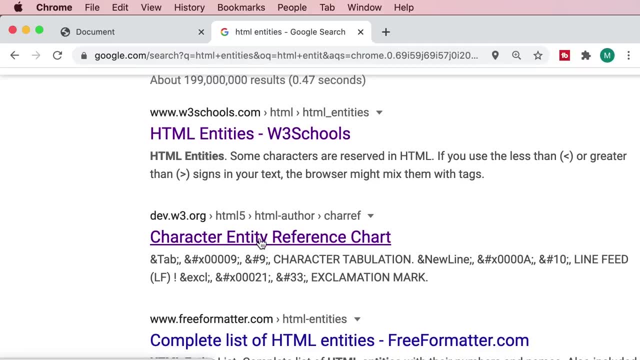 let me show you the complete list. So, on google search for html entities and on this second link, devw3.org, you can see the complete list of these entities. So, as you can see, there are so many entities. 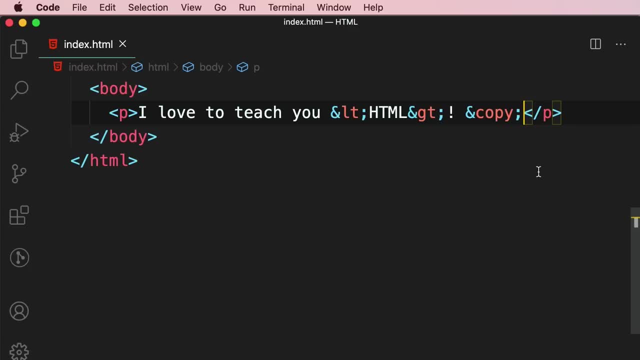 and, honestly, I have never used any of them. The only ones I have used are these three plus non breaking space. Let me show you what that is about. So I'm going to delete this line and generate some dummy text. So we add a paragraph element now to generate: 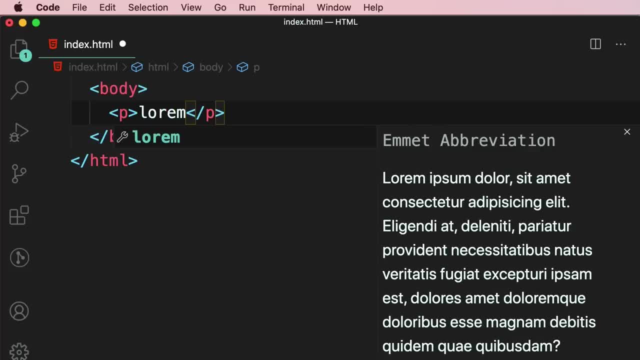 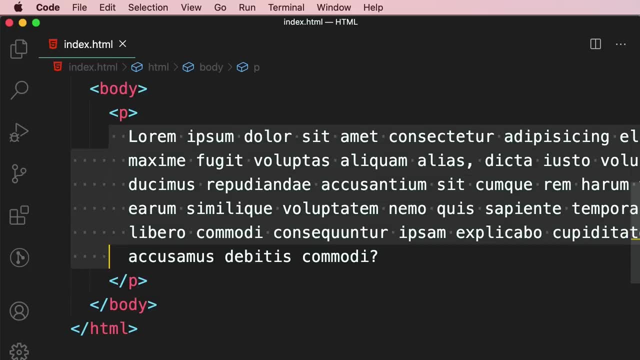 some dummy text. we type lorem, followed by the number of words we want to generate, Let's say 50. Tab. look, this is some dummy text in latin. Now let's preview it in the browser. so here's what we get. let's imagine: 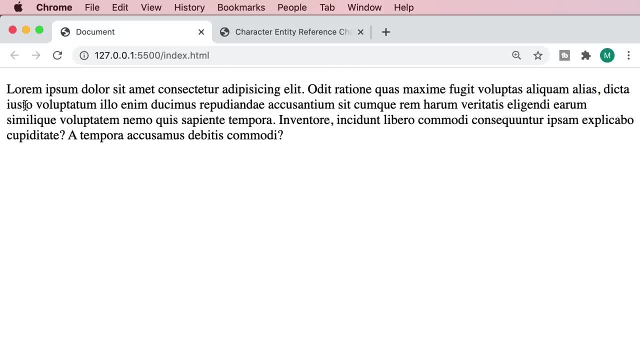 that the last word on the first line and the first word on the second line should be: stick together. Here we have a line break in between these two words. We want to prevent that, So I'm going to copy this word now. 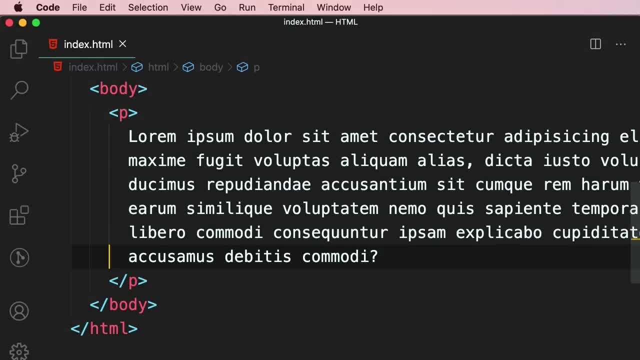 here in vs code. let's bring up the search panel by pressing command and f on mac, or control and f on windows. Now we paste this word. okay, here it is. we want to make sure that these two words are always together. there is no line breaking between them. 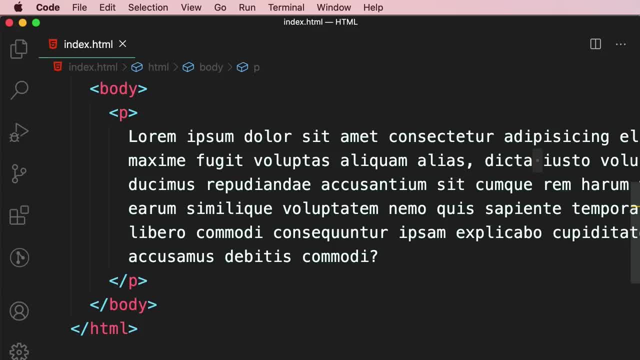 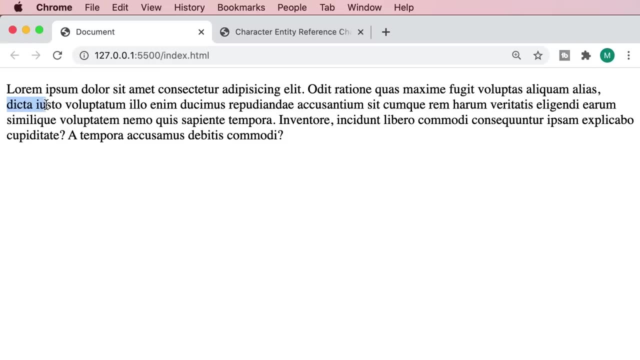 So I'm going to replace this regular space with a non breaking space, which is an html entity. So we type an ampersand- nbsp, which is short for non breaking space, followed by a semicolon. Now take a look. So both these words. 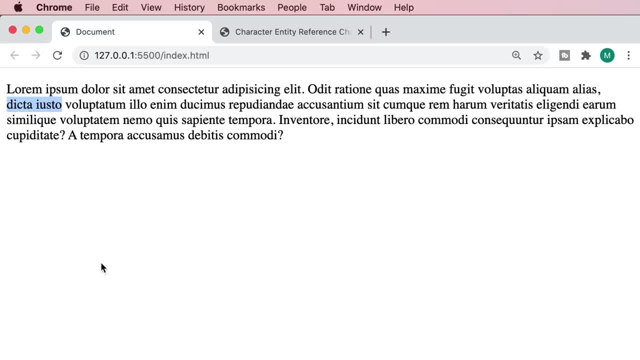 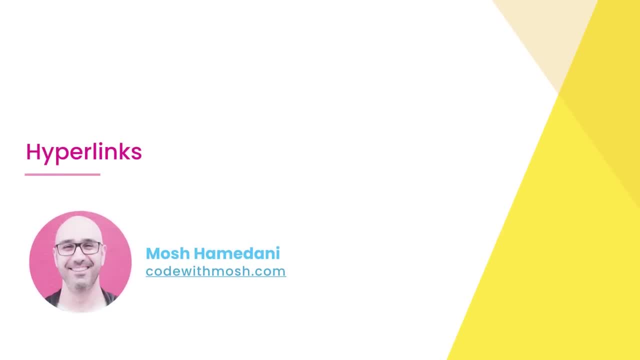 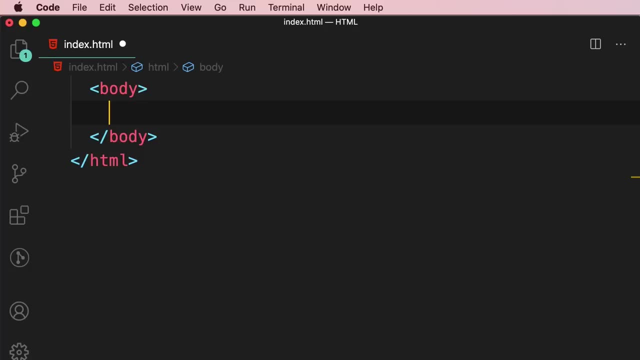 are in the second line. So this is all about html entities. next, we're going to talk about links. Almost every web page on the internet has links to other pages or websites. To create these links, we use the anchor element, So we type: 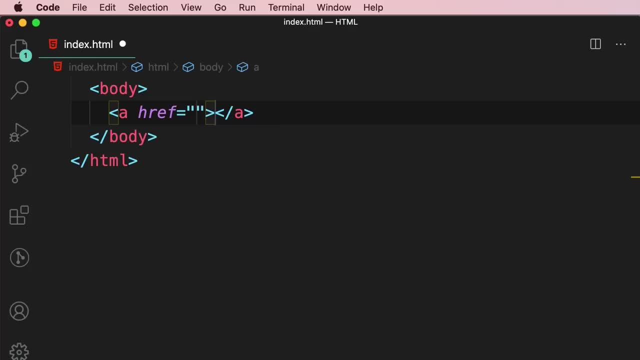 a- that is short for anchor, and then press tab. Now every anchor element should have an href attribute. Href is short for hypertext reference. I know it's a mouthful. it basically means a url or a link. So for this demo, I'm going to create a second page. 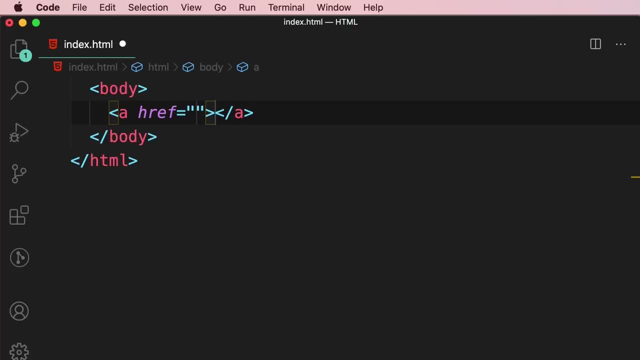 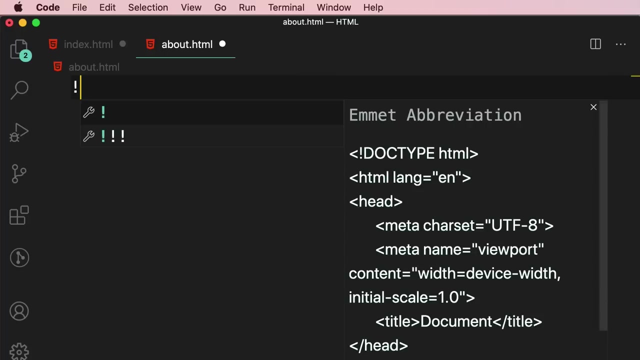 called abouthtml and then link to it over here. So here in the explorer panel, let's add a new page called abouthtml. Now, here we're going to create a basic html boilerplate. Remember how to do that? We type an exclamation mark and then press tab. That's it beautiful. 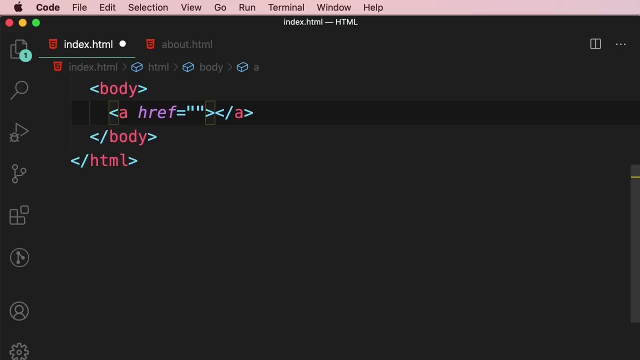 Now back to indexhtml. here we can use a relative or an absolute url. What do you mean by that? Well, a relative url starts from the current page. So currently we are on indexhtml and we want to go to abouthtml. 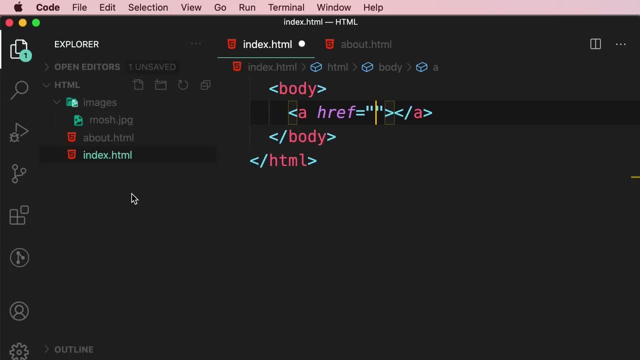 Now, currently both these pages are in the same folder, so we can type a relative url and we want to go to abouthtml, to abouthtml, like this: abouthtml. That's a relative url. Now what if abouthtml was in a different? 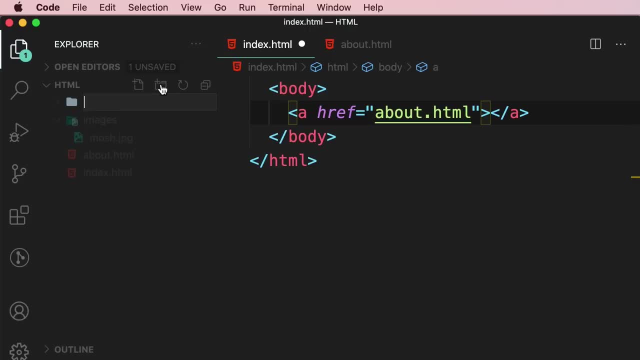 folder. So let's add a new folder to our project called company and then move about to this folder. Now, where is abouthtml relative to the current page? It's inside the company folder, right? So here we type: company slash abouthtml. 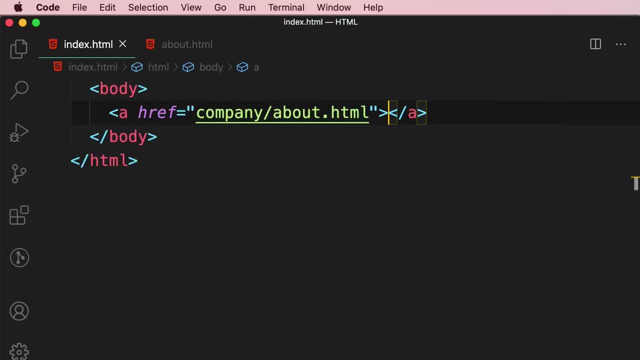 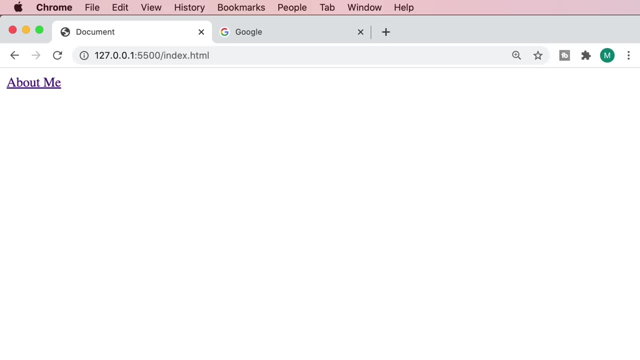 This is a relative url. Now let's give this link a text I'm going to say about me. So we type our text inside the anchor element. Okay, Save the changes back to the browser. here's our link: click and we're currently on the about page, which is: 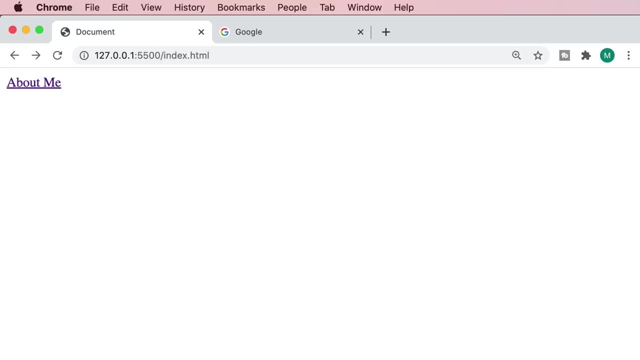 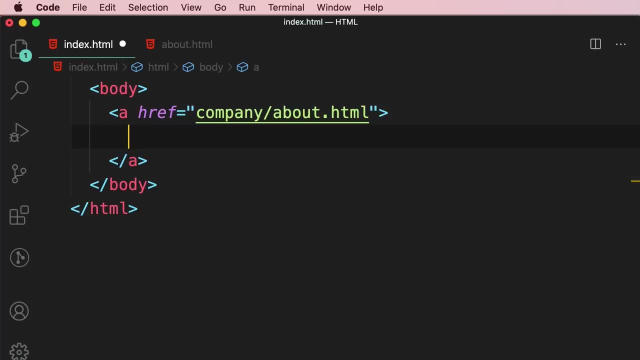 empty, beautiful. Now back to our home page. instead of a text, we can also use an image. So I'm going to delete about me and add an image element. So img tab. once again, here we can type a relative url to our target image. 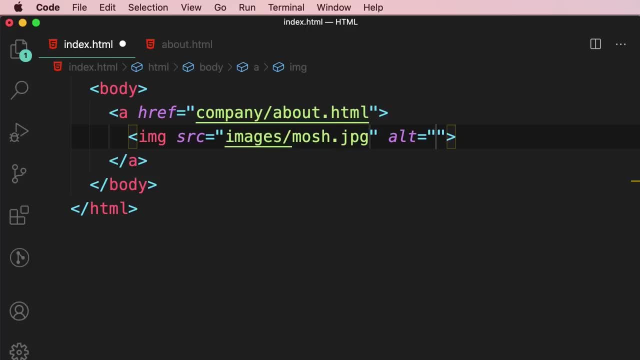 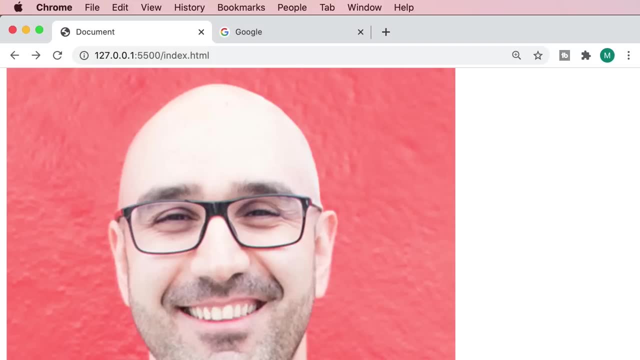 So I'm going to go with images: slash, moshjpg. Now save. take a look. Obviously, this image is way too big. we can always use CSS to resize it. but that aside, look at the mouse icon when we hover over this image. 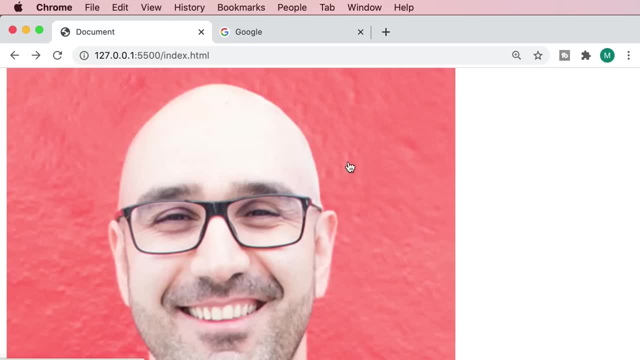 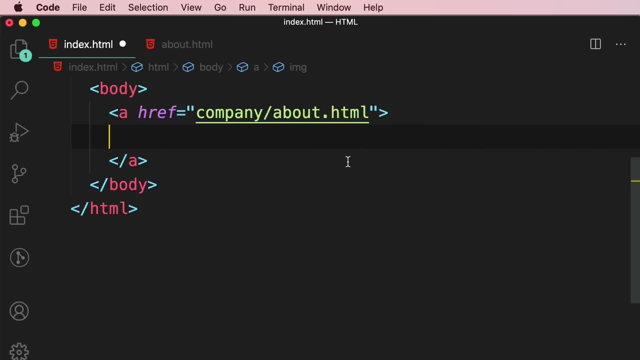 It changed to a hand to indicate that this image is clickable. Okay, Now back to our code. to keep things simple, I'm going to get rid of this image and get back to our text About me. Now let's go to the about page and add a link back to the. 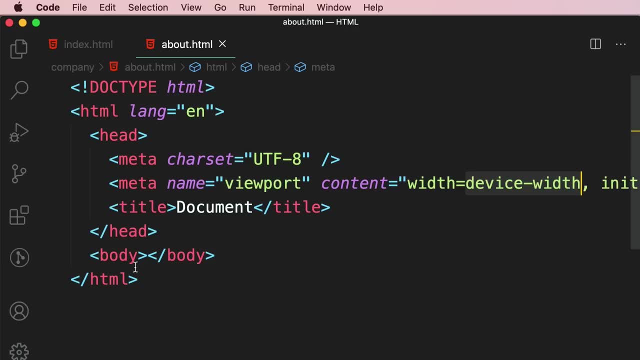 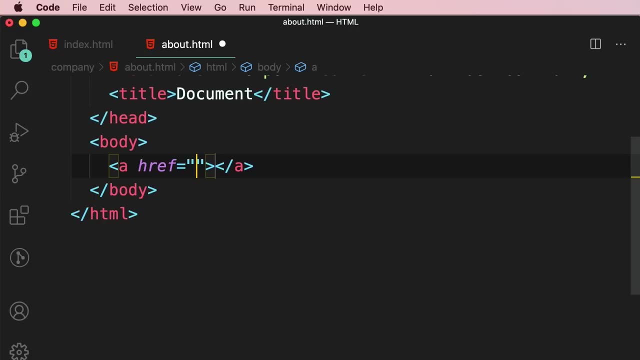 homepage. So over here we're going to add an anchor element. What should we type for the href attribute? Well, currently we are inside the company folder. We have to go one level up so we can access indexhtml right. To do that, we type double period and a forward slash. 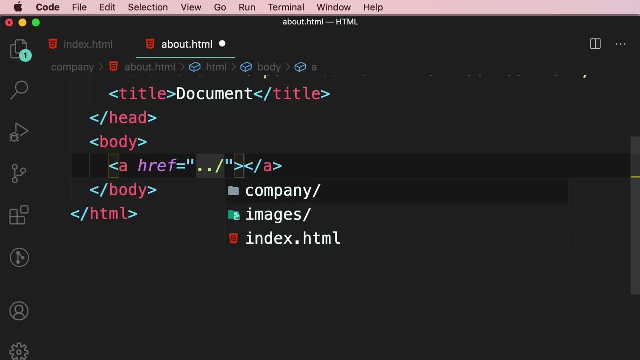 With this we can go one level up, level up. Now, at this level, which is the root of our website, we have the company folder, the images folder and indexhtml. So we can reference indexhtml and for the text we're going to say: 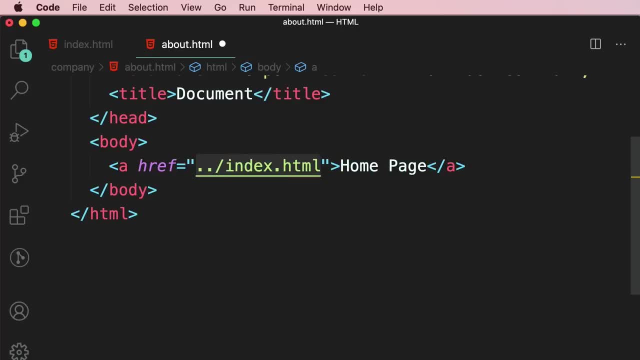 homepage. Again, this is another example of a relative url, because it starts from the current page and goes somewhere else. Now if you're inside a deeply nested folder structure, you might have to go multiple levels up. So double period and a forward slash. 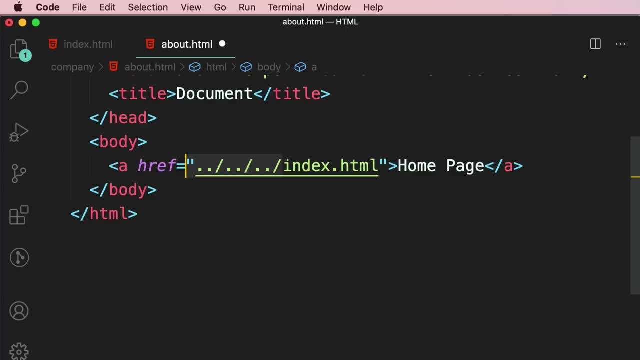 then we repeat and repeat. with this. we can go three levels up. Now, as you can see, urls like this kind of look messy. they look hard to read. In those cases, we can use an absolute url. So we start with a forward slash and this represents: 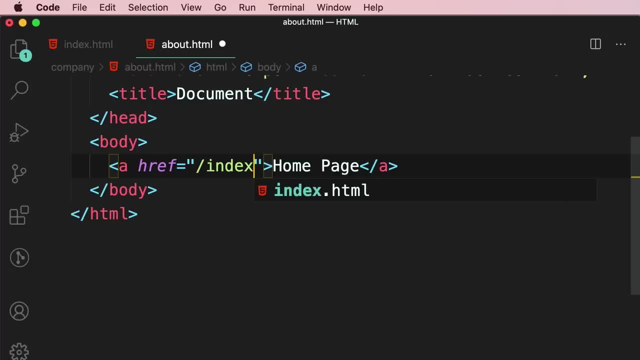 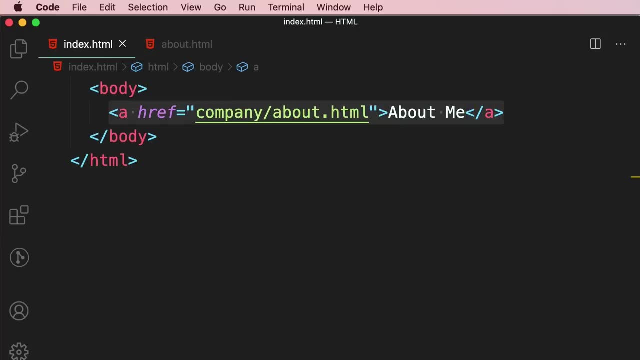 the root of our website. Now, at this level, we have access to indexhtml, So this is an absolute url. Now back to indexhtml. here we are linking to an html document, But we can also link to an indexhtml to non-html documents like images, pdfs, powerpoints. 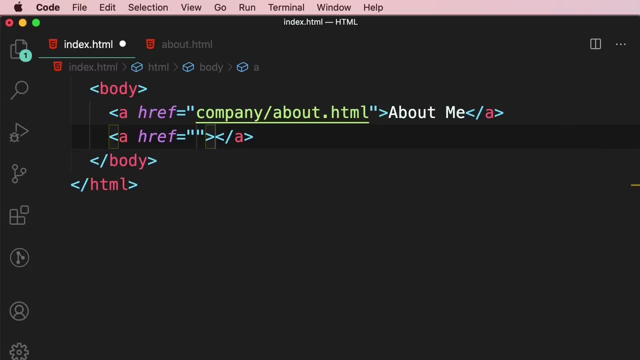 and so on. So let's add a link to my image. so for the href, I'm going to say images slash, moshjpg. and for the text, I'm going to say my photo Save, take a look. So here's our second link. 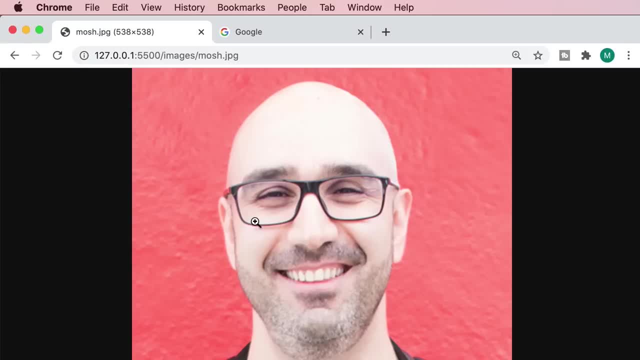 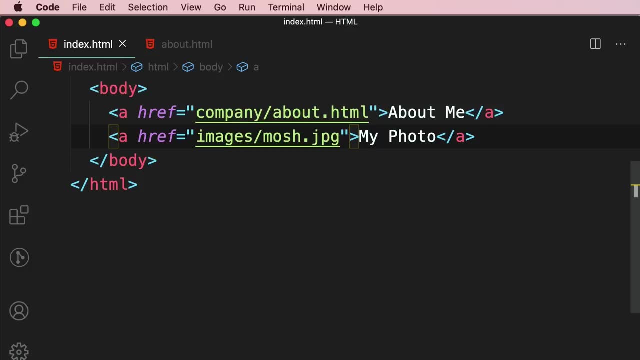 click, my image is displayed in the browser. But what if I want to prompt the user to download it? That's very easy. We're going to add the download attribute to our anchor element. So we type download, press enter. now this attribute doesn't have a value. 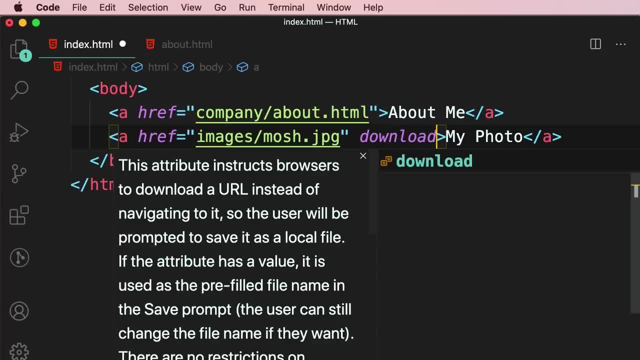 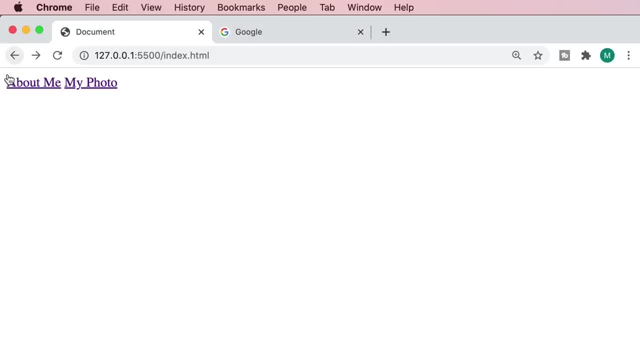 so we can remove the double quotes and the equal sign. So we just add the attribute name Now save back to the browser. we go back here. we have to manually refresh the page because the live server only refreshes the current page Now. previously. 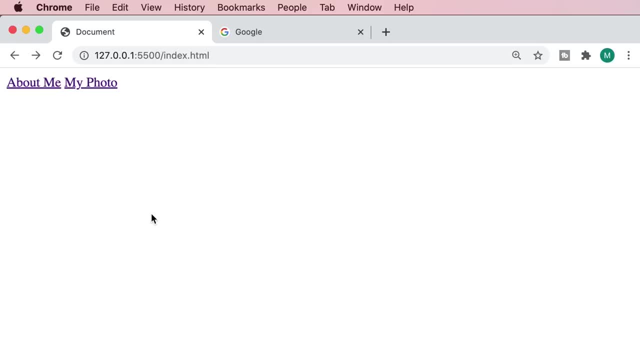 we were on my image, so that was the url. that live server refreshed, So here we refresh to get the latest changes. now, when I click on this link, instead of seeing my image, we're going to see my image getting downloaded. Take a look, click and here's my image, beautiful. 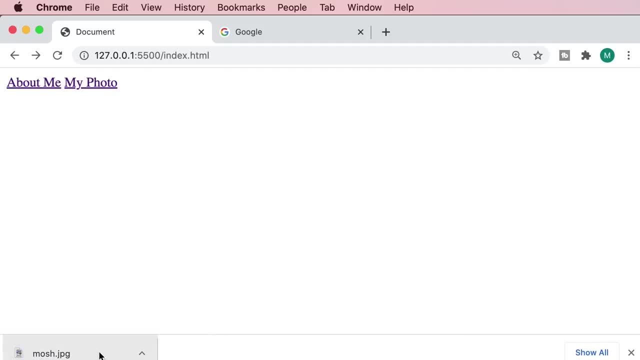 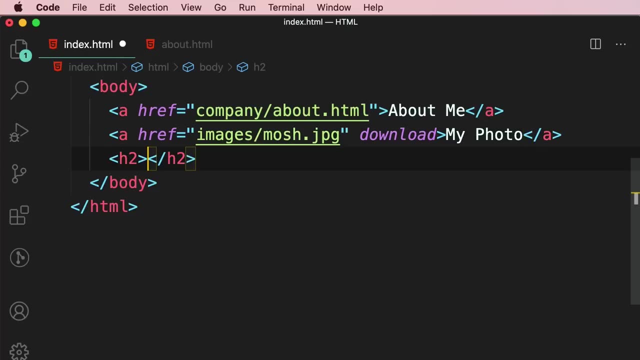 Now we can also link to other parts of this page, so let's create two sections with a lot of text. so I'm going to add an h2 element and of course, I missed the h1, but let's not worry about it. 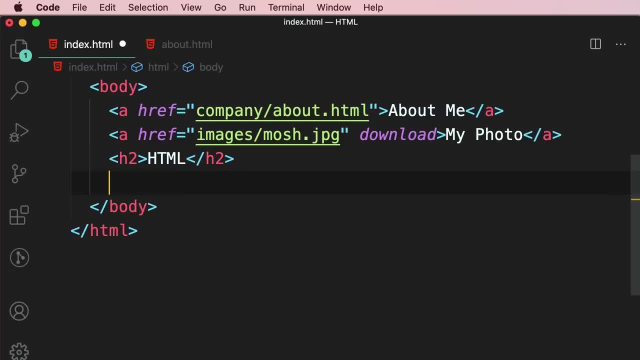 for this h2 we're going to say html, and below that we're going to add some dummy text with 200 words. So paragraph lorem 200, good. Now, right after that, we're going to add another h2 for the css section. 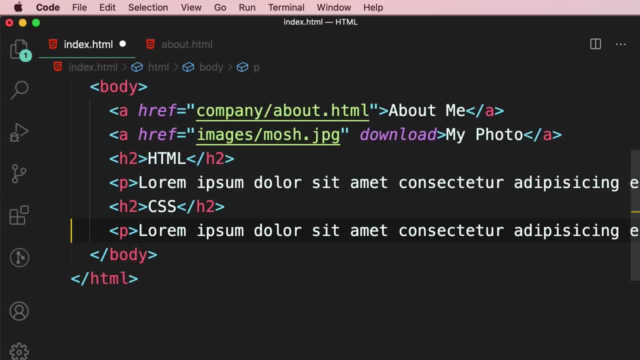 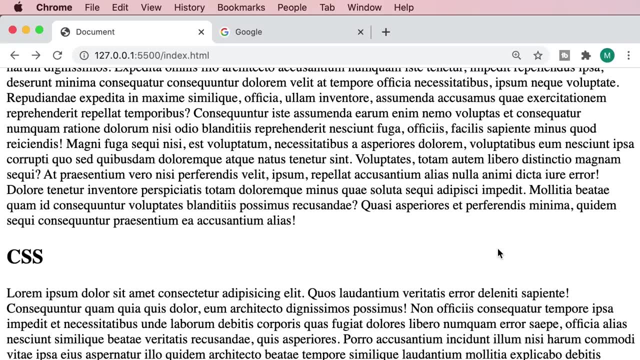 with some more text. Okay, Let's save the changes. take a look: as you can see, the css section is below the fold, so we have to scroll down to see What we can do. here is on the top. we can add a link. 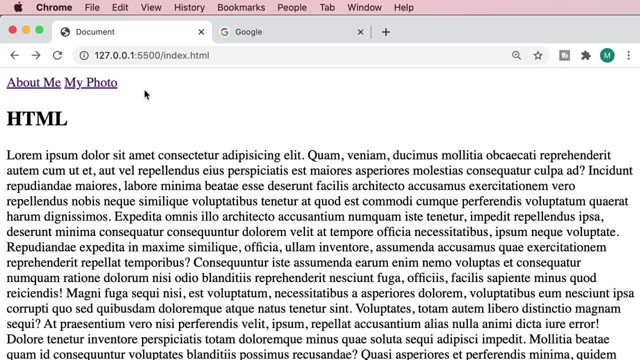 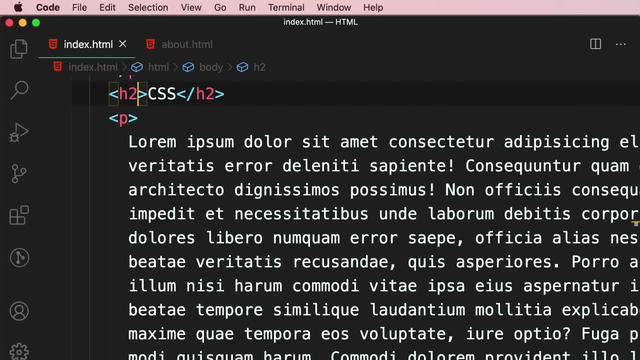 to the css section. so when the user clicks on that they will immediately jump to the css section. that is very easy. So here's the css section. first, we have to give this element a unique identifier, just like everyone in the real world can have a unique identifier like a driver's license or 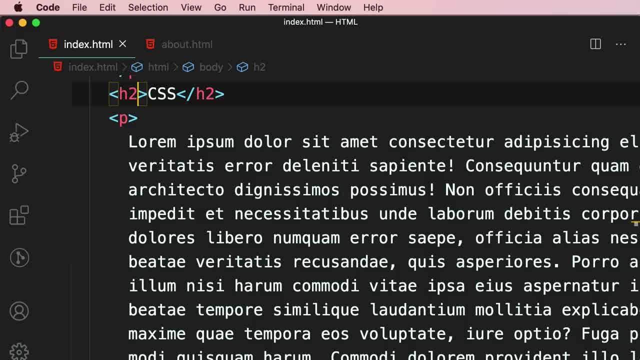 a password. every element on a page can also have a unique identifier. So here I'm going to set the id attribute to css, or we can use a more descriptive name like section dash, css. The name doesn't really matter here. what matters is that we're defining what is called a fragment. 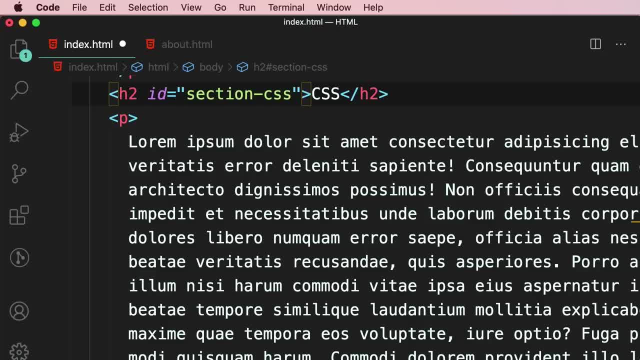 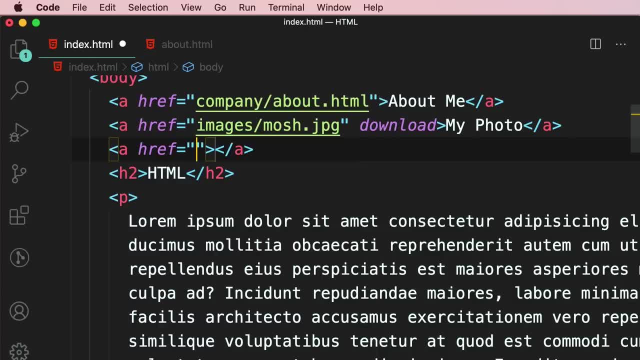 or a place on this page. Now we're going to add a link to this fragment, so on the top let's add another anchor element. now for the href, we're going to type a pound sign followed by the name of our fragment. 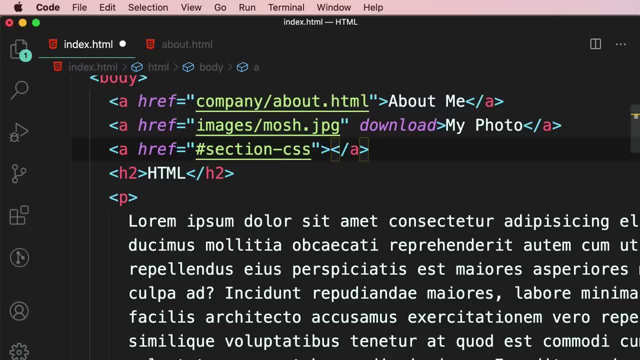 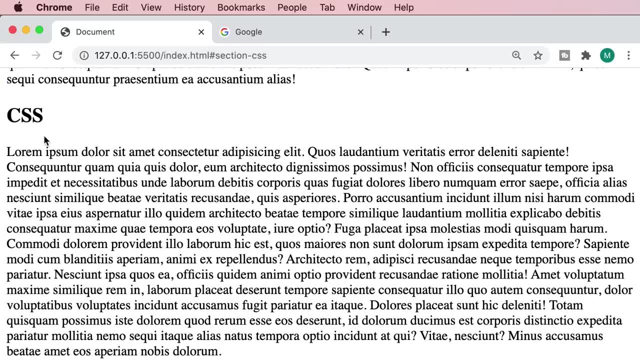 which is section dash- css, and for the text we're going to say css. Now back to the browser. take a look. I'm going to click on this. we immediately jump to the css section. beautiful Now. a lot of websites like this also have a link that helps you jump to the top. 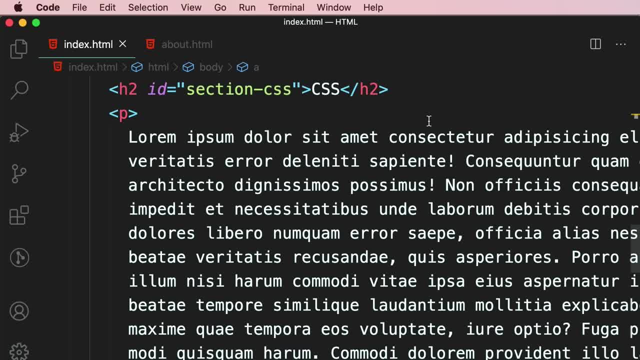 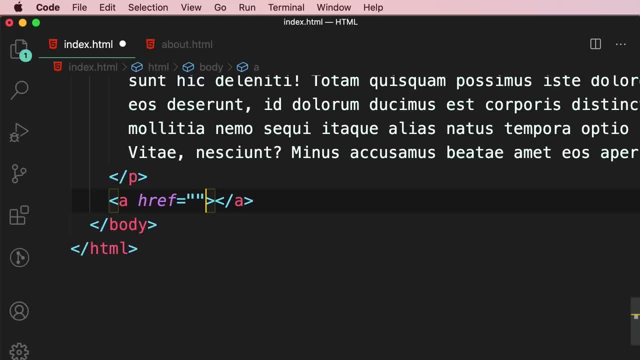 of the page. let's see how we can create that. So after the css section I'm going to add another anchor element. now for the href I'm going to use an empty fragment, so we just type a pound sign without an identifier and then we say jump to top. 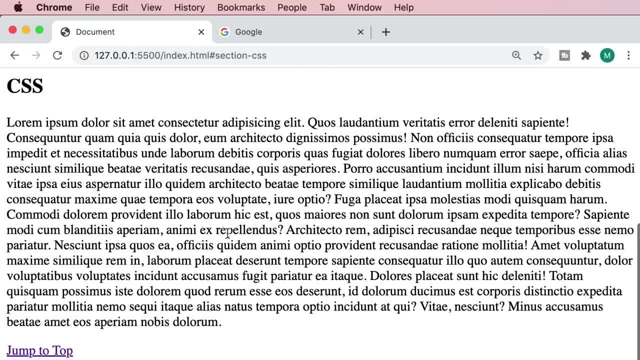 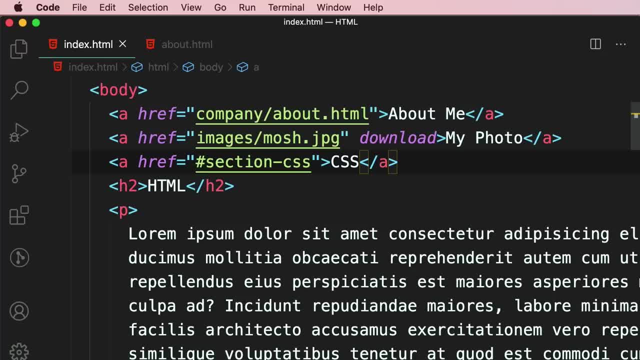 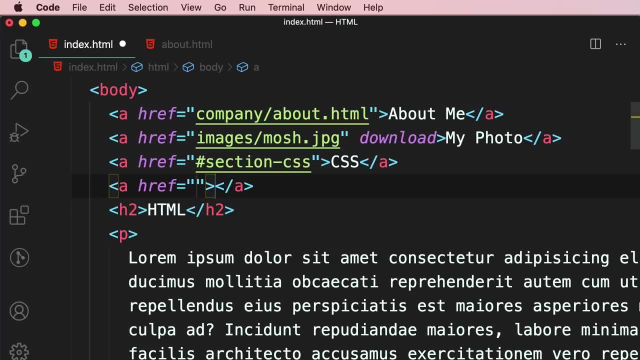 Take a look. So here's our link: click and now we're on top of the page. Now let's see how we can link to external websites. So let's add another anchor element to link to google. Now what should we type here? Well, googlecom is a different website. 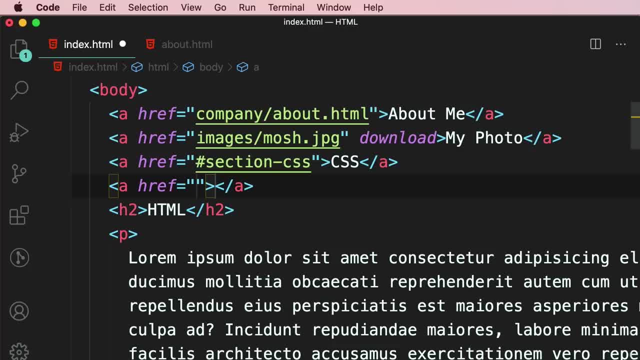 so here we cannot use a relative url. we have to use an absolute url. But if you start with a forward slash, you're referencing the root of our website, But in this case we want to go to a different website. how can we do that? 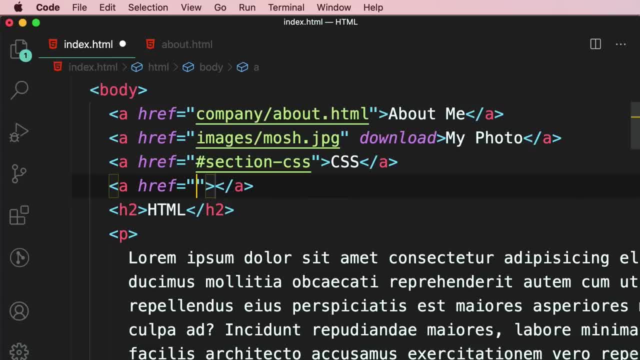 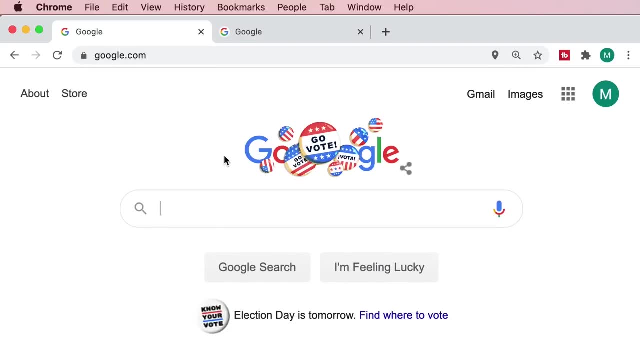 Well, we have to start with a protocol. so https//googlecom. Now let's type google and test our page. click, we're on google, beautiful Now. sometimes, when linking to external websites, we want that link to open. 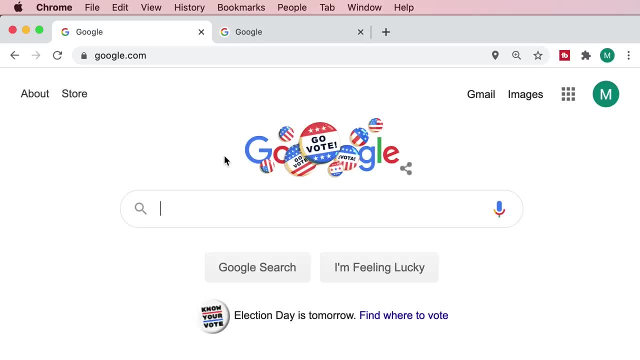 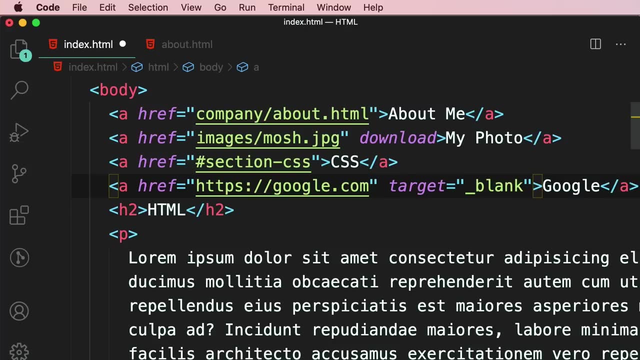 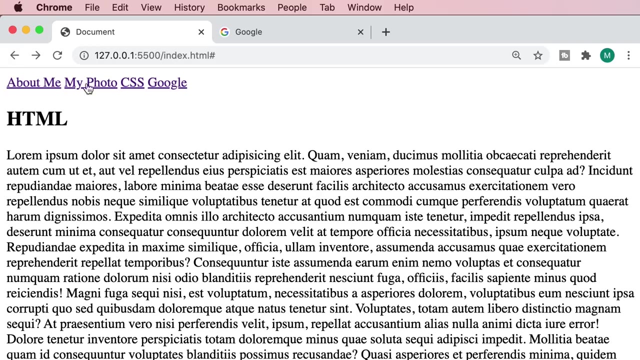 in a new browser window or a new tab. Let me show you how to do that. So here's our anchor: we set the target attribute to underline blank. Now back to the homepage. once again, we have to manually refresh to get the latest changes. Okay now. 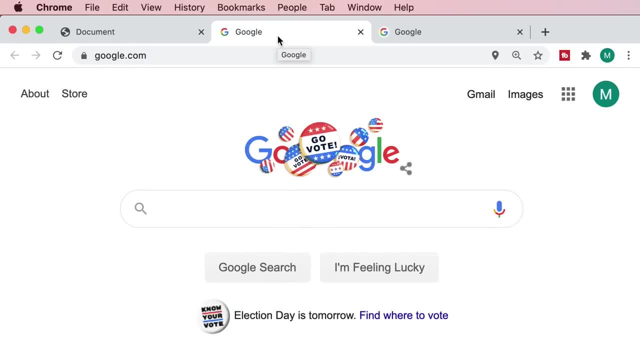 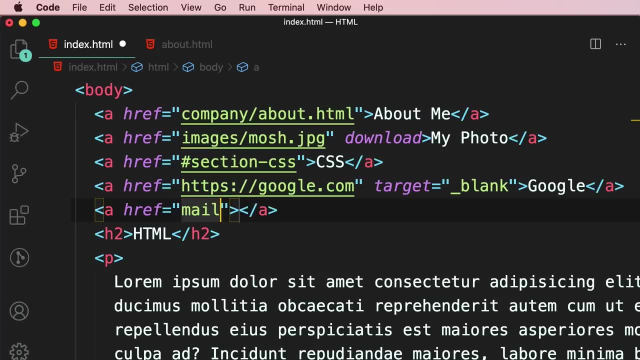 when I click on google, you see a new tab- beautiful. And one last thing: we can also link to emails. so I'm going to add an anchor and for href I'm going to say: mail to colon programming with mosh at gmailcom. 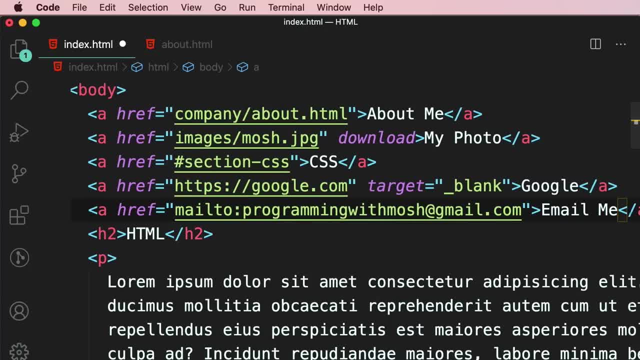 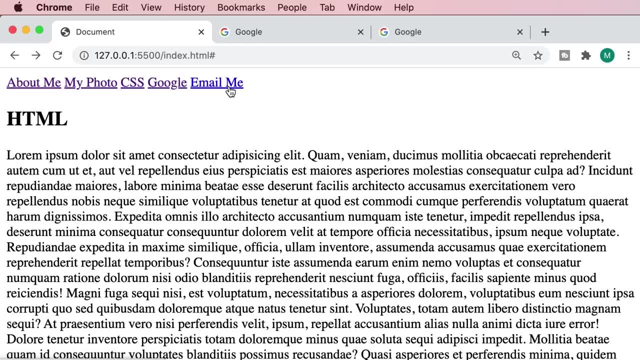 Email me. Save the changes. now back to our page. when I click on this link, my mail client will open and my email address will be pre-populated. Take a look, so click, and here's my mail client. 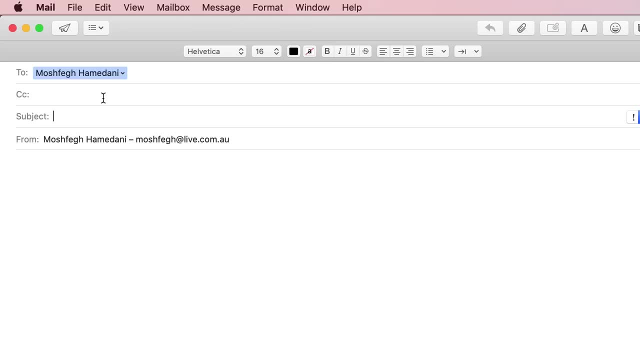 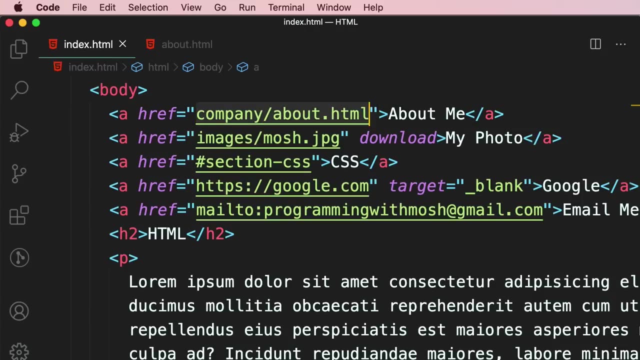 So this is all about links. now one last thing before we finish this lesson: What is the difference between a link and a hyperlink? Well, a link is just an address, a URL, the location of the target page. A hyperlink is the element that. 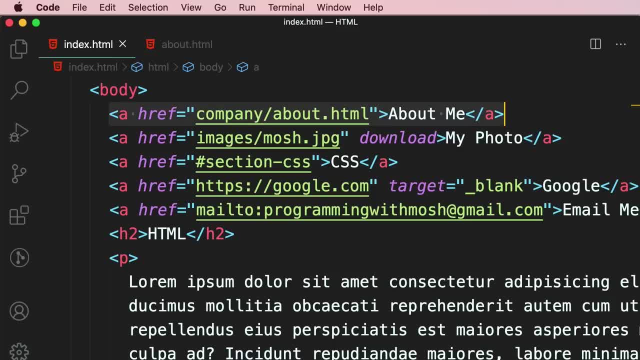 the user can click on to navigate to that target page. That is the difference between a link and a hyperlink, But quite often these terms are used interchangeably. Alright, we're done with this lesson. next we're going to talk about images. 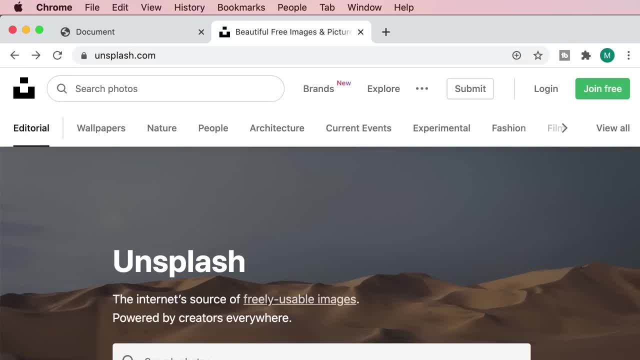 Alright, now let's talk about embedding images in a bit more detail. For this lesson, I'm going to grab an image from unsplashcom, which is where we can find a lot of beautiful and freely usable images. So let's search for coffee. 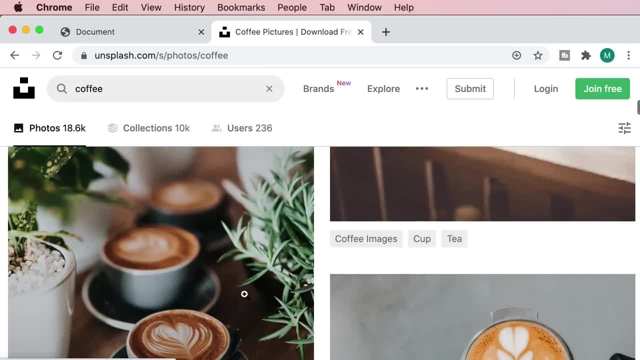 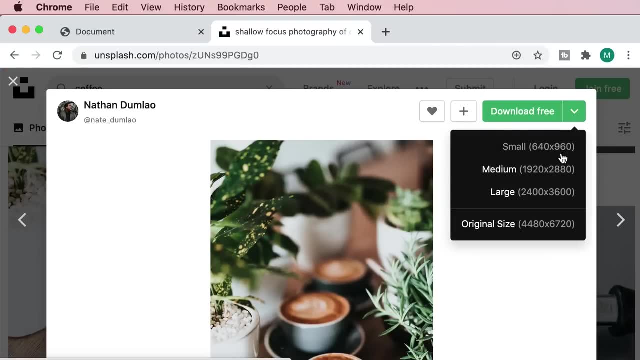 there are tons of coffee pictures here. I'm going to grab this picture. we can download it for free. now look, this image comes in different sizes: small, medium and large. For now we're going to grab this image in a small size, but in the future we're going to talk about 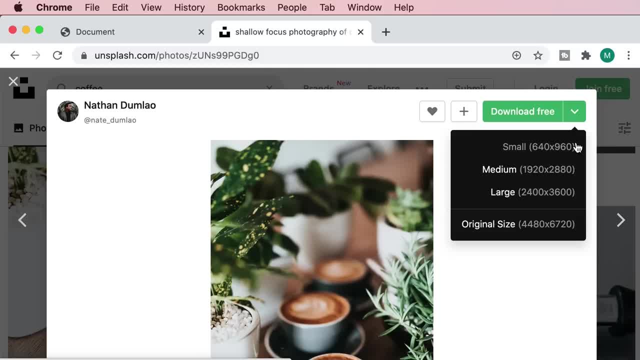 embedding images at different sizes depending on the device. So on mobile devices, you want to serve a smaller image, and on desktop computers, you want to serve a larger image. For now, let's not worry about these complexities. we'll have a complete section on this topic later on. 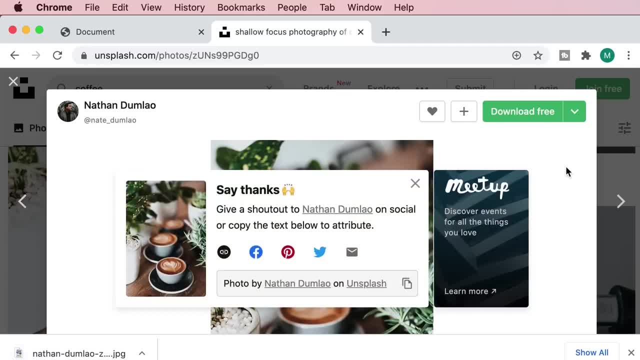 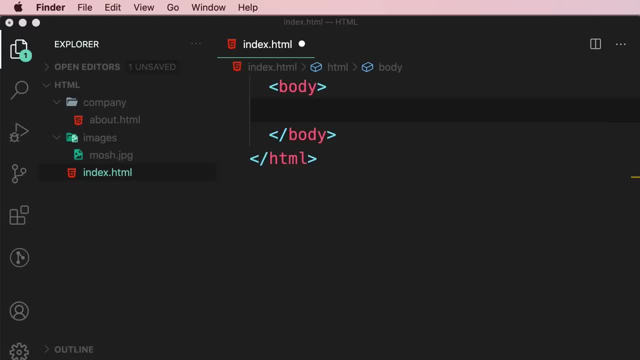 So let's download this small image now. it says: say thank you to Nathan. thanks, Nathan, this is a beautiful picture. you have done a great job. Now I'm going to drag and drop this image onto the images folder and then rename it to coffee. 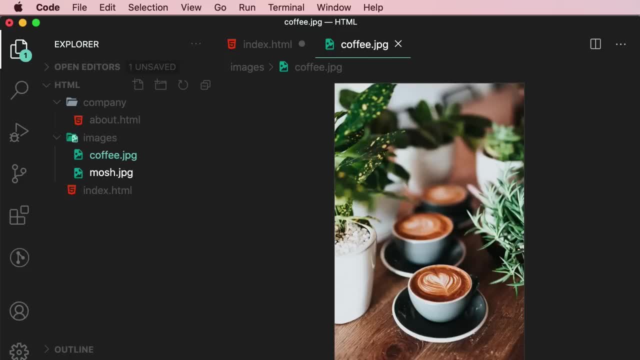 You want to give it a descriptive name. this is a small search engine optimization tip. When we provide descriptive names for our images, search engines can better understand and index our pages. okay, So here's our image. now let's add an image element. 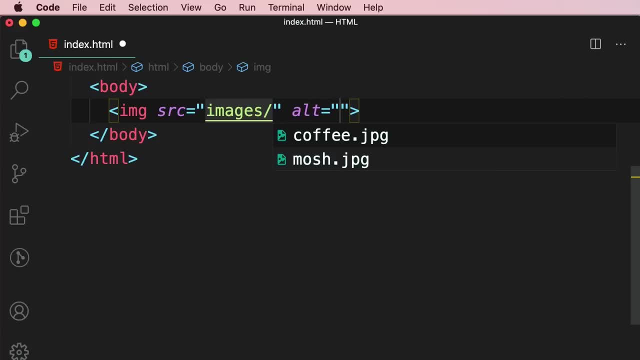 we set the source to images slash coffeejpg. Now, what about the alt attribute? Well, I briefly mentioned that we use this attribute to provide textual description of the image. It's not compulsory, but it's highly recommended for a number of reasons. 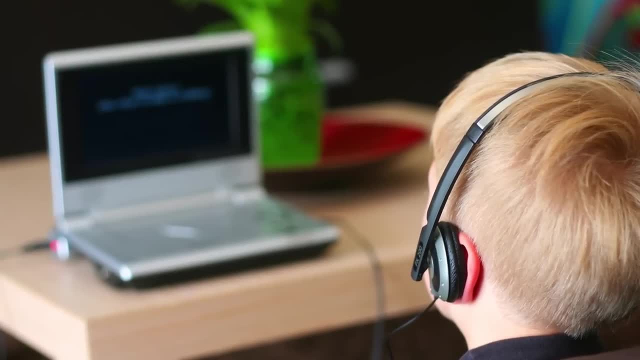 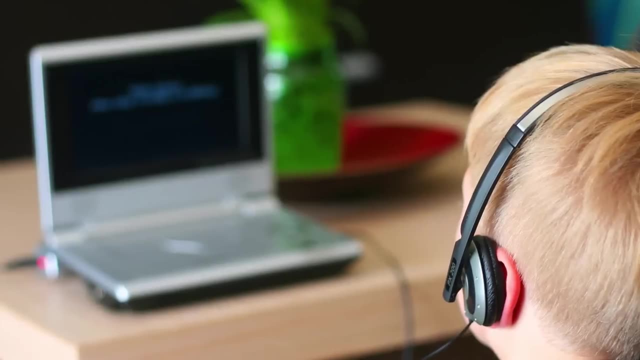 The first reason is to make the image look like a picture, To make our page accessible to visually impaired people. These people use a screen reader to read the web out to them, So with this alternative text, we can tell them what we are showing on the page, And that means we should write. 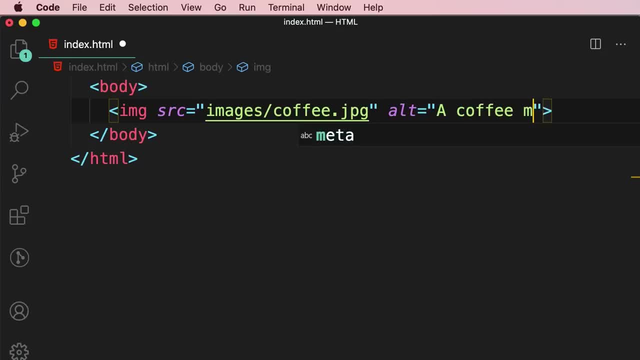 a good, meaningful description here, like a coffee mug on a table. Don't write something like image or image one. that is pointless. Now the second benefit of providing an alternative text is that we help search engines read this text and understand what we are providing here. And there is one more benefit. if this image 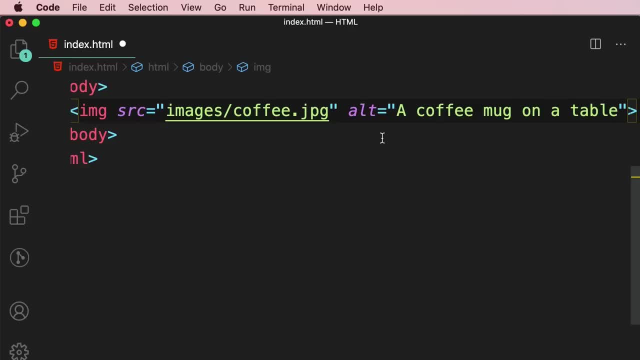 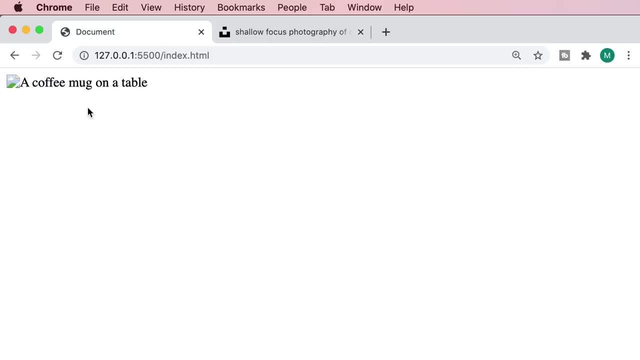 cannot be loaded, for some reason, the alternative text is shown. Let me show you what I mean. So I'm going to add a typo here. now back to the browser. look, the image is not loaded, but we see the alternative text. This can also happen if there is a network connectivity. 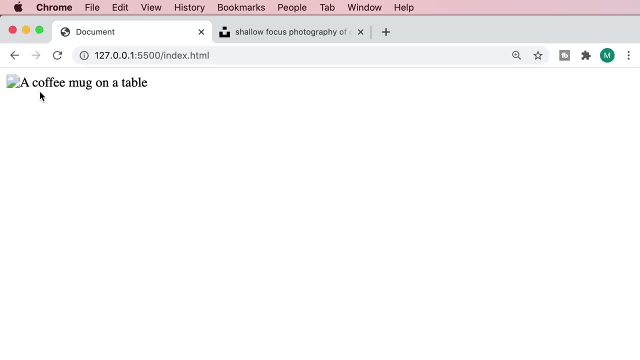 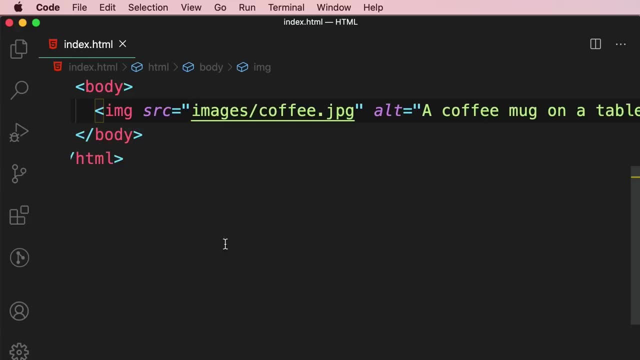 issue. If the user gets disconnected, they can still see the alternative text. So let's remove the typo. now let's talk about sizing images. As I told you before, we can use CSS to resize our images. So here in the head section, let's add: 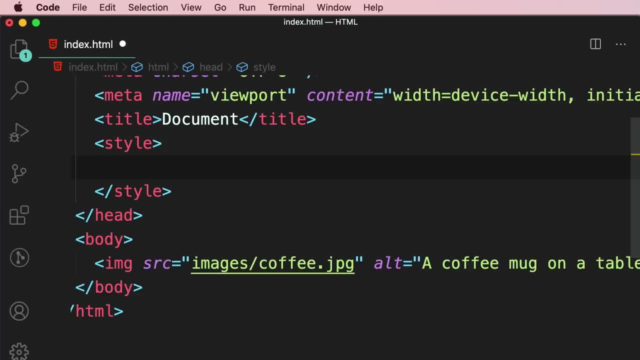 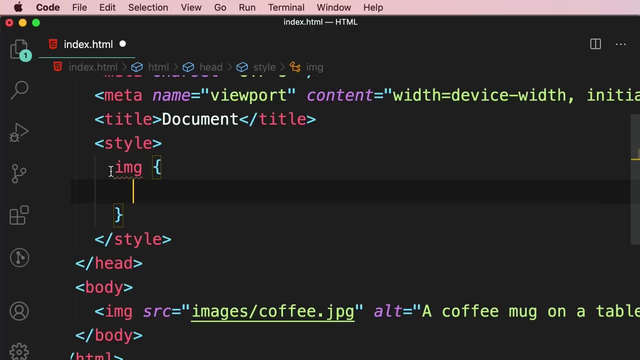 a style element and apply a rule to our image. Now this rule is applied to all images on the page. this is probably not something we want to do in a real world scenario. In a real world scenario, you want to apply a class to this element and then define rules for that class. 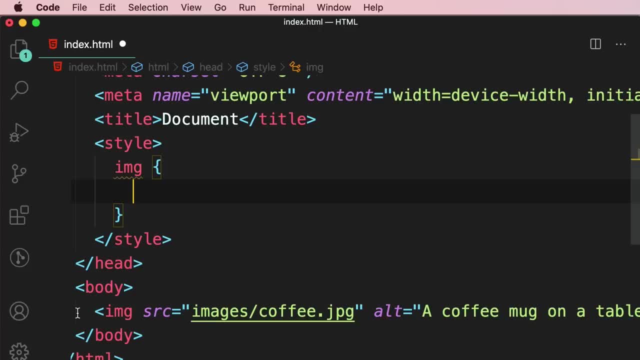 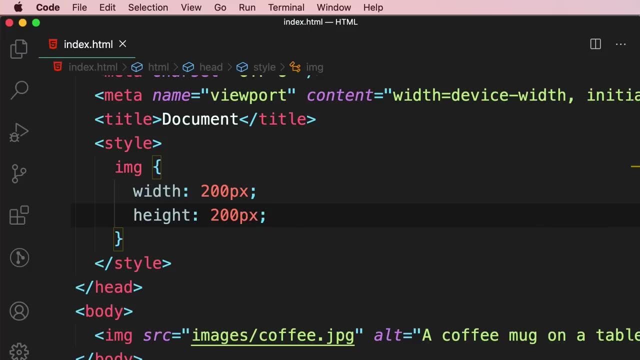 We'll talk about this in more detail in the future. So for now, let's give this image a width of 200px and a height of 200px. Now there's a tiny problem in our image, can you tell? Our image is kind of squashed. 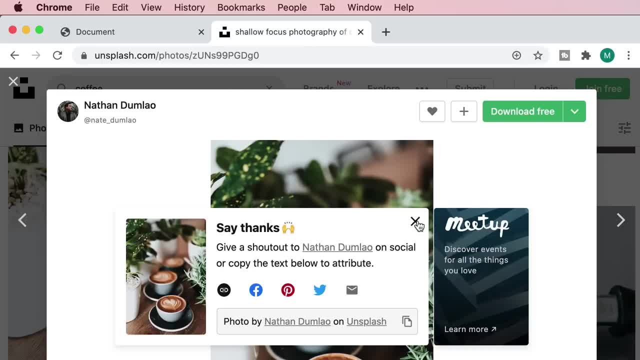 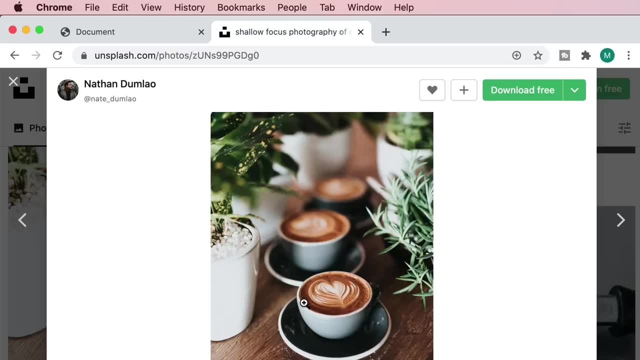 Here's the reason: we're dealing with a rectangular image. look, this is a rectangular image, but we're converting it to a square image. Now look at the shape of this coffee mug. it's kind of round. right Now, compare it with what we have over here. our image is vertically squashed. 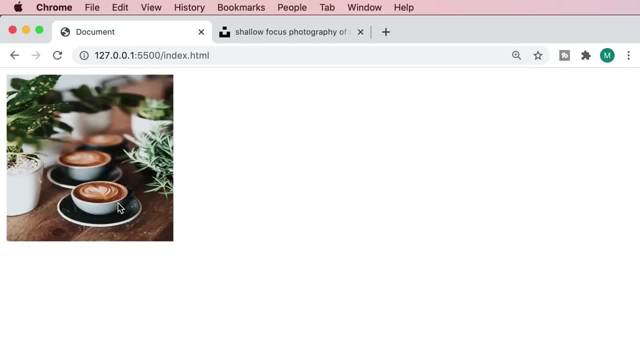 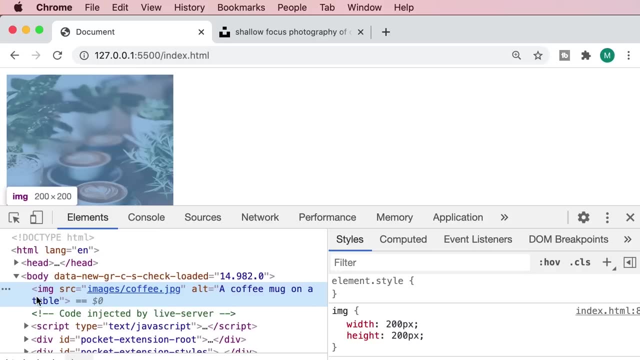 Let me show you how to do this. Let me show you another way to verify this. We can right click on the image and then go to inspect. this opens chrome dev tools and selects our image in the DOM. Now, on the right side, we can see: 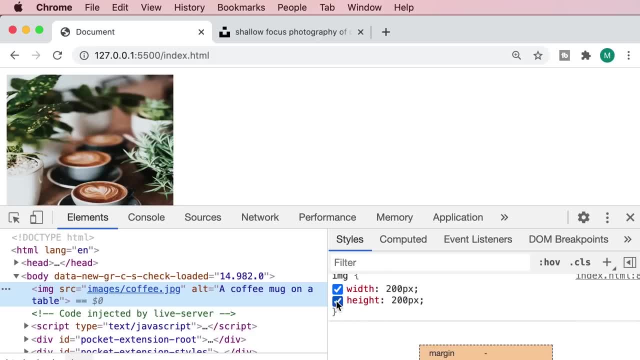 the styles that we applied to this element. Now I'm going to disable the height property and I want you to pay close attention to the image and see how the shape changes. So look, now the coffee mug is more round. but if I apply the height property, 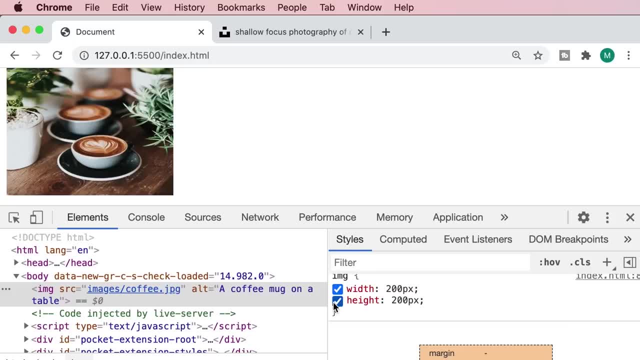 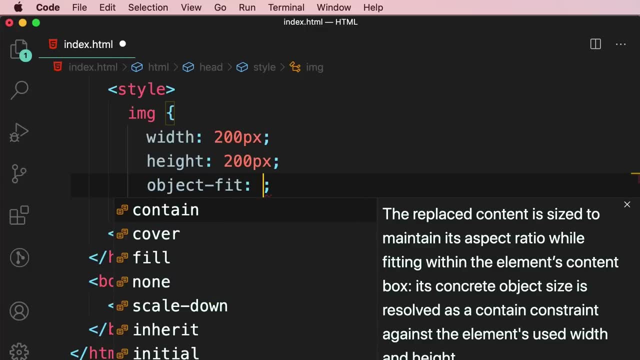 it becomes squashed. So how can we solve this problem? Well, we have a new property in CSS called object fit. So here we can set object fit to one of these values. Most of the time we use cover, so the image covers its containing box. 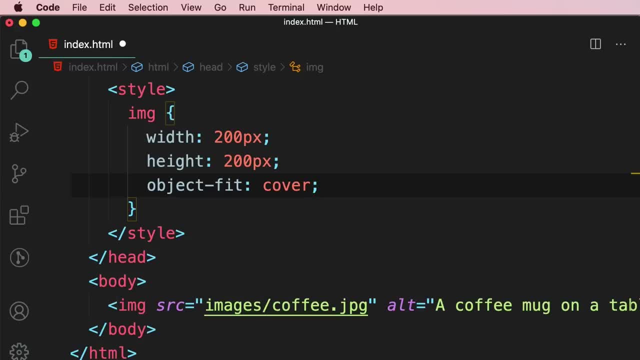 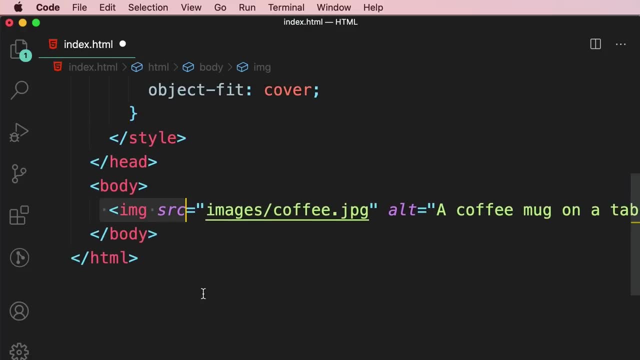 What is this containing box? Well, first let me set this to cover. here we have this image element right, Conceptually, there is a box around every element in an HTML document. We don't see this box, but the browser uses that box to figure out how. 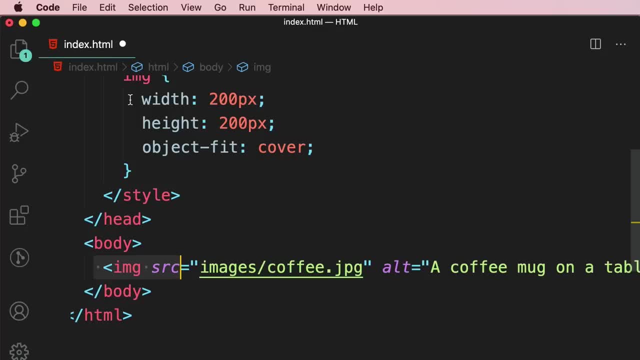 the page should be displayed. So here we have a box with this dimension, 200x200, and in this box we're trying to insert this image right Now. when we set object fit to cover, our image will get resized and potentially cropped so it covers the entire.